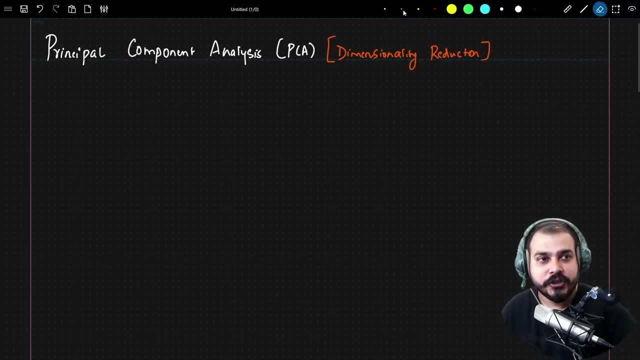 understand why should we use PCA or dimensionality reduction? So for this we really need to understand about a topic which is called as curse of dimensionality. Okay, so curse of dimensionality. and in order to make you understand this specific topic, let me take some examples over here. 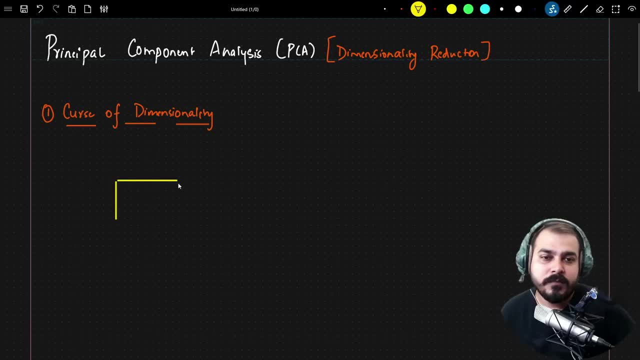 Let's say I have various models. Okay, so let's say, this is my machine learning model M1,, this is my machine learning model M2,, this is my machine learning model M3,, this is my machine learning model M4, and I still have some more machine learning models, So be. 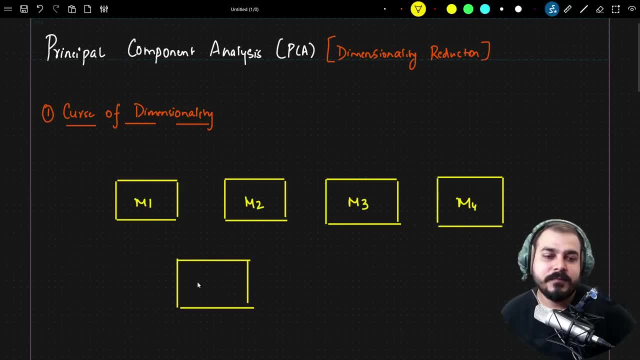 patient. Okay, M5, and this is my machine learning model M6.. Okay, so let's consider, I have this many machine learning models. Now let's say that I have a data set and in this specific data set, I have somewhere around 500 features. 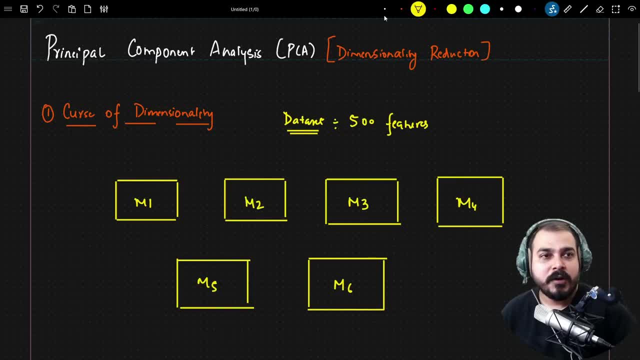 Okay, and whenever we say about dimensionality, this basically means we are talking about something called as dimensions, And whenever I say dimensions, this is nothing, but this is features, Okay. so let's say, this data set that I specifically have is to basically determine, or. 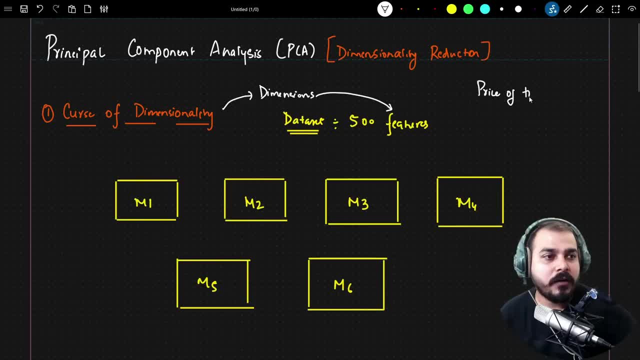 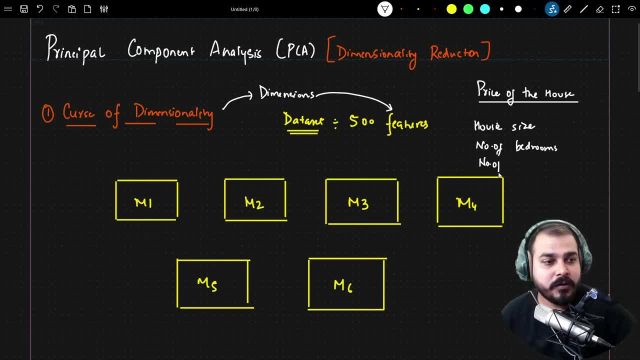 or it maybe, uh, I may also have features like number of bathrooms. Right, I may have this many kind of lot of features. Okay, Now, obviously you know, to basically find out the price of the house, What is the most important thing? 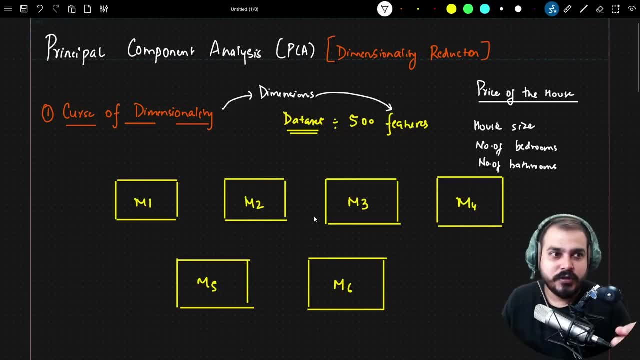 You know, probably you need to know the house size, You need to know the room size, you need to know the number of bedrooms, You need to know many number of washrooms. right, let's say, for the model m1, i have provided around the most. 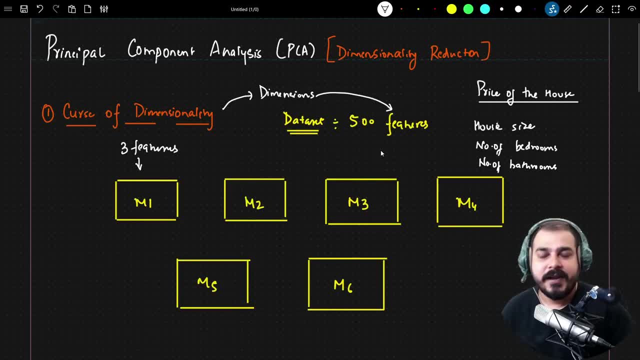 three important features to train out of this entire 500 features. okay, let's say after that, for the m2 model, i provided somewhere around six features for training the model- okay. similarly, for the model 3, i have provided around nine features, let's say for training the model m3. 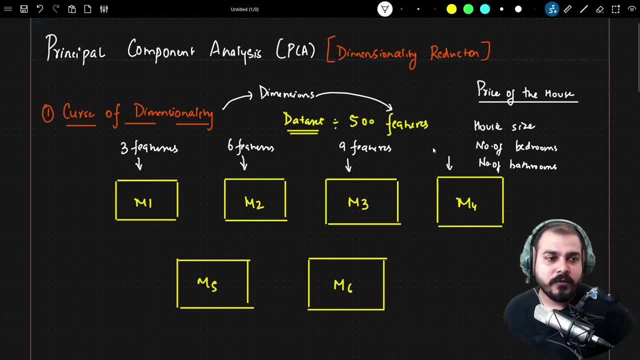 right. and after that, for the m4, let's say i have provided 50 features okay. or let me just not make it as 50 right now. let's say that okay, in this, in this particular case, i have provided probably 15 features okay. so let's say, over here i have provided 15 features and here now i have increased. 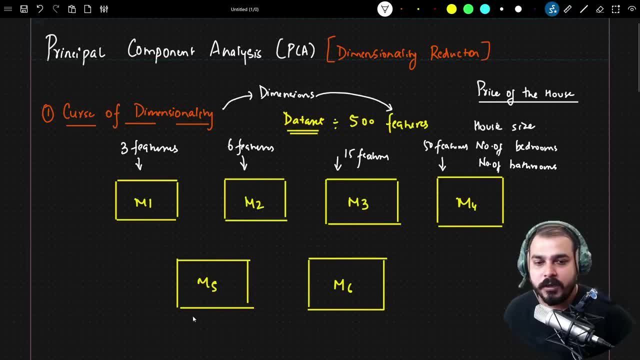 the number of features. here i have provided 50 features for training this particular model, and then probably here i have provided 100 features, and then here i have actually provided 500 complete features. okay, now, what will happen when i'm providing this many number of features for every model? okay? 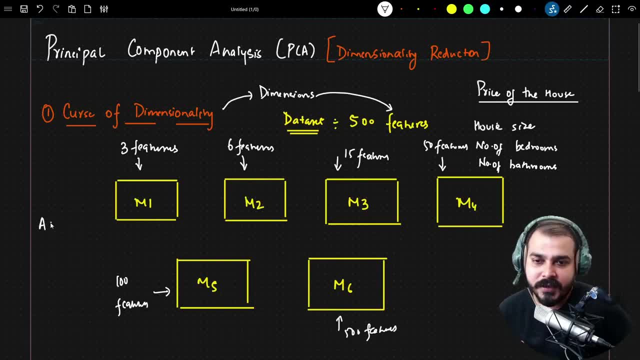 now, let's say, this model m1, uh, i will be getting some accuracy, okay, and uh, this accuracy is based on this three specific features, right? so here let's say this is my accuracy one. so here i am specifically getting accuracy one right now, after i train my model with these three features and probably train this particular model, i'm going 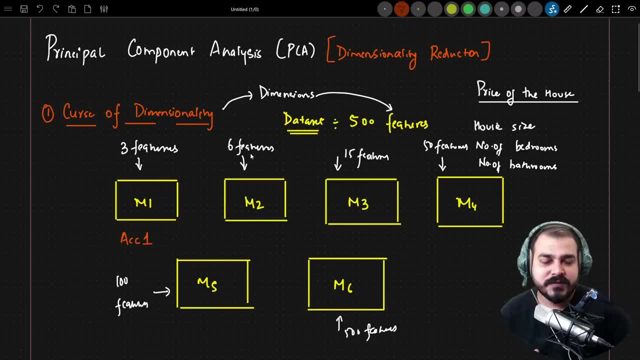 to get accuracy one. now let's go to the next model, where i specifically use six features, and let's consider these six features. all are very, very important for determining the price of the house. then what may happen is that my accuracy two will still increase, right, uh, when compared. 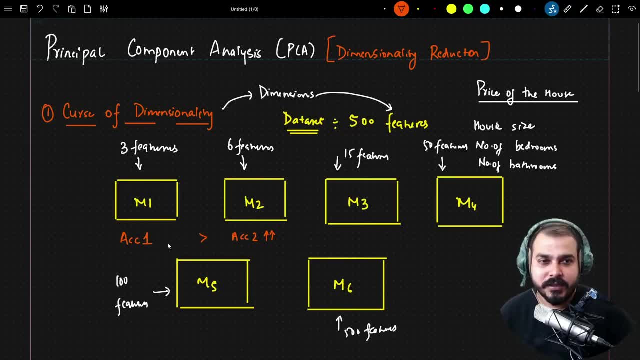 to accuracy one. so here i can definitely say accuracy two will be greater than accuracy one. then let's say m3. uh, again, when which, whichever features we actually provided, like this 15 when compared to the previous six feature. so i may get an accuracy three which may be more good. 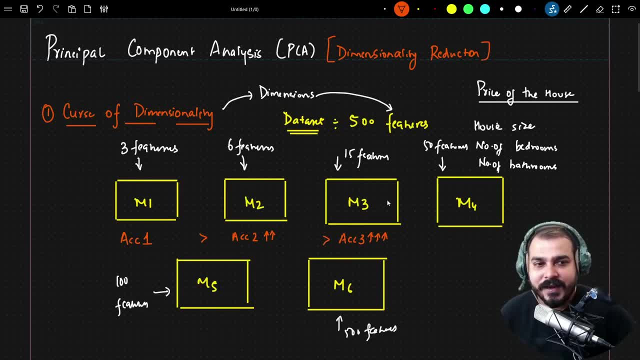 at this point of time- okay now, let's say when i probably went to model four here. now you will be able to see that i'm providing 50 features now. now, in this features there may be a scenario that some of them may not be at all so much important, right, and some may have more importance, some may 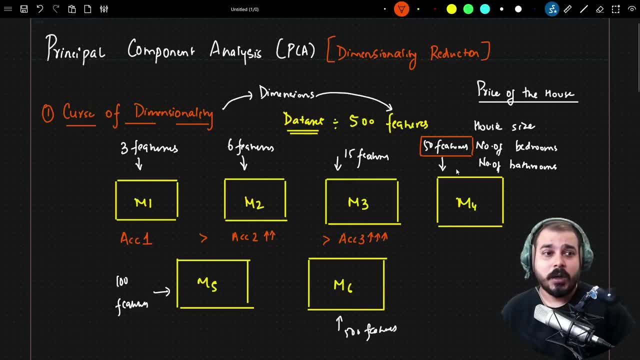 have very less importance. some may have no importance at all. right, so now, when we will try to find out the accuracy here, you'll be able to find out. the accuracy will keep on decreasing when compared to the previous accuracy. now what will happen is that, uh, in this scenario you will be 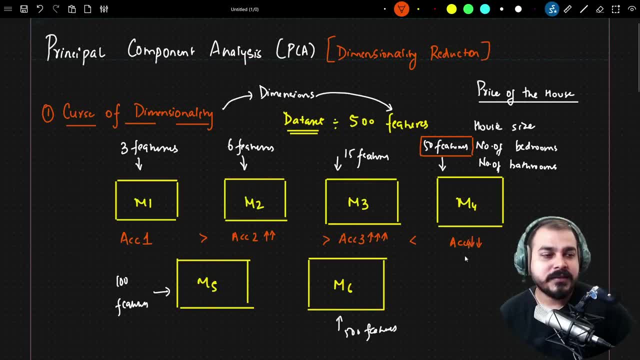 seeing that this accuracy 3 will be greater than this accuracy 4. okay, and i'll explain you why this specific thing will probably happen. so let's say, this is my accuracy 4, and here you can see that the accuracy 4 has decreased when compared to accuracy 3.. then when i go to the next model where i'm 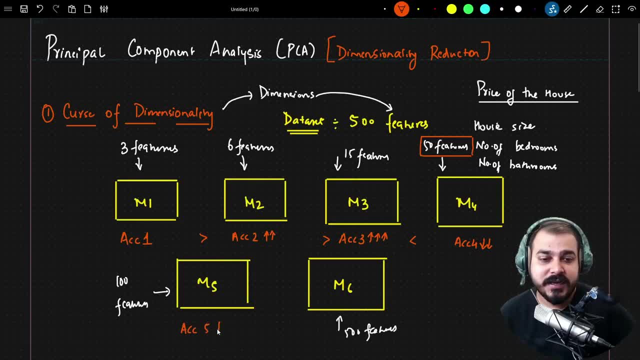 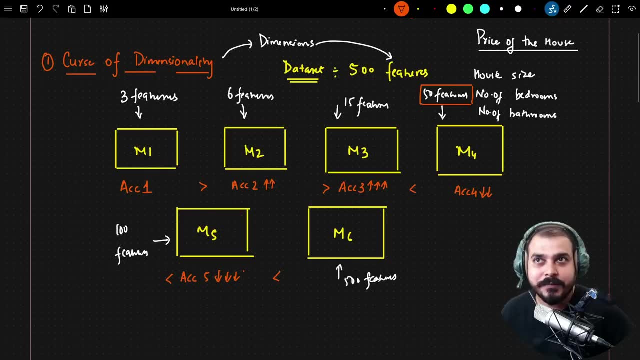 specifically providing 100 features. here the accuracy will still decrease. and then when we go to the next model, where i've specifically provided 500 features- and this may include all the features that i've provided in the data set here- you'll be able to see the accuracy. 6 that you will be. 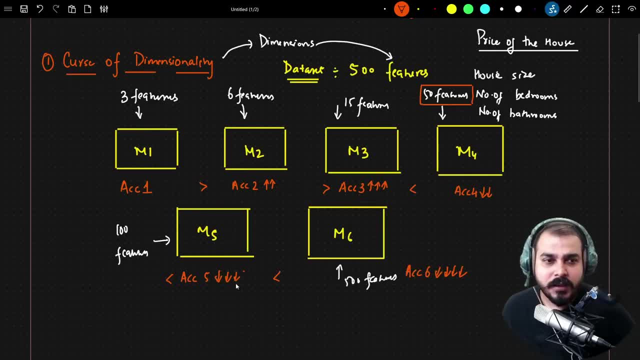 getting will still more decrease when compared to the previous accuracy. now you may be thinking right why this thing is basically happening. this is the reason why we say curse of dimensionality. now just imagine, guys, it's just like over here in model m1, m2 and m3 when we were seeing that after training with, let's say, an m3 model, we were 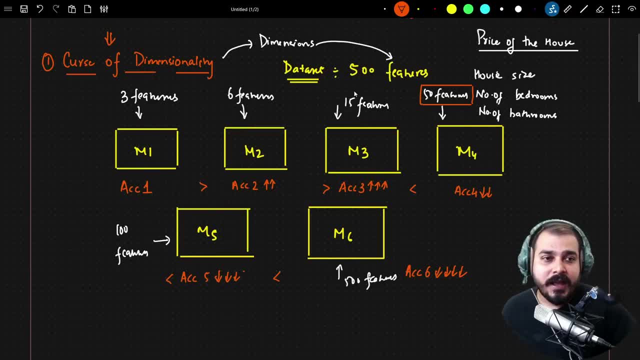 training with 15 features. the accuracy was quite increasing over here and we can consider that this, all features were quite important for this particular model to perform. well, you know. but when we went to accuracy 4 or when we went to probably this model 4, you know, here we have 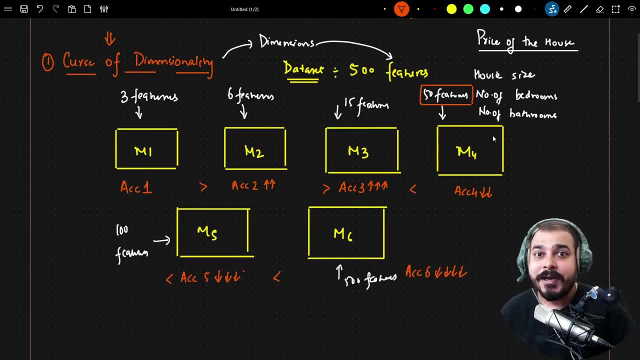 increased the number of features. now this specific model did not require that many number of features to do the prediction over here you can just say that the model is overfitted. right, the model is overfitted, so model should be given that many number of features through which. 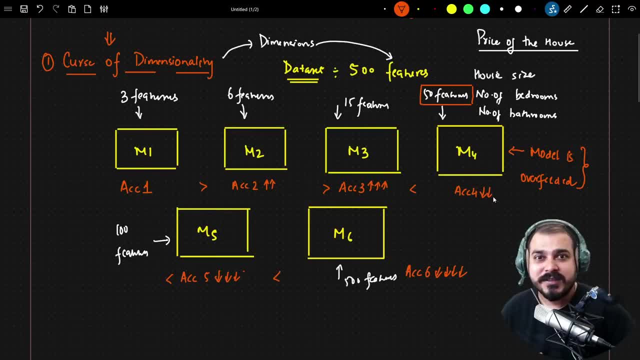 the accuracy should keep on increasing, but here you can see that the accuracy is decreasing. similarly, after this particular step when we go to the next step. you know, here also you could see that as soon as i provided 100 features, and obviously in these features there may be a situation that some of the features may not be at all useful. 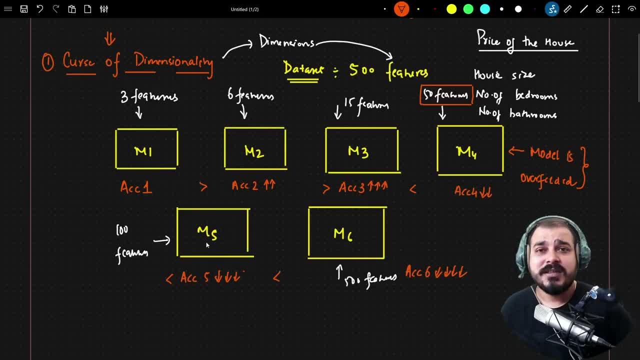 there may be a situation that some of the features may not be at all useful, you know, but still it is. model is basically getting trained on that and a lot of confusion actually happens within the model itself. why? because see, model is altogether inside. if you probably say right, any machine learning algorithm, those are nothing but mathematical equations. 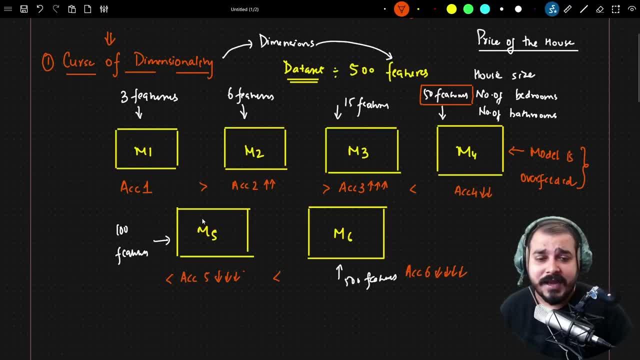 now with respect to mathematical equations. you know, as you keep on feeding new and new features, it will try to learn those features also, even though it is not that important right. so because of that, your model will get overfitted and it will definitely lead to a lot of confusion and 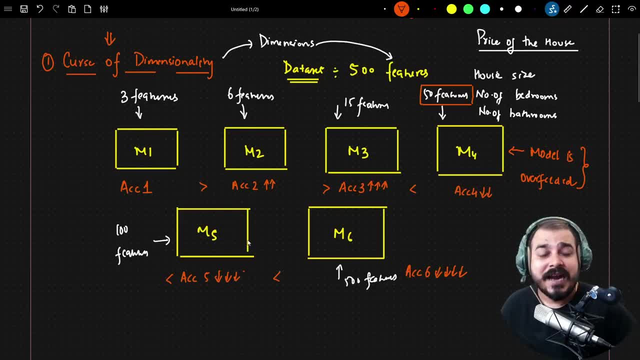 based on that, as the number of features gets increased, your model will start performing like it will stop performing well, you know. at from that point of time, your model performance will also degrade. now here, your second point is that your model performance will also degrade. why? because, as the number of features are increasing, just imagine, the number of dimensions are. 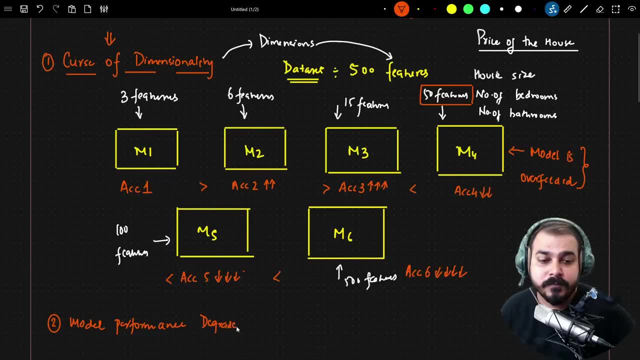 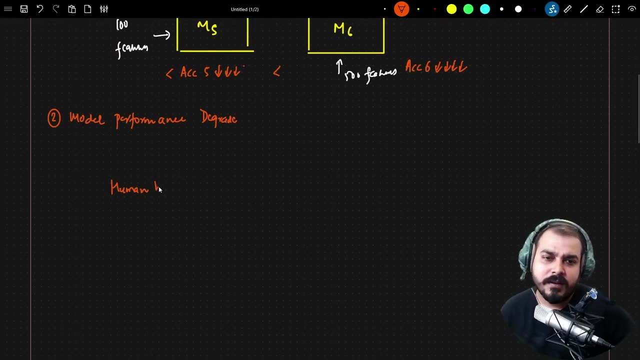 increasing your model performance will degrade, because now the mathematical, mathematical calculation will happen for that many number of dimensions. So because of that the model performance will also degrade. Okay, Let me give you a very simple example. Let's say you are a human being. Okay, Let's say there is a person. I'll just consider there's a person over. 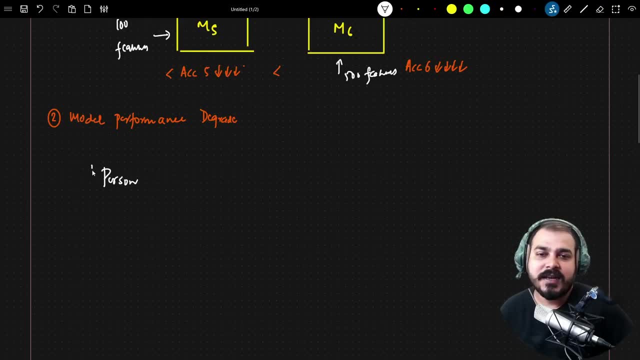 here, Let's, let's say, and suppose I will just ask this person: okay, what is the cost of a house in this specific location? Okay, In location A, what is the cost of the house? Okay, Then the person will probably understand some of the features. Okay, Which location this is. 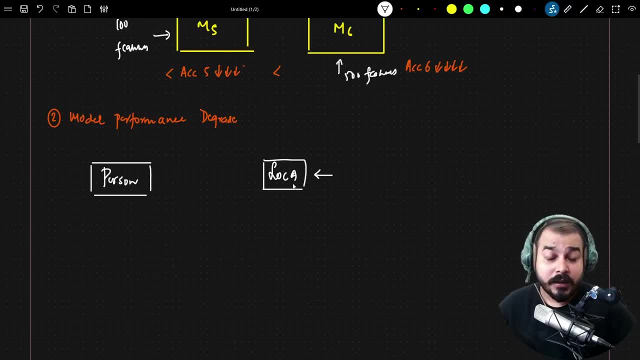 Okay, And let's say he does not have any other location, any other features, So this location may be my feature one. Now, here he may guess that, okay, you're probably, your house may cost between 450K to 500K. Okay, Now you say that no, I specifically want a 3BHK apartment. Okay, Now. 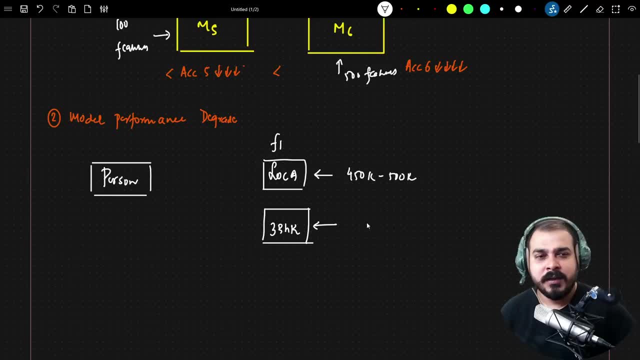 I have got a new feature. Okay, Then he may say that, okay, fine, This was for an average. he, he, he just thought that, okay, this may be an average price for a 2BHK apartment. Now, when he says 3BHK apartment, then he may say that, okay, now your price may be rising. 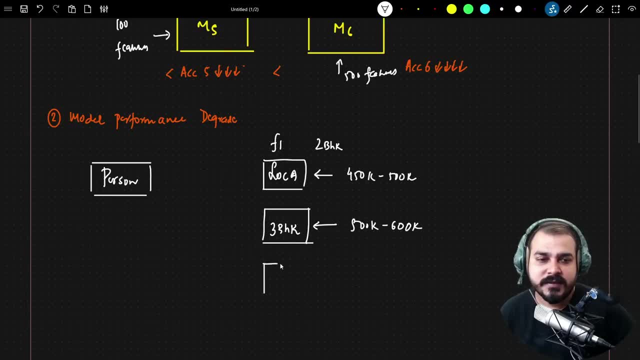 between 600 to 500 to 600K. Then he suddenly says that I need a house near a beach. Okay, Now this particular parameter is added. Now you know that what will happen? The person will start thinking and this price will keep on increasing. Okay, Then let's say, after some point of time, 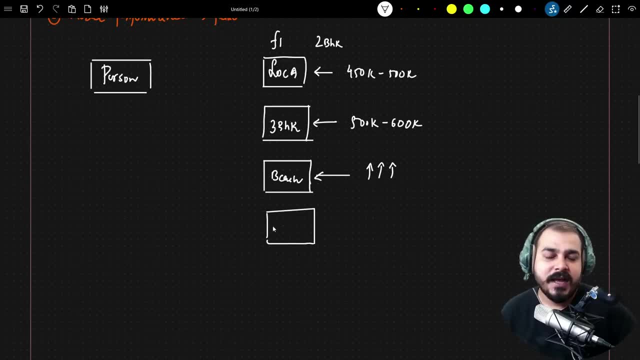 the person demands increases The other person who wants to buy the house. he says that I want a house near to a celebrity. Okay, Near to a celebrity house. So let's say, now this particular feature is also added. Now, here again. 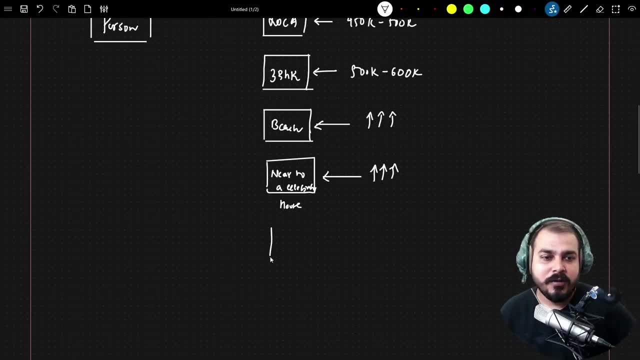 the price will keep on increasing like this. It'll keep on increasing. Now, suddenly the person says: now I also want something like in: uh, beside my house, there should be a lot of grocery shops. Now this particular feature may not be that important to basically increase the price or not. 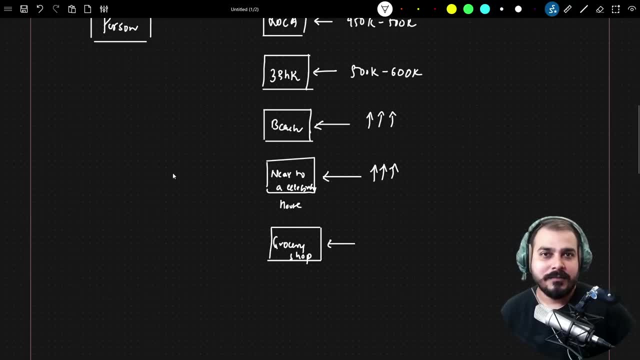 but still, we are adding this particular feature for training our model Right Now. what will happen? You know, this may create an impact, but it will create very less impact. Okay, Then suddenly you'll be saying that: okay, how many number of? 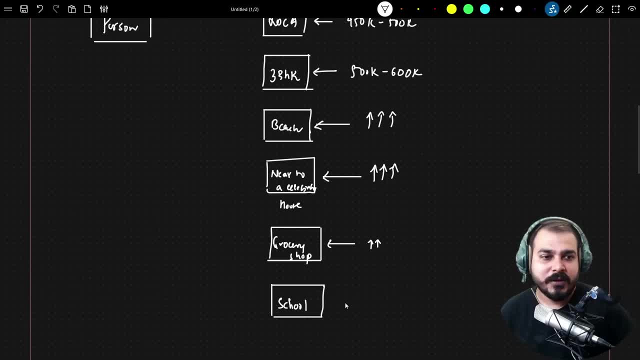 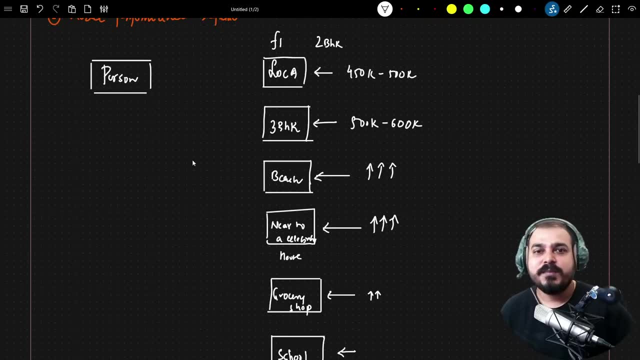 schools are there surrounding my uh, surrounding my house, Then suddenly one more feature will keep on getting added. Now, as soon as we keep on adding this many multiple things, this person who is about to say the price right, he will also get confused at one point of time. 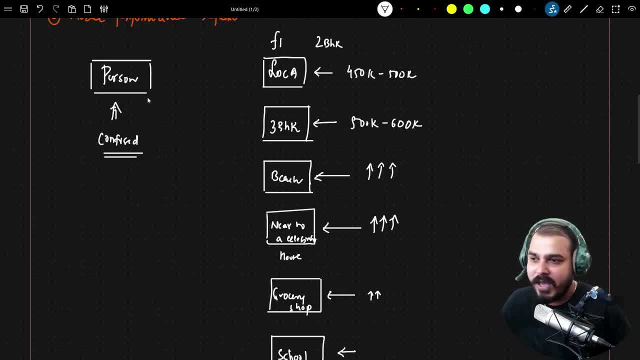 Might, because we are just feeding him with multiple features. Okay, I want this, I want that, I want this. so now the person will still get confused and he will not be able to tell you the proper price. that basically means the performance of this particular person, who's a domain expert in. 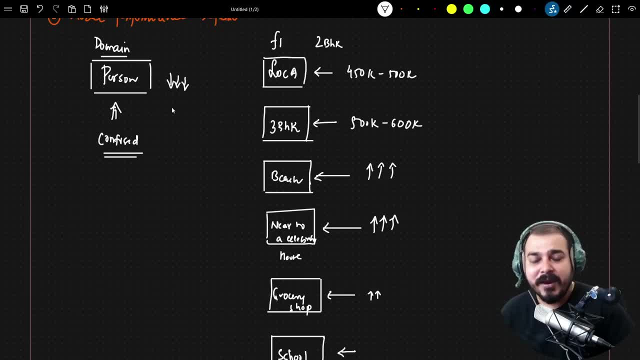 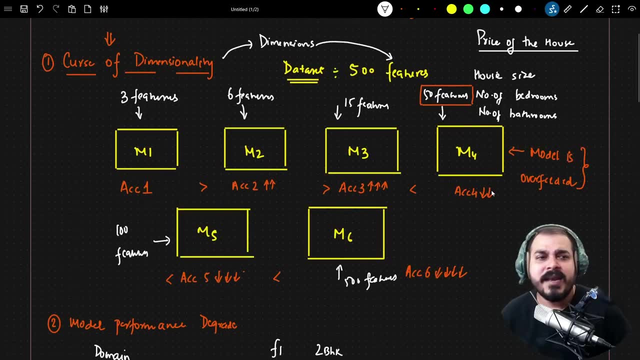 telling you the price range of the houses will decrease, and he may also not be able to tell you the accurate result. and this is the same thing that is happening when we train our model with many, many, many features. that is where your curse of dimensionality comes to picture. 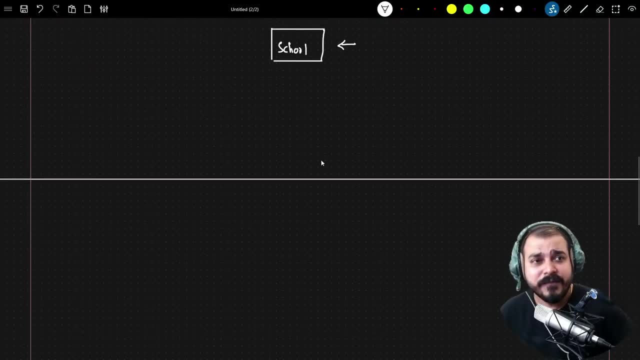 now the question rises: how do we prevent it? there are two different ways how to remove this curse of dimensionality. so two different ways to remove curse of dimensionality. one is feature selection. now, what does feature selection will be saying that we will try to take the most important feature. 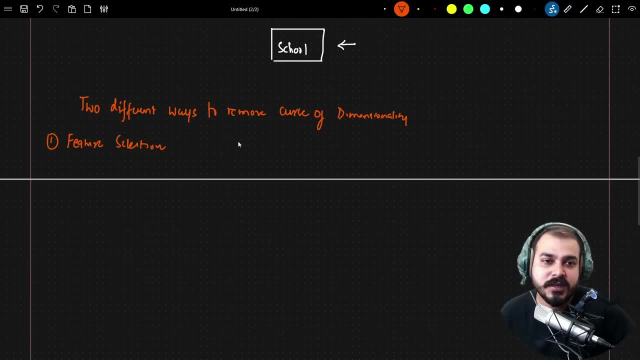 and then we'll try to train our model. that is what happens in the feature selection. the second technique which we are going to discuss in the series is something called as pca, and i'll not just write pca, i'll just say dimensionality reduction. and in this series we 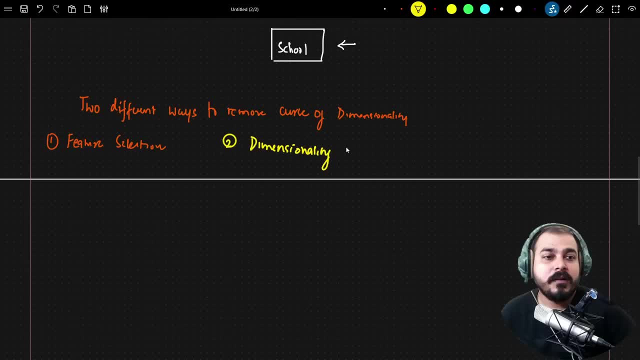 are going to focus more on dimensionality reduction, and in dimensionality reduction there are again many, many algorithms. we'll start with pca. that is principal component analysis. okay, so two ways to remove curse of dimensionality. one is through feature selection. in feature selection, what we do is that we try to take the important features and then we train our model. 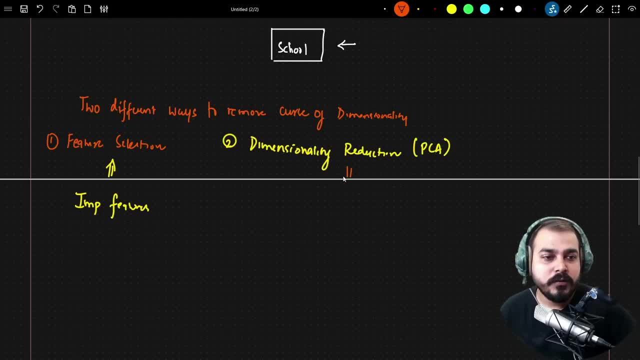 whereas in the case of dimensionality reduction, what we do, we do, and this process is basically called as feature extraction. okay, feature extraction now. feature extraction basically says that we'll try to derive a feature from a set of features. you know where we will be capturing much essence of the previous feature. let's say that i have features like f1, f2, f3 and 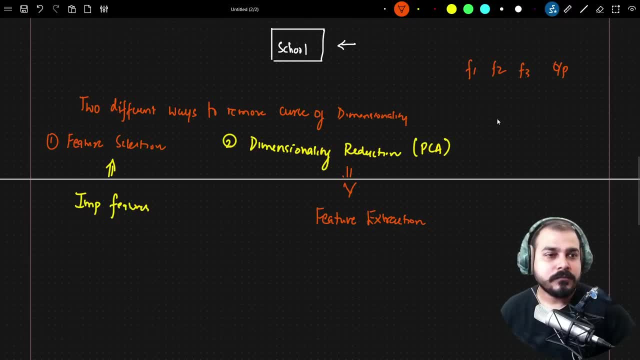 this is my output. what we'll do is that we'll try to derive- we'll try to derive- a feature like f1 and, let's say, we'll try to derive a new feature- this is d1 and d2- from out of these three features and 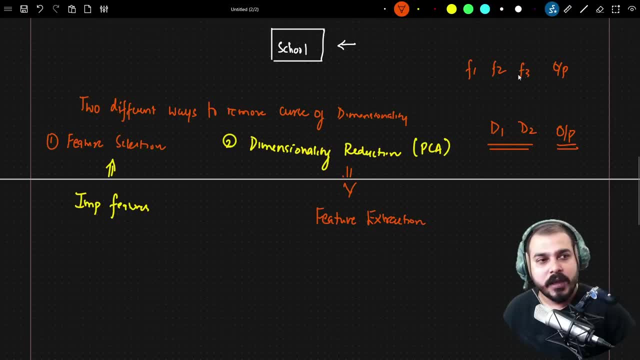 we'll use these features to basically find out our output. okay, then we'll try to see that. how do we derive this particular feature and all everything? in short, we are extracting this new information. so that is the reason we say this feature is important to us and we're going to try to derive. 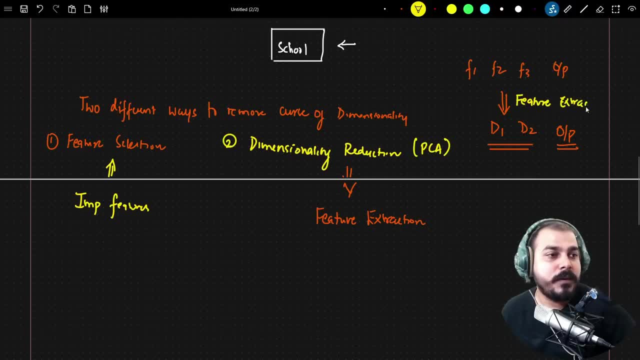 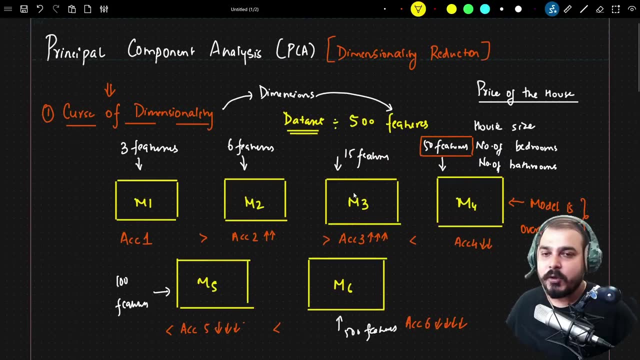 this as feature extraction, Super important topic. Okay, So I hope you got an idea about what is curse of dimensionality. In brief, if I tell you that, as we keep on increasing the number of features, those features, at one point of time when we are training those models, my model will. 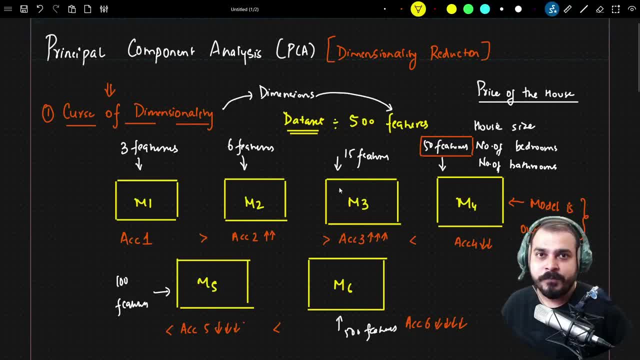 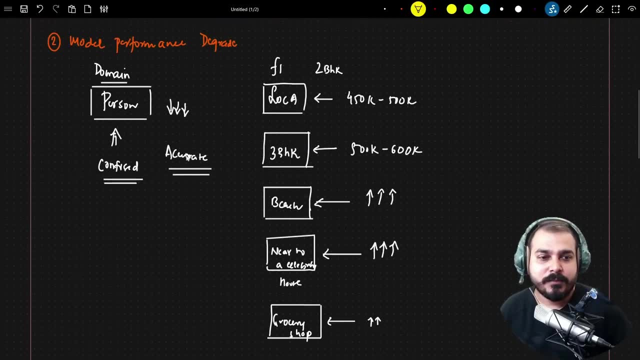 get confused because I have so many features to learn And because of that, the performance of the model will basically degrade. And I have also given you an example with respect to a specific person. right, If you keep on adding features and if you ask this domain expert, what may be? 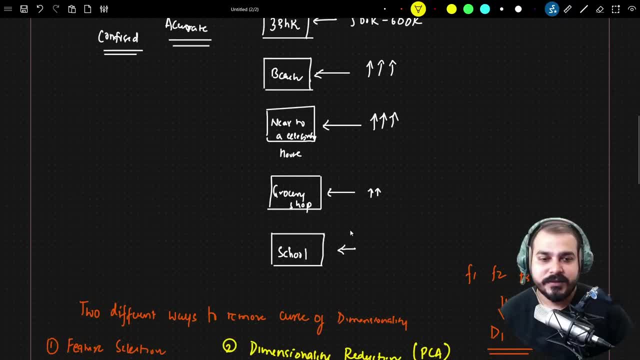 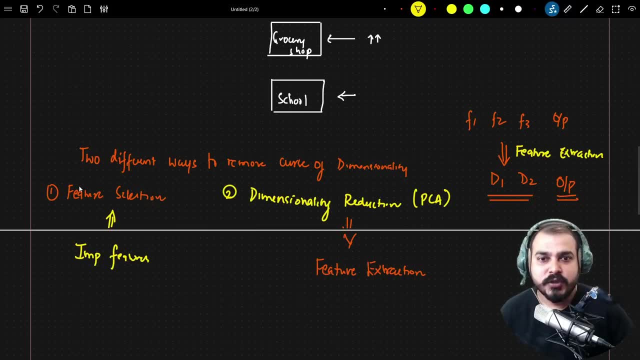 the price, then he or she may also get confused with respect to this right. So how do we prevent or remove curse of dimensionality? There's two techniques. One is feature selection And the other technique is something called as feature extraction. In feature extraction we are going. 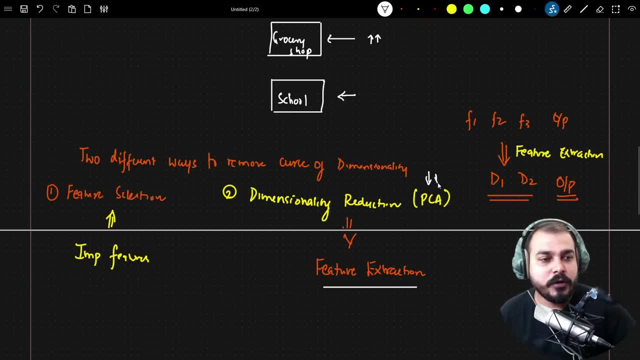 to learn about the first technique, which is called as dimensional reduction, And in that we are going to learn about this algorithm which is called as PCA. Okay, In short, we will be extracting some features For out of the previous features. So this was my original feature And out of this we will be. 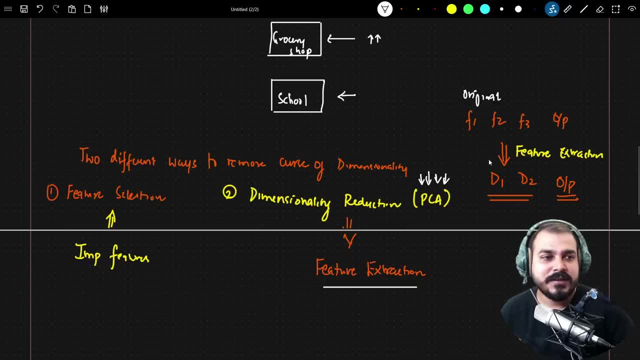 extracting some features like this. it may be in lesser dimensions And obviously, remember, this will be in the lesser dimensions And we'll try to capture the essence out of all these original features, the the same essence of variance, I can also say, and then we'll try to derive this: 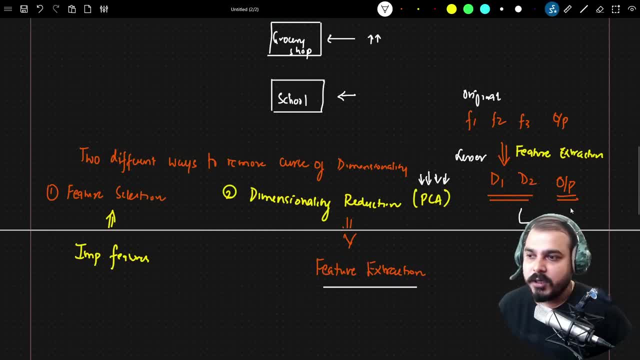 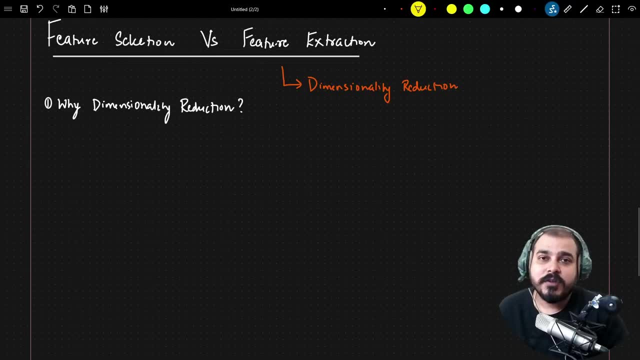 particular feature which will be able to perform well when we are training our model. In this section, we are going to discuss the differences between feature selection versus feature extraction, And this techniques, as you all know, is used in dimensionality reduction, which will 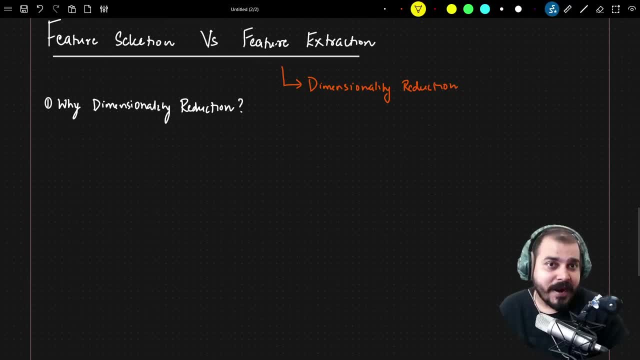 actually helps us to reduce the number of features or to extract some important features from the older features that we already have. Now, before we go ahead and understand about this, we really need to understand why should we perform dimensionality reduction? So here I'm going to. 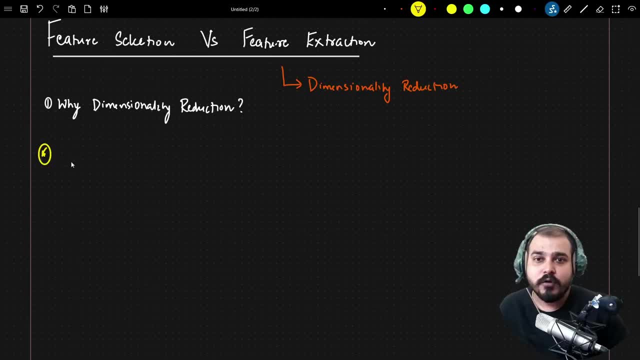 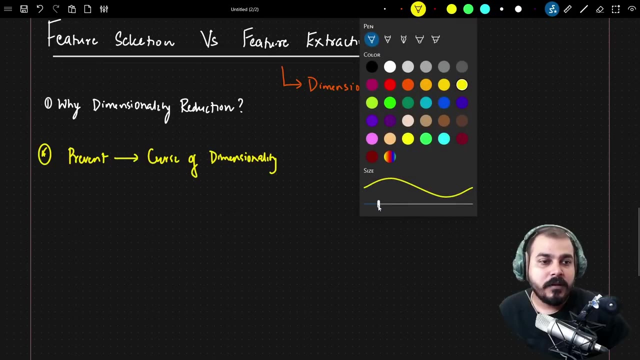 note down some important points, And this can also be an interview question. The foremost reason is to prevent curse of dimensionality. So that is the reason why we specifically use dimensionality reduction. Coming to the second point, coming to the second point over here is that to improve the 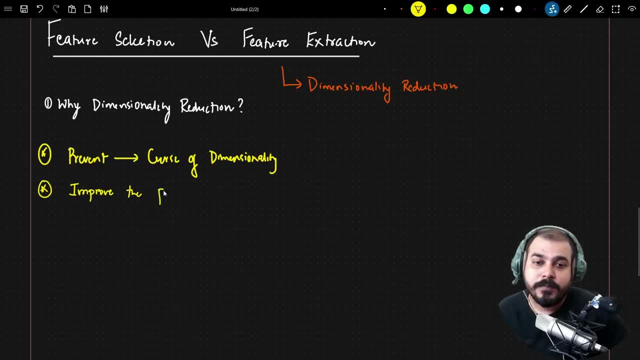 performance of the model. to improve the performance of the model, Now just imagine guys in your data set if you have 100 features, that basically means 100 dimensions are there Obviously to train the model? right, Because in every model when the training happens, some mathematical 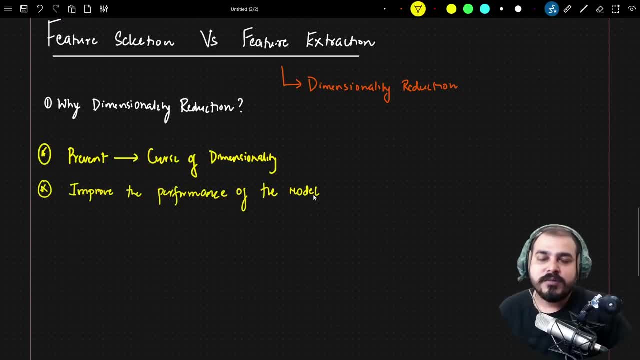 equation is already present over there, right? So those mathematical equation gets applied to all the 100 dimensions, right? So because of that, it may take more time for training of the model. So basically, to improve the performance of the model we can also use dimensionality reduction. 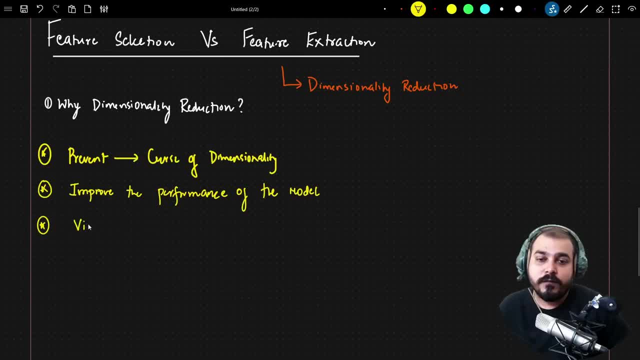 The last point that we are going to discuss is super, super important: to visualize the data And, at the end of the day, once we are able to visualize, we will also be able to use dimensionality reduction. We will also be able to understand the data. Now you may be thinking what exactly this is. 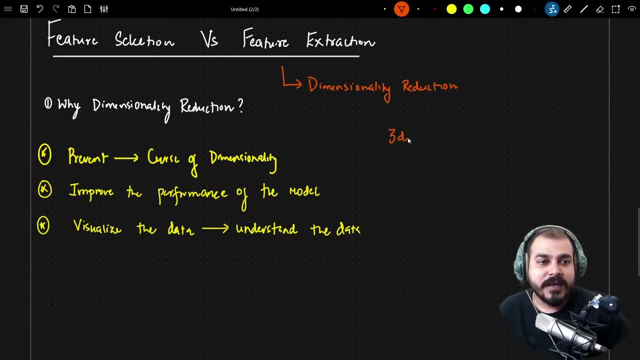 Guys, we human being, you know we can, at the max we can see in a three dimension way. We can visualize anything in three dimension, right, That is in 3D. You can also visualize in 2D, right. We cannot visualize 4D or any dimension that are higher. 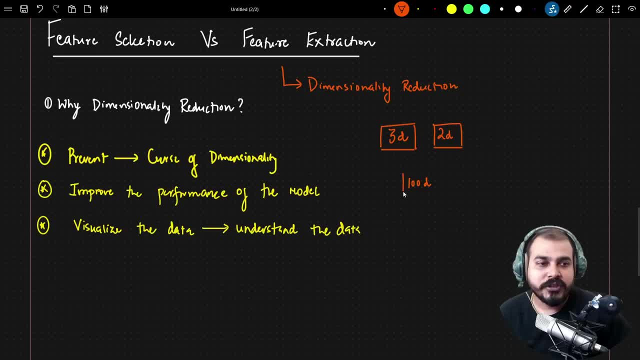 than 3D. right Suppose, if in my data set I have 100 dimensions, obviously I cannot visualize this. So, in order to understand this data, what I can do? I can reduce the number of dimensions to 3D or 2D And I can also see this particular information clearly in front of my eyes. 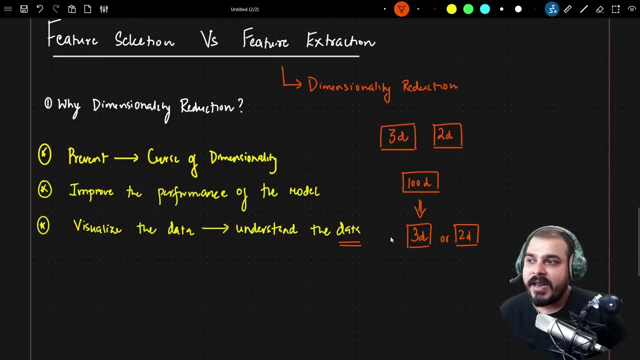 so that we will be able to understand the data right. So if in any interview question, if someone asks you why do you specifically use dimensionality reduction, You should definitely talk about these three points. One is course of dimensionality, which I have already explained. Improve the performance of the model right, Visualize the 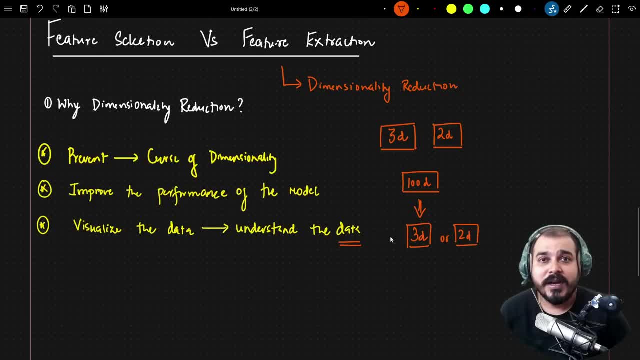 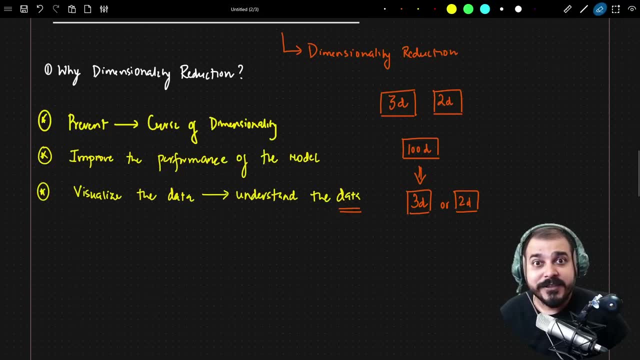 data. If you really want to visualize that data in 2D, 3D or 1D mode, you can definitely use dimensionality reduction, And the major aim is basically to understand the data. Now let's go ahead and discuss about feature selection. Okay, So this feature selection is? 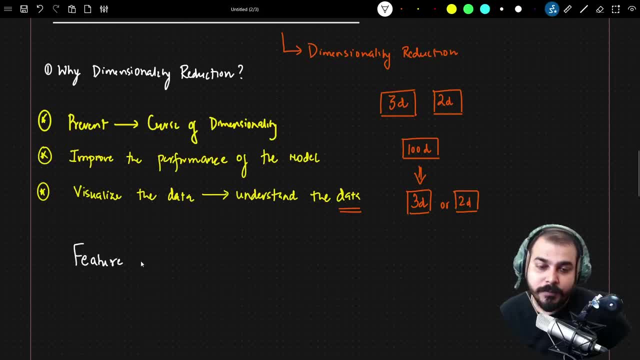 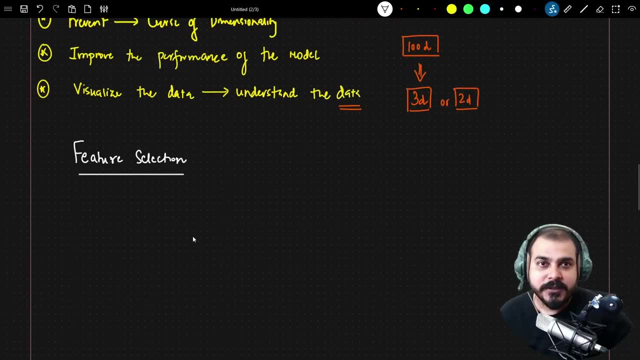 a process wherein it will help us to select the most important feature, which will actually help us to predict the output. Okay, Now, in order to understand the feature selection process, uh, let's consider that I have a feature which is called as X. 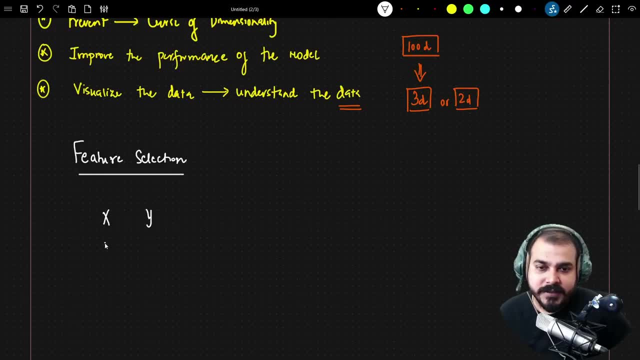 And I have a feature that is called as Y. Now, let's say, I have some data points over here, something like this: Now, with respect to this, if I say, when my X value is increasing, my Y value is increasing, And if my X value is decreasing, my Y value is decreasing. 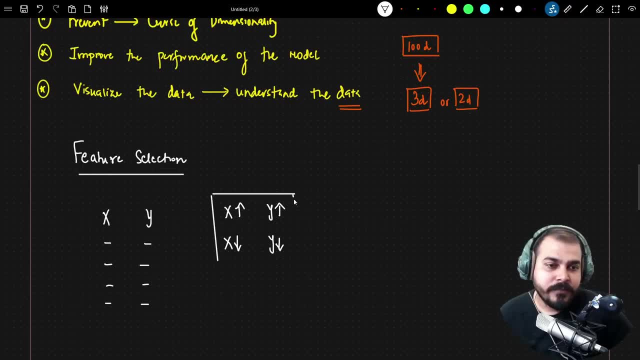 So here I can definitely say there is some kind of relationship right In this particular scenario, that is, when the X is increasing, Y is increasing, And when the X is decreasing, Y is decreasing. Similarly I can have one more relationship wherein when my X is decreasing, my Y is increasing. 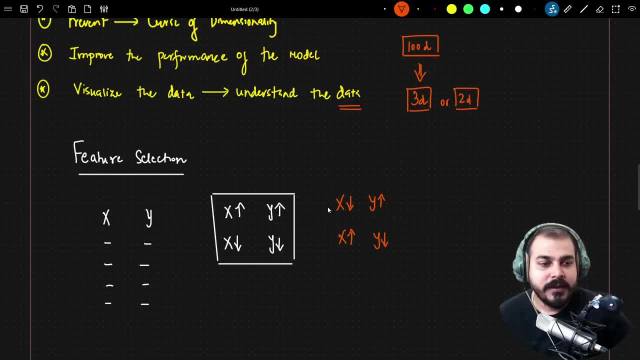 and when my X is increasing, my Y is decreasing right? So this is also another relationship that I can have between X and Y And in this particular case, let's consider X as my input feature and Y is my output feature. right, With respect to X, I need to predict what is Y. 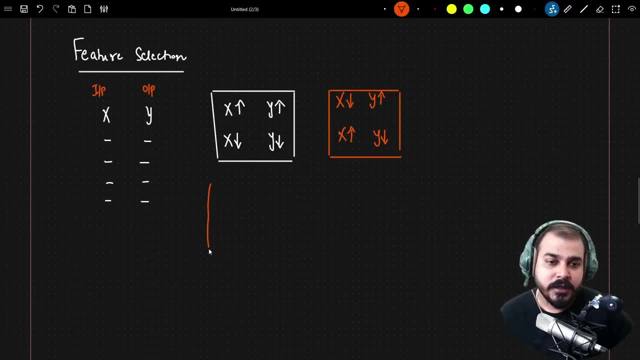 Now, whenever I have this kind of relationship, then here you'll be able to see if I plot with respect to X and Y, I can have one more relationship, right. Similarly, I can have one more relationship axis. here you'll be able to see. all the data points will be in a linear relationship, right. 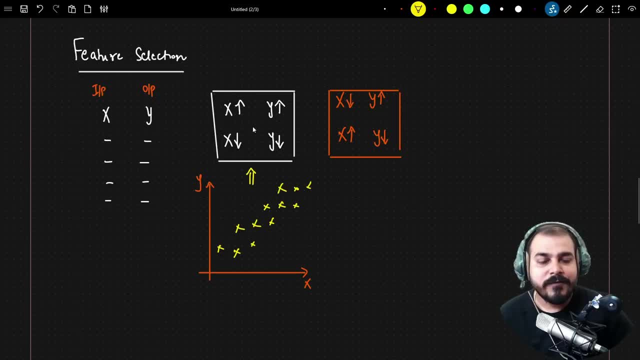 when it is in a linear relationship, then it will probably follow this particular approach. where x is increasing, y is increasing and x is decreasing, y is increasing, and that is true in this particular case. when x is decreasing, y is increasing right now. similarly, in this particular case, if i probably want to draw a scatter plot, my scatter plot will look something. 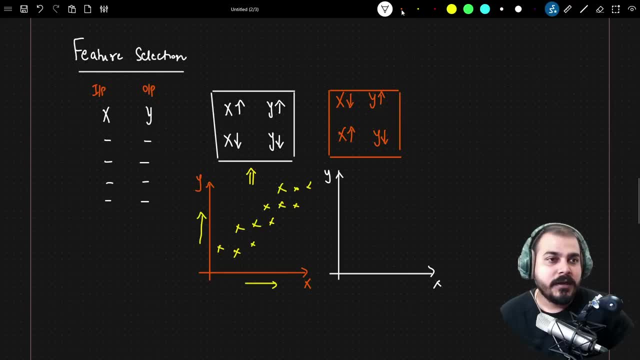 like this with respect to x and y. right now, if i probably try to see this, all the points will be in this inverse relationship. now, whenever we have in this inverse linear relationship, then you'll able to see that it will follow this specific approach. in this particular case it will follow. 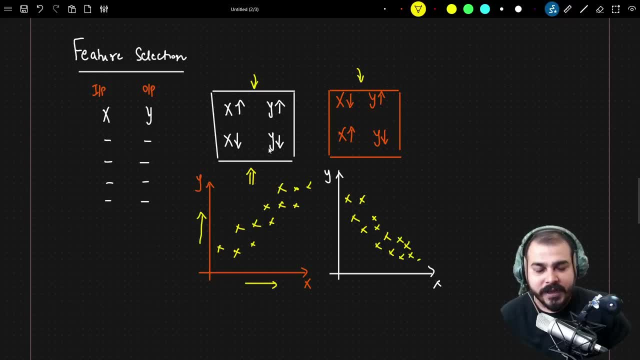 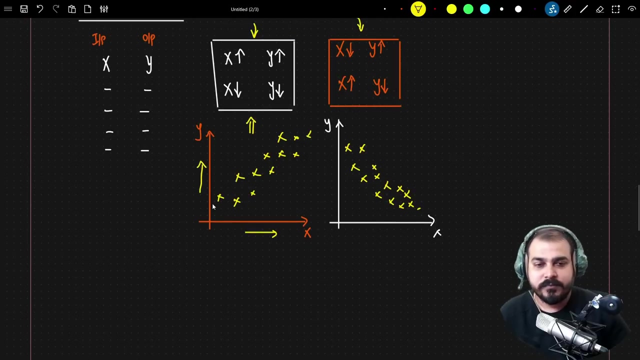 this particular specific approach. now, obviously you know that when you have this kind of linear relationship, then definitely x value will be very, very helpful in finding out the y output, and mathematically we can also find out a way to quantify this relationship, and the technique that we specifically use in this is something called as covariance. okay, so here. 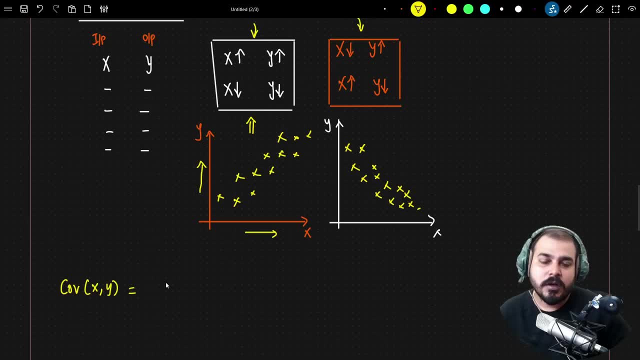 if i really want to find out the formula between covariance of x comma y, the formula that is used is: summation of i is equal to 1 to n. x minus x bar multiplied by y minus y bar divided by- and here i'll write x of i, y of i divided by n minus 1, since we are doing it for sample data, that is: 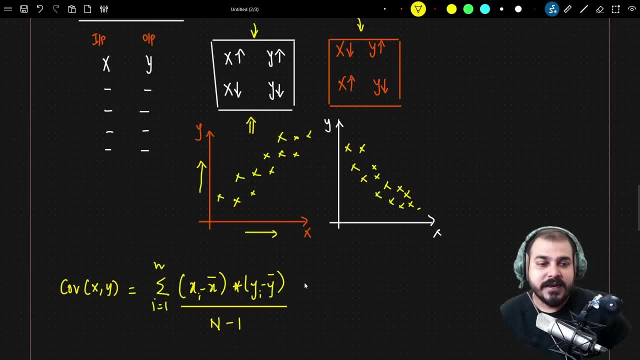 the reason we use n minus 1 now in this particular case. let's say, if we are going to get a positive value, if it comes as a positive value, that basically means we are going to follow this specific relationship. if it comes as a negative value, then we are going to follow this specific. 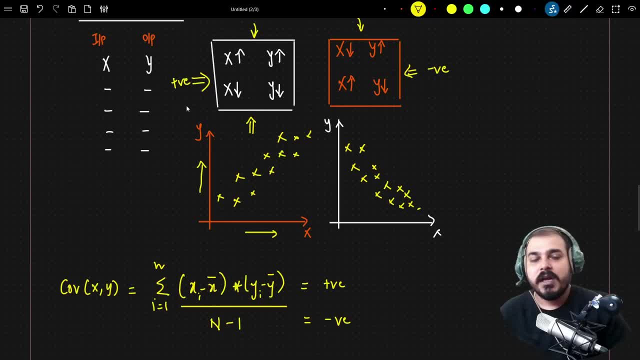 relationship. so for this, whenever we get negative, we are going to follow this. whenever we get positive, we are going to follow this. that basically means the relationship between x and y will have this kind of relationship. that is the linear relationship. when my covariance is positive, when my, when my covariance is negative, it will follow inverse, real, linear relationship. 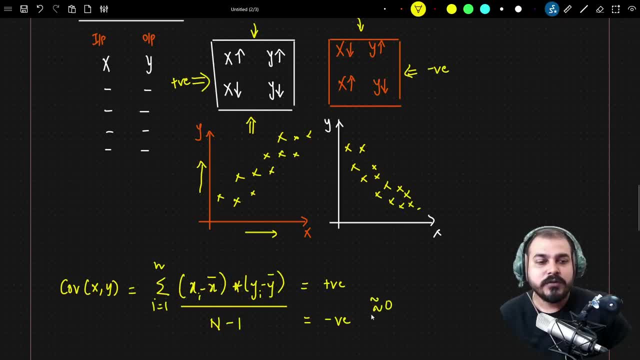 and along with that, let's say, if my covariance is approximately equal to 0, that basically means there is no relationship between x and y, no relationship, no relationship between x and y, no relationship between x and y. so if i try to plot this in this kind of day, a scattered plot with respect to x and y, i will. 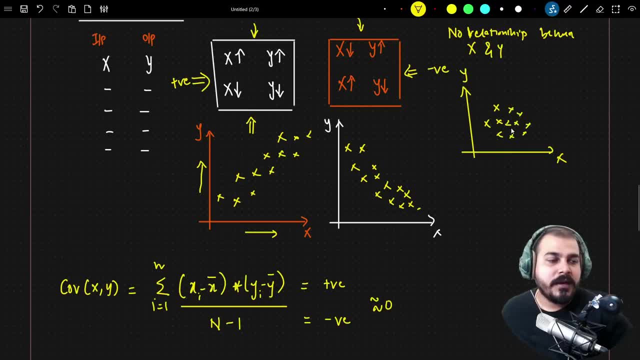 be just getting a scattered plot which may be in circular way, and here you can not definitely find out. uh, the relationship between x and y. that basically means, when x is increasing, whether y is increasing or not, or whether y is increasing or y is decreasing, whether x is increasing or not. 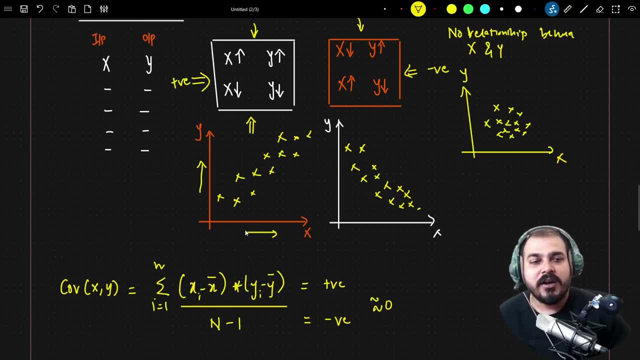 right? so whichever have this kind of highly positive co-relationship- sorry, covariance, highly positive relationship, which we basically calculate through covariance, we can definitely say that those features are super important features, right? so in this particular case, i can definitely say that if i get a covariance as positive, i can definitely say x is a super important feature. 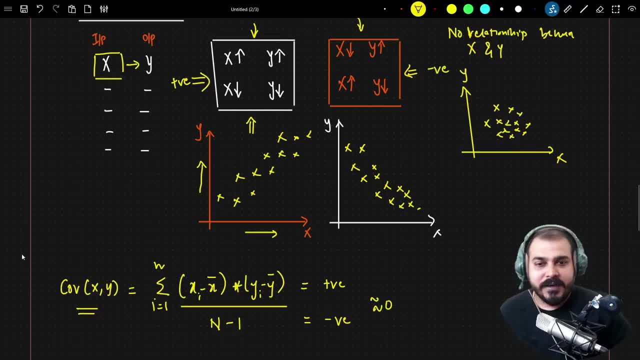 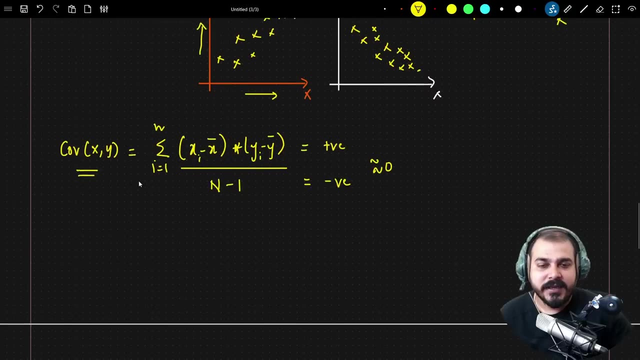 and it will definitely be helpful in predicting y. but if i get the covariance between x and y as 0, i'll definitely say that there is no much relationship between x and y. right, so i can definitely remove this specific feature also, right. Now let's understand. along with covariance, there is also a technique which is called as correlation, and we basically say it has Pearson correlation. 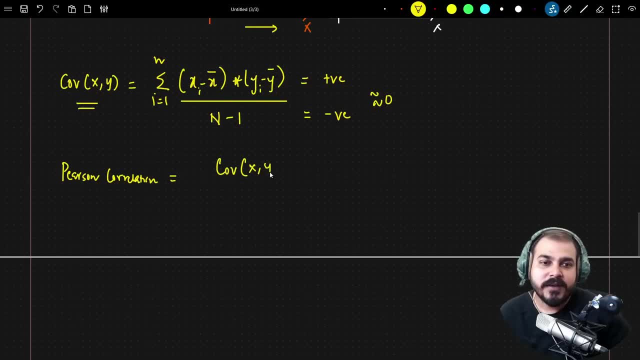 And Pearson correlation can be given as a formula of covariance of x, y multiplied by standard deviation of x multiplied by standard deviation of y. Now, with the help of this, your correlation will be ranging between minus 1 to plus 1.. In this case, there is no such range. It can be any positive value. it can be any negative value. 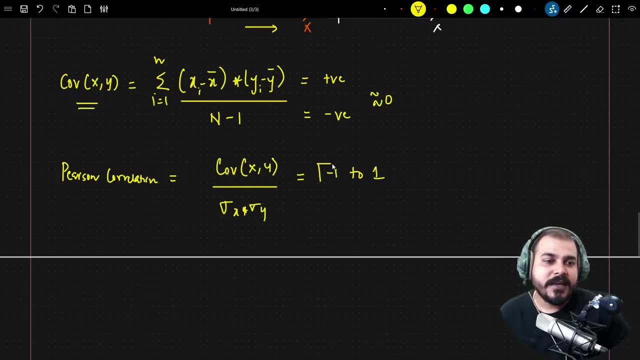 But with the help of Pearson correlation coefficient, you will be getting your value between minus 1 to plus 1.. The more the value towards plus 1, now understand this is a super important point- the more towards the value of plus 1, the more positive correlation it is. 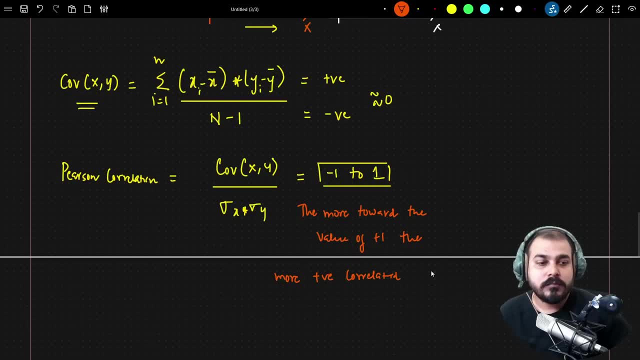 The more positive correlated it is, And the more the value towards minus 1, the more negatively correlated it is. So the same thing gets applied to minus 1, the more negative correlated it is, And similarly, if my correlation between x and y is near to 0, that basically means no relationship. 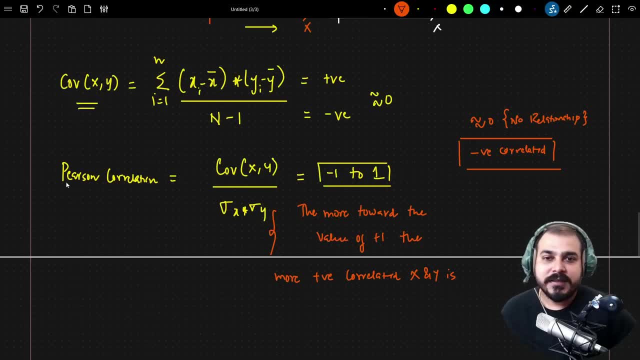 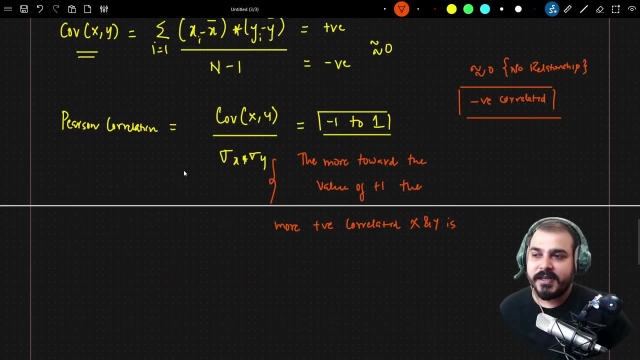 Okay, Now this was an idea to talk about the relationship between x and y, Now how this works. So this particular process is basically used in feature selection. This is just one of the techniques, guys. There are other techniques also in feature selection. 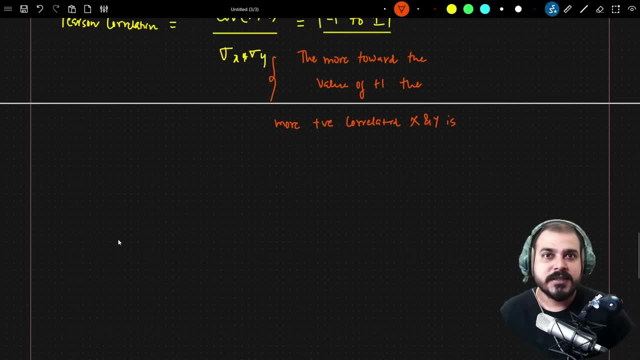 But I just really want to give you a brief idea before we go ahead and understand PCA. Okay, Let's say I have a specific data set And let's say this is my housing data set. In this data set, let's say, I have features like house size. 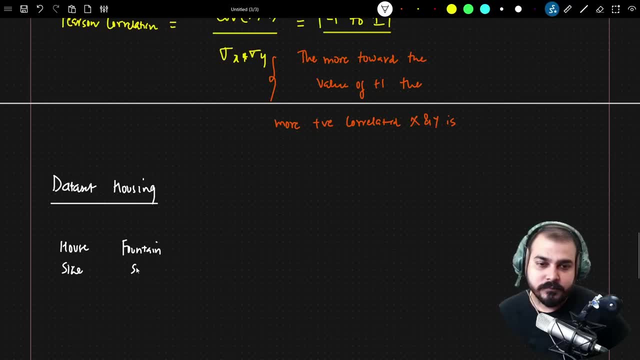 The other feature that I have is something called as fountain size. Let's say that this house, These houses, are present within an apartment and we are also going to take this as a property to predict the price of the house. Now, in this case, these are my independent features. 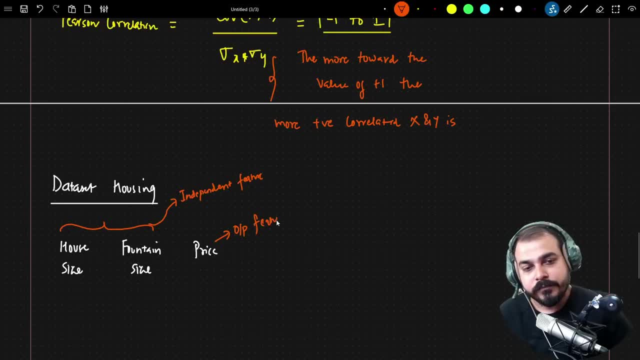 And this is my output or dependent feature. So that basically means I'm going to use this two independent feature to predict the output feature And obviously, when this value changes, this is also going to change. Now, guys, if you just apply common sense, you know that fountain size may not be a very important feature. 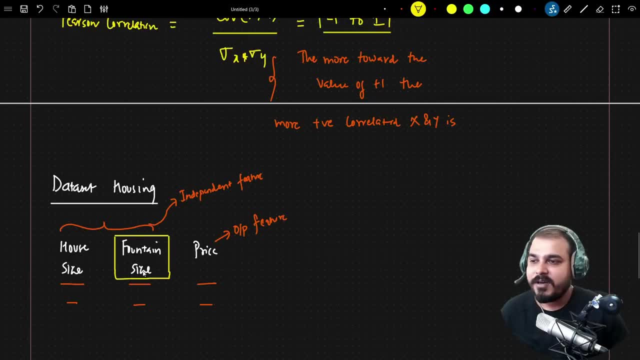 Because obviously, even though you have a bigger fountain, a smaller fountain, it does not mean that your house price will increase within an apartment right, Within a number of apartments, right, And obviously most of the bigger apartments- you know group of apartments- will definitely have some kind of fountain. 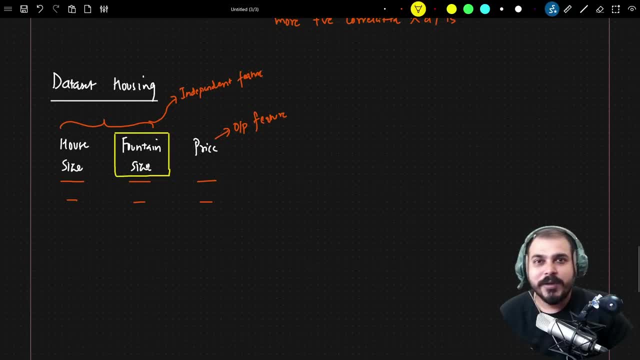 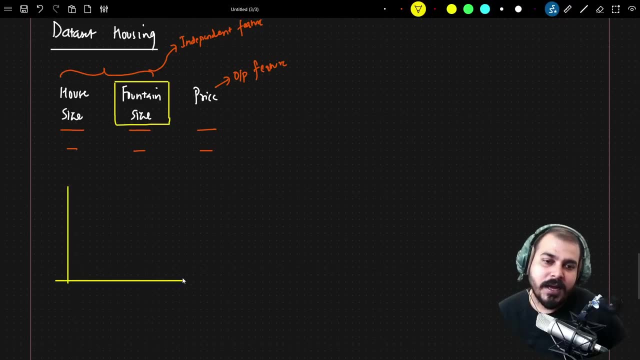 Right, Just to showcase, just to put some nice showcase. this fountain is basically used right Now. if I go ahead and take Each and every feature, let's say, Let's say one of the feature I have taken- house size. 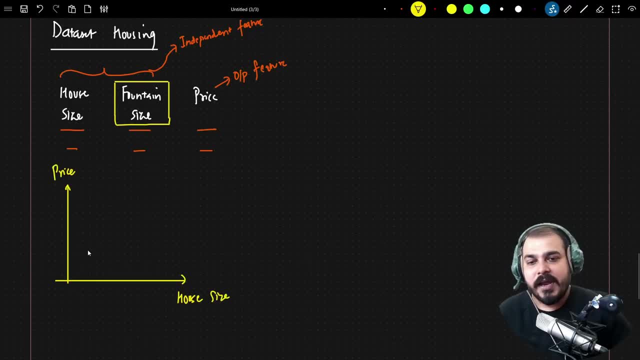 And I have plotted along with the price house And, let's say, if I have found out this linear relationship, definitely this indicates that this house size is an important parameter to determine the price because it has this linear relationship. And how do you calculate the linear relationship? 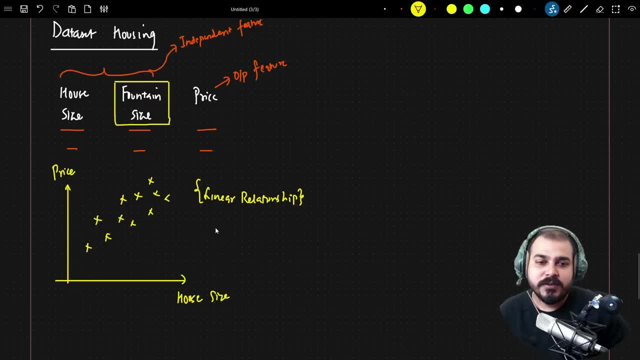 Or how do you quantify the relationship between house size and price? You can definitely use something like covariance And obviously you will either get a very high positive value or, for some other use cases, you may also get some negative co-value, Some negative value, okay. 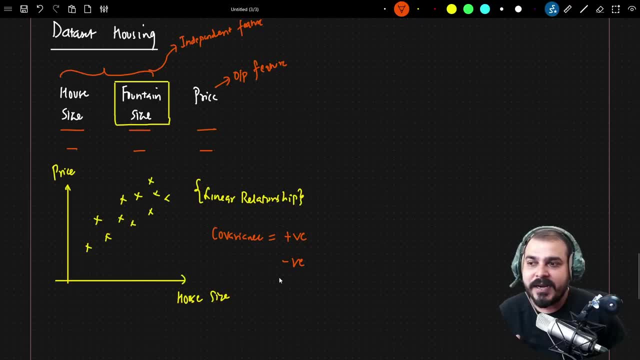 Or you can also apply correlation. That basically means you will be getting your value between minus one to plus one. Now in this particular case you definitely can say house size is an important property And obviously important attribute And just by common sense also you can come to the conclusion: 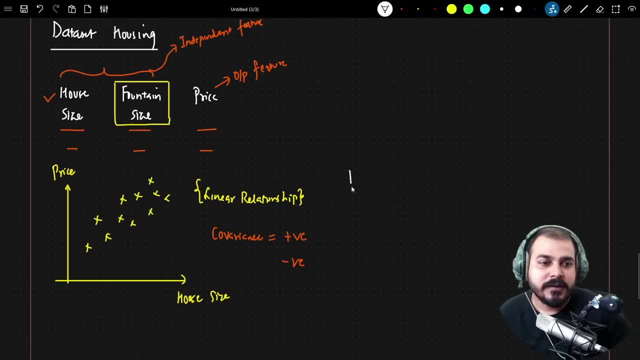 Now, what about the feature that I have taken? Now, what about the feature that I have taken? That is, if I try to plot this feature, that is fountain size and probably price of the house. Now, in this particular case, let's say, my plotting happens like this: 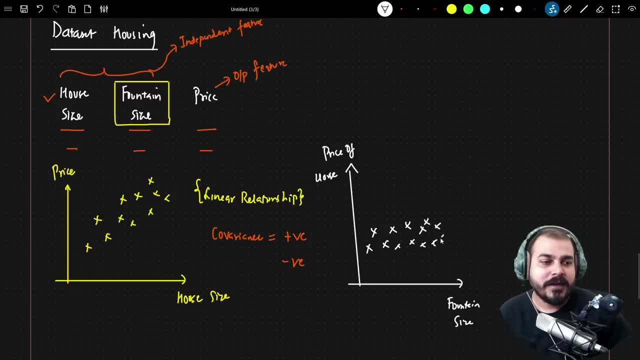 And let's say that this is not at all that much important right Now. here you can clearly see that there is no relationship between fountain size and price of the house. You can see that Here. you can definitely see that even though the fountain size is increasing, the price of the house is stagnant almost within this specific region, right. 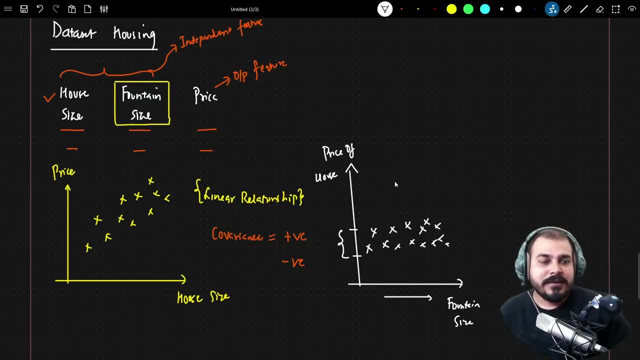 So definitely we can come to a conclusion that the relationship between fountain size and price of the house will be very, very less, or it will be approximately equal to zero, Or let's say it is ranging between zero to 0.25, okay. 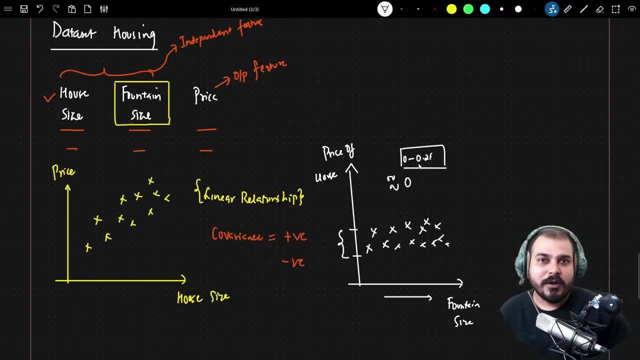 Not that positively or negatively correlated right, Not that positively or negatively correlated right. So in this particular case, what you can do is that you can consider that fountain size is not that important feature and you can drop this feature. Now, these steps that we have performed, we have basically- we are basically saying this as a feature selection process- 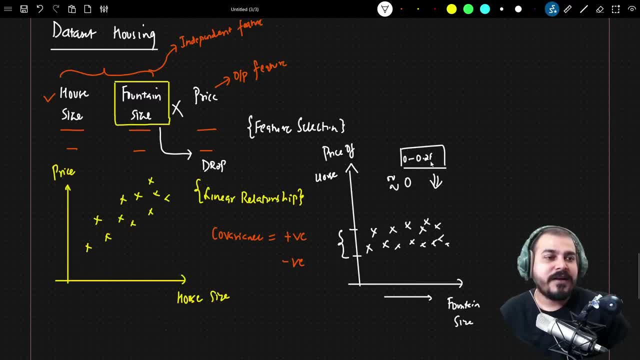 And here you can also make sure that you can apply covariance and find out how a correlation and find out like what is the relationship between this fountain size and price of the house. So this is how you can come to a conclusion whether fountain size is important or not. 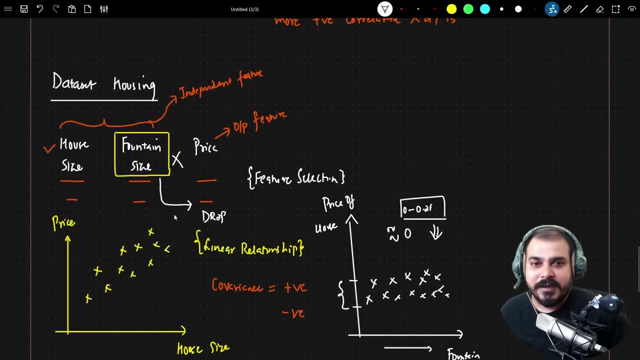 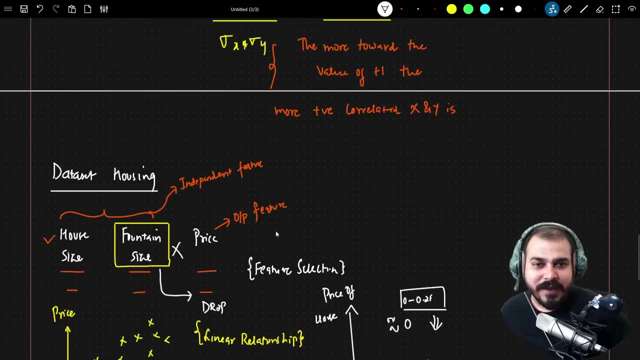 And, based on that, you can basically draw a line. Okay, You can basically drop it Right, And this is what we usually do in the feature selection process. We use correlation and covariance to do it. Okay, Now let's go ahead and discuss. 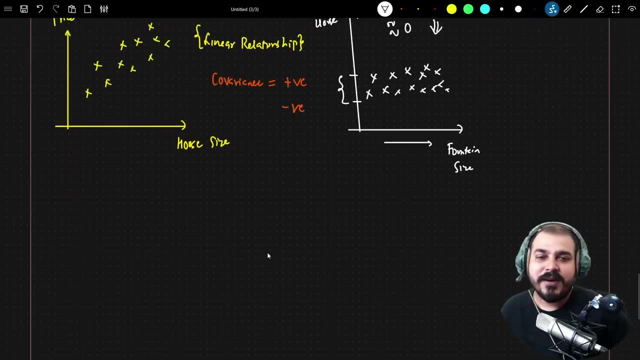 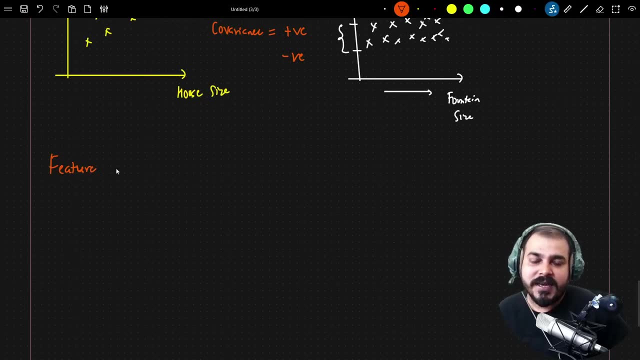 I hope everybody got an idea about feature selection. Now, what we are going to do is that we are going to discuss about an important topic, which is the next topic, which is called as feature extraction. Now, what does exactly happen in feature extraction? 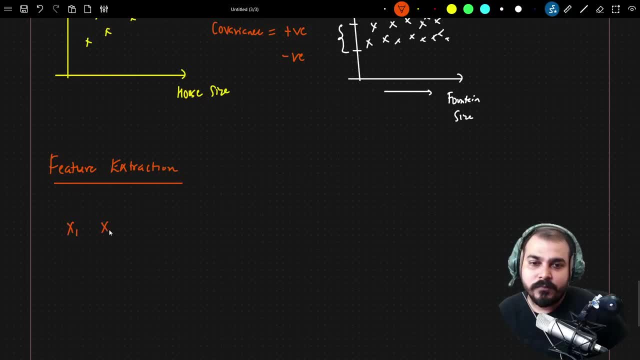 In feature extraction. let's say I have features like X1, X2.. And let's consider the same housing example. Now let's say I have something like house size And let's say I have like number of rooms And finally I have something called as price of the house. 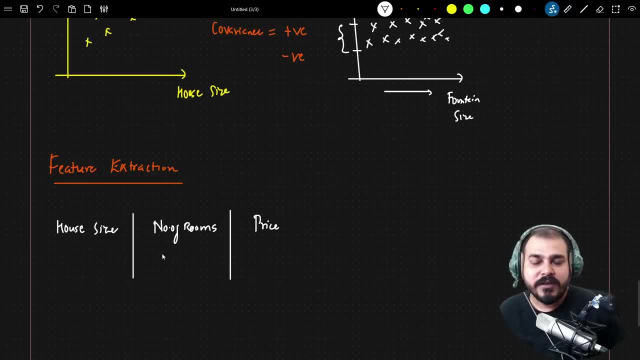 Now, in this particular case, you want to reduce your number of features from 2 to 1.. That is what we are doing, Right? We are in dimensionality reduction. Let's say that I want to reduce my two features into one feature. 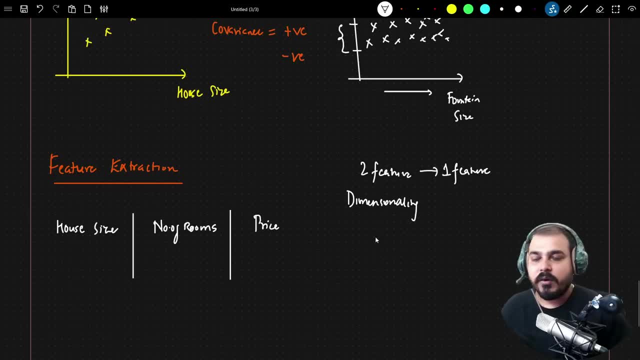 That is what we do Now in this scenario. you know that, obviously. or let's say, instead of house size, you know, I will just write room size. Okay, Room size. Now. here I really want to perform some dimensionality reduction, wherein, from two features, I want to convert this into one feature. 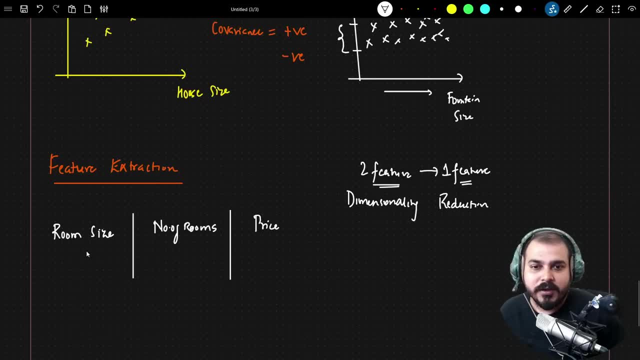 So obviously I cannot use feature selection. Why? Because both these features are super important in predicting the output that is your price. Both these features are super, super important. Right, These are my independent feature And if I also try to find out the correlation or covariance between my input and the dependent feature, here you will always be able to find out either very high positively correlated or high negatively correlated. 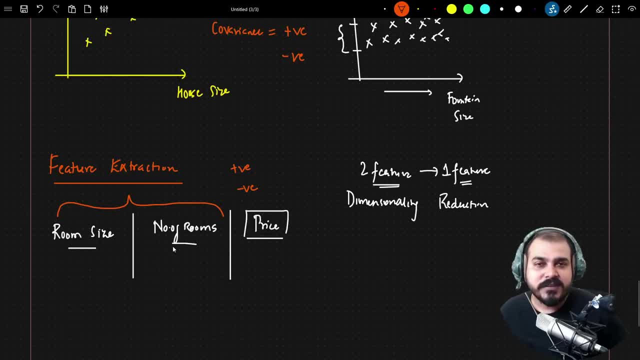 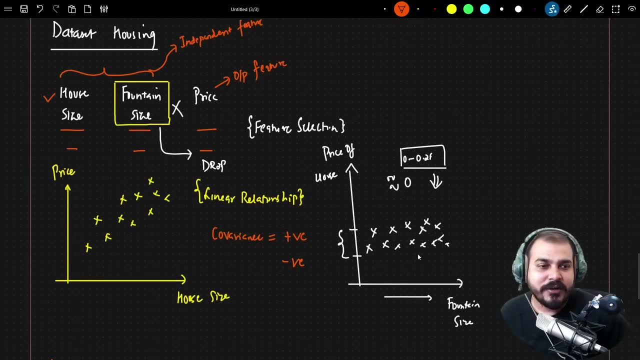 We will be able to find that out, And it is a common sense question. guys, This is obviously going to have a linear relationship with respect to this specific feature. On the top, we basically had fountain size, and I just tried to show you an example by plotting it. 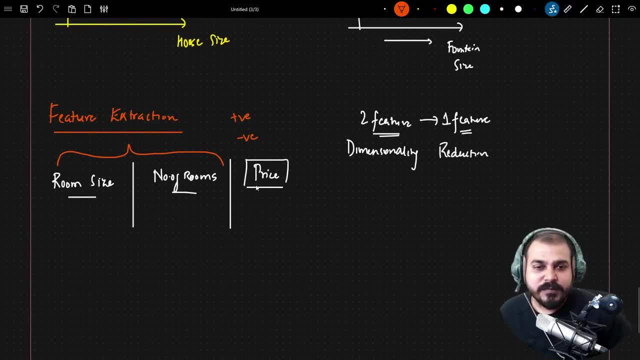 It did not have a much a linear correlation. Now, in this particular case, I obviously cannot drop one of the feature and just consider one feature, because here we can definitely see that there is some relationship between the independent and the dependent feature. So in this case, what do we do? 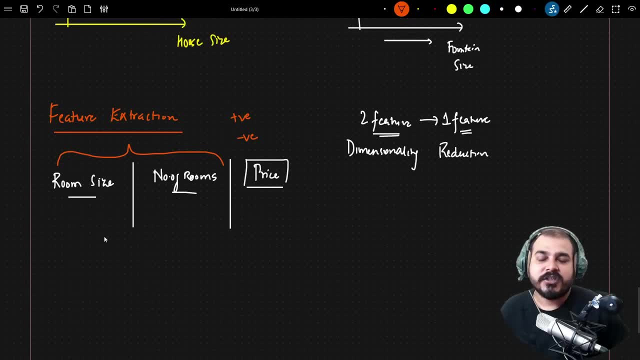 In this case we perform something called as feature extraction. In feature extraction, the core idea is that we take these two independent feature, We apply some transformation. We apply some transformation to extract new feature And let's say this new feature is something called as house size. 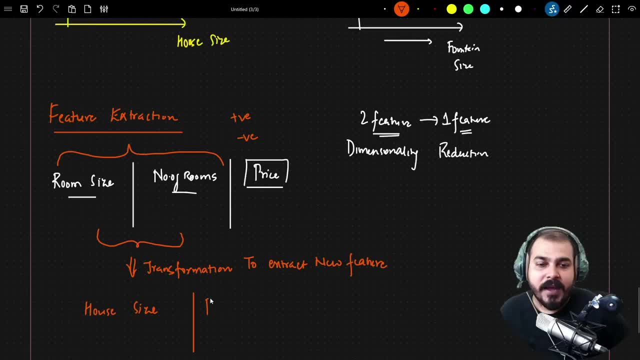 I am just giving as an example And my output feature is something called as price. Now, instead of using these two feature, that is, room size and number of rooms, If I also get to know the information of the house size, then also I will be able to predict the price. 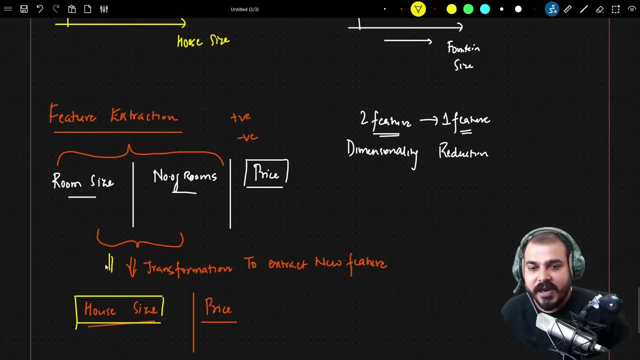 So, in short, from these two features I am trying to derive a new feature, or extract a new feature, which is called as house size. Now just imagine for a domain expert team, If domain expert team is given with these two fields- room size and number of rooms- he or she will definitely be able to predict or tell you the price. 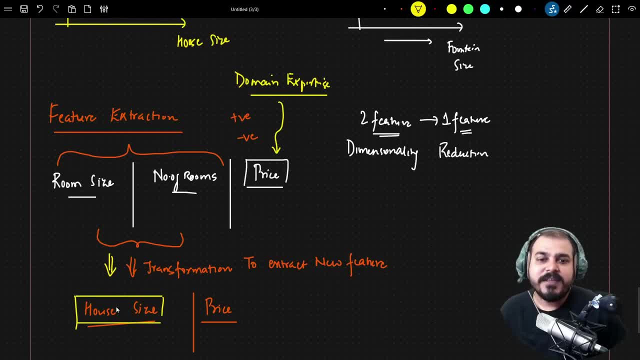 Now, instead of that, Now, instead of giving these two features, if we just give one feature to the domain expert team, Then obviously he or she will also be able to predict the price, with some difference, Right, With some difference. 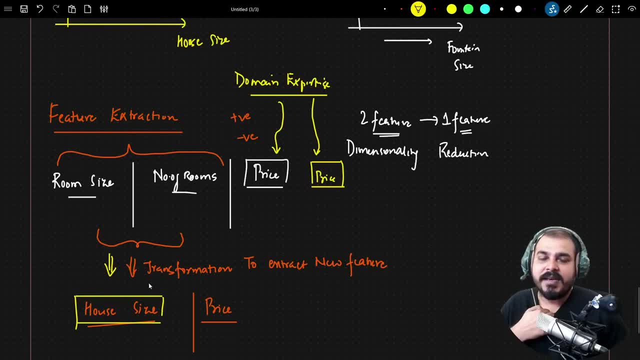 Obviously some amount of information is lost over here. But again, domain expert team will also get some clear idea about like with the help of house size. also, He or she can definitely predict the price. So in feature extraction what we are doing is that. 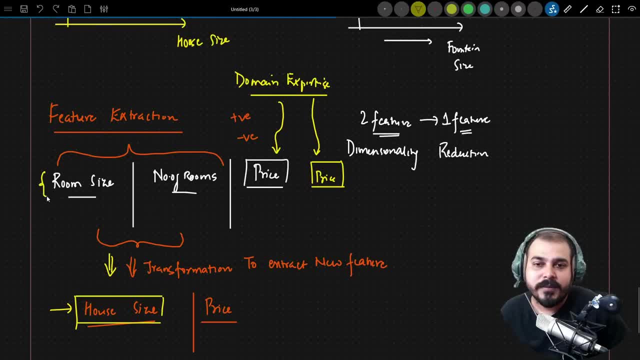 We are trying to extract a new feature from the feature that is already present. Okay, And this is how we basically reduce the number of features or dimensions. Okay, Usually- here the example that I have taken- only two independent features. But, guys, in a real world scenario you will be having 10 to 15 features and we will try to reduce it to 2 to 3 features. 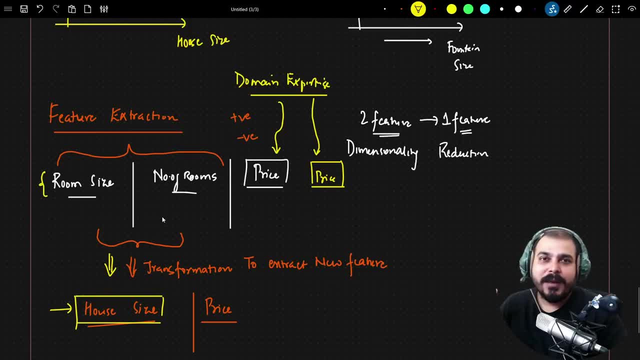 Okay, Now, once I reduce this, I will obviously be able to visualize it in a proper way. I will be able to see it and I will also be able to understand the data. Now, this is the idea behind this. This is the idea behind feature selection versus feature extraction. 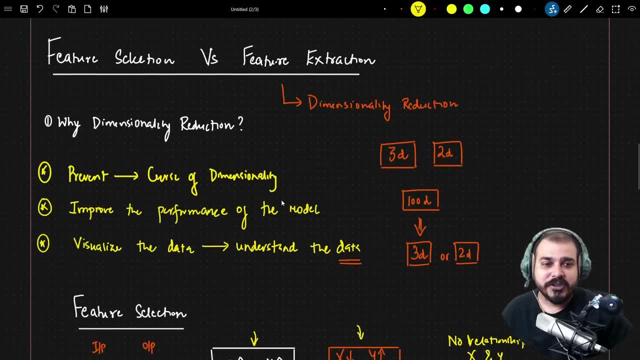 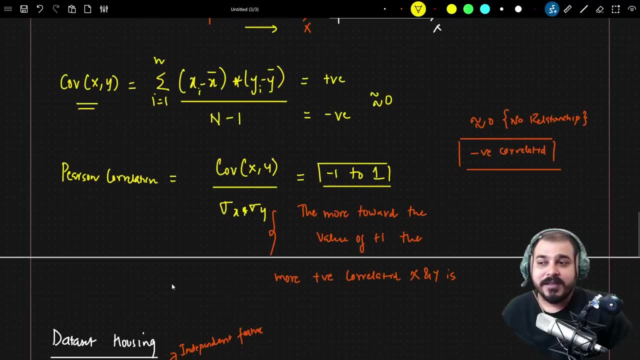 So in this video I have covered so many things. First of all, why dimensionality reduction? Then why feature selection? What is feature selection? What is covariance? What is Pearson correlation? There is also another correlation, which is called as Spearman rank correlation. 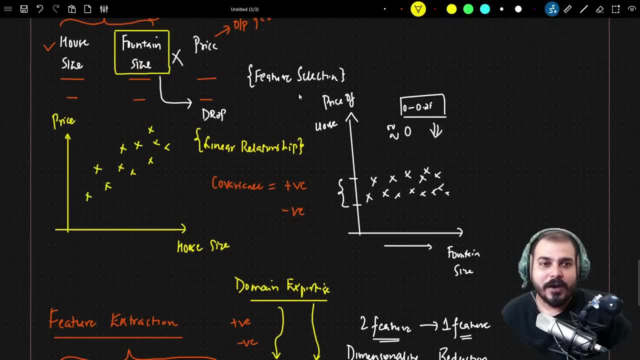 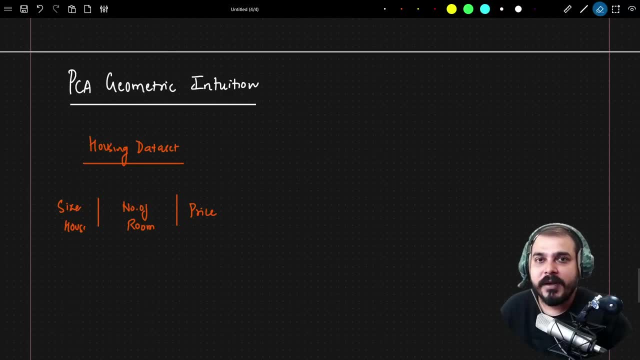 Then we have taken an example with respect to dataset housing. Then I showed you that, how we can go ahead with feature selection And how do we come up with feature extraction. So, guys, Now let's go ahead and discuss about the geometric intuition. 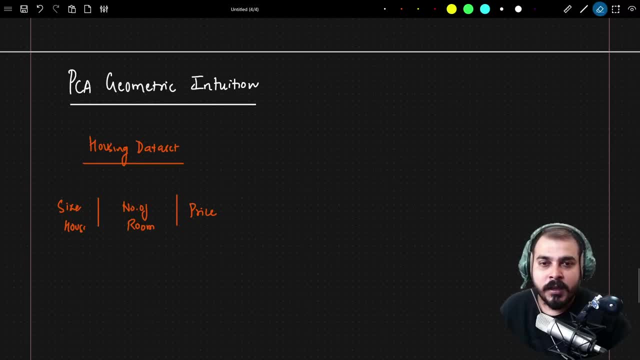 The geometric intuition behind the principal component analysis. Now, obviously you know that principal component analysis is used for dimensionality reduction, Right Dimensionality reduction. That basically means we are going to extract some features with respect to the older features that are present in the dataset. 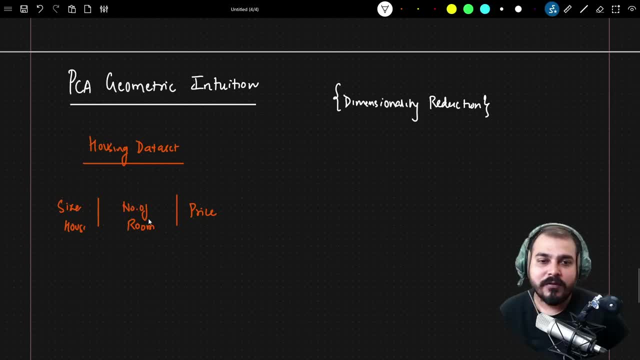 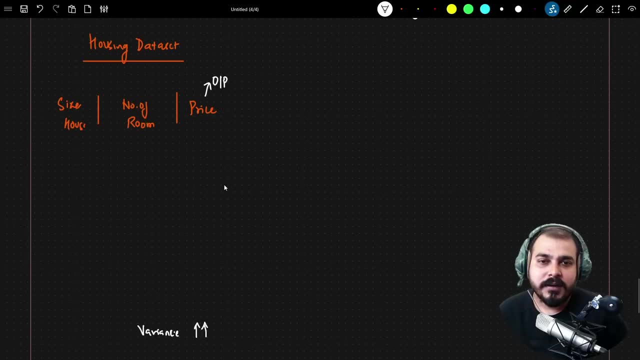 Let's say, I have features like size of the house and number of rooms, And this is basically the price of the house, which is my output feature. Right, This is my output feature. Now, here let's go ahead and probably plot a data point between the size of the house and the price of the house. 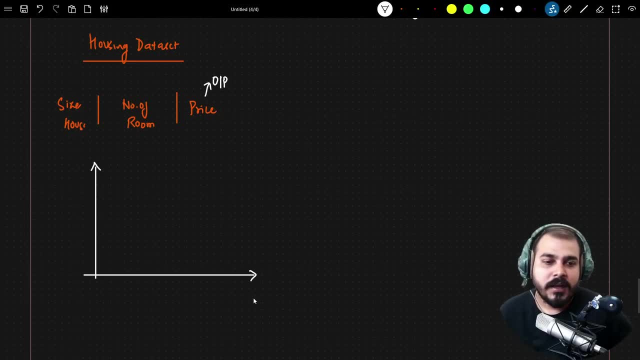 So let's go ahead and plot some data points over here And let's say: this is my size of the house and this is basically my number of rooms. Now let's say that I have some data points, which looks like this: Right, 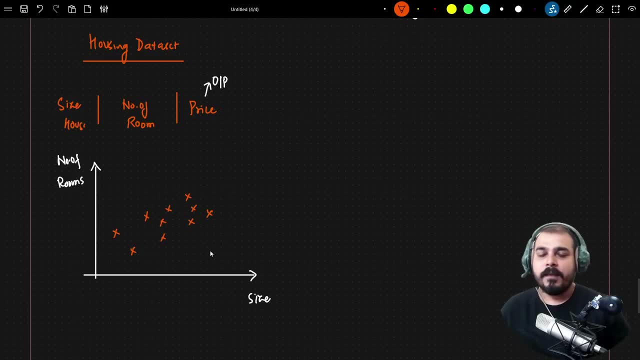 Let's say, I have some data points which looks clearly like this: Okay, Now, in this particular case, you can see that from this you are able to find out when the size of the house increases, the number of rooms are also basically increasing. 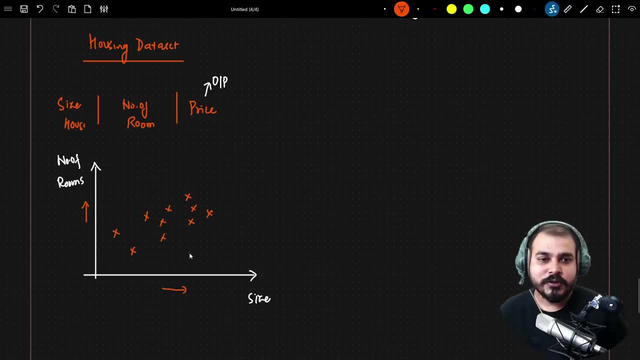 And obviously it is a common sense question- It really needs to increase. When the size of the house increases, you can assume that, yes, the number of rooms is also going to increase. Now let's consider that with the help of PCA. 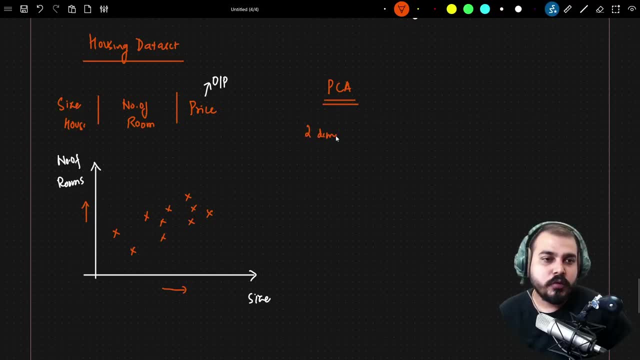 Okay, I want to reduce this two dimension of features into one dimension. Okay, Into one dimension. Now, if I want to perform this, that basically means I just want to convert this two dimension into one dimension. Okay, This is what I am actually looking, with the help of PCA. 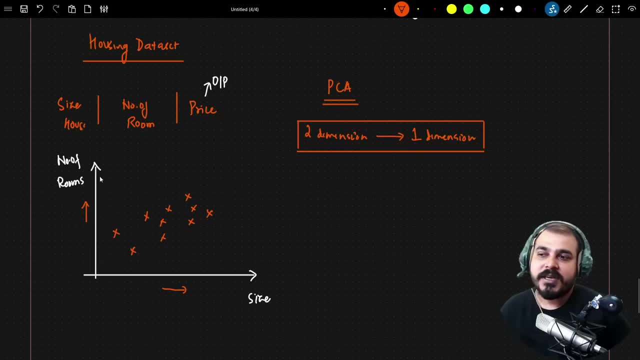 That basically means, instead of having two independent features, I just need to have one independent feature and try to basically create that independent feature. Try to find out this one dimension or independent feature. Now, in this particular scenario, let's say that one way. obviously, I have already taught you. 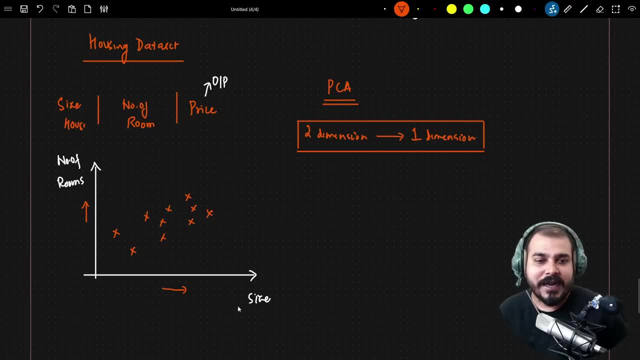 Right In feature selection. In feature selection, what you can do- you can take either one of the feature and you can ignore the other feature, And a simple way of converting a two dimension into one dimension is that. what I will do over here is that I will make sure that I will plot all this point in my x-axis. 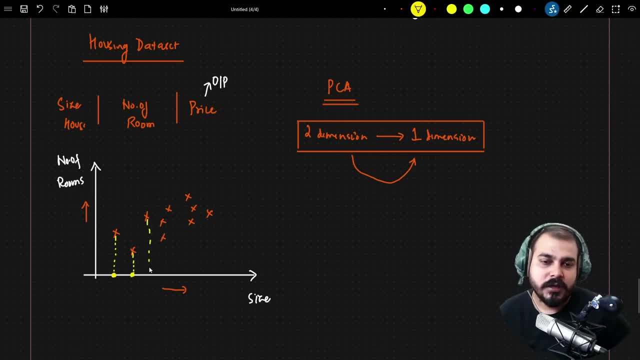 Let's say, I am just going to project all this point in my x-axis. So here you will be able to see: here I am getting the point, Here I am getting the point, Here I am getting the point Right. So once I do this, you will be able to see that I will be able to project all the points over here. 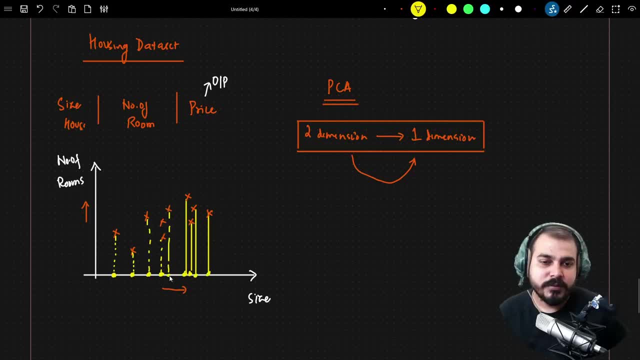 Now, when I project all the points, obviously I am able to get all my data points in one dimension. So this data points that you will be seeing, we are able to get it in one dimension. So here what I have done: I have basically converted this into from 2D to 1D. 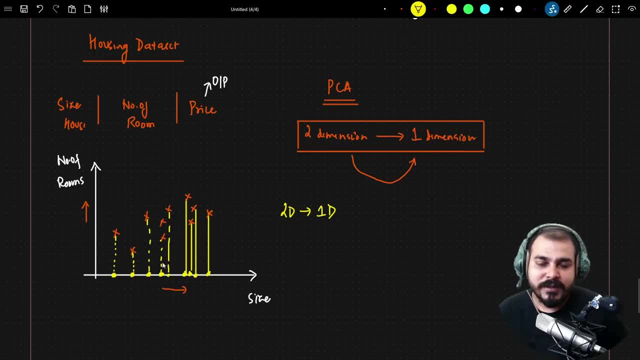 Right, And one more thing with respect to this specific data points which is super important to understand in PCA is that if I probably see the first data point here, the first data point, and the last data point, the area between this is basically my spread of the data points. 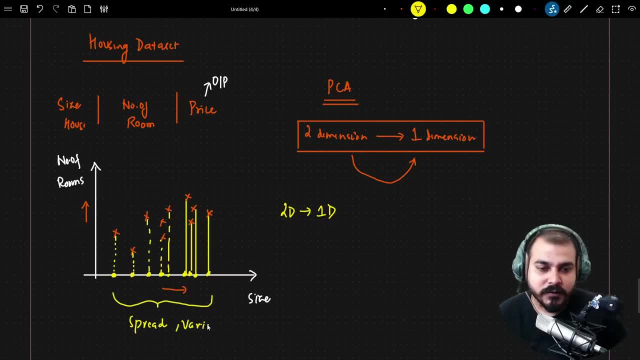 Now, if my spread is huge, then what will happen? My variance will also increase. My variance will also increase. If my spread is increasing, my variance will also increase. Okay, So this is. both are directly proportional to each other. Now what is the disadvantage by using this approach, where I am directly projecting in my x-axis? 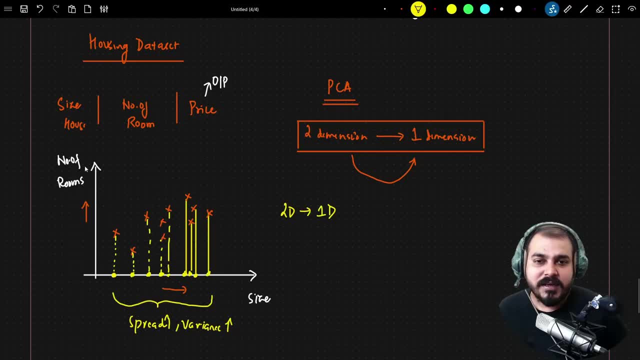 So here, obviously, the size information is getting captured, But the number of rooms information is getting lost. So this information that you had related to number of rooms, Why this information is getting lost? Because understand over here, If I try to project from here to the first point also. 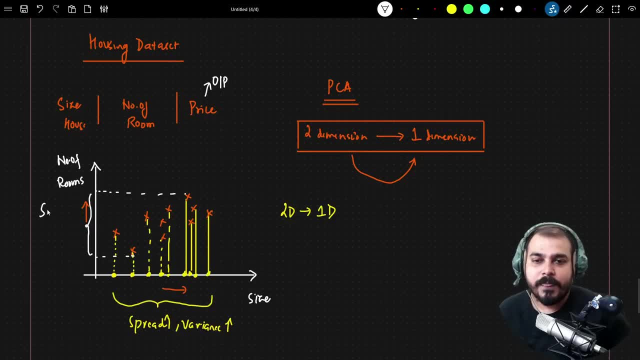 Right. Here also, you have some amount of spread. Now, as I said, if the spread is increasing, the variance is also increasing And over here because of this variance, here also some information regarding number of rooms are there Right, And you are directly skipping this information. 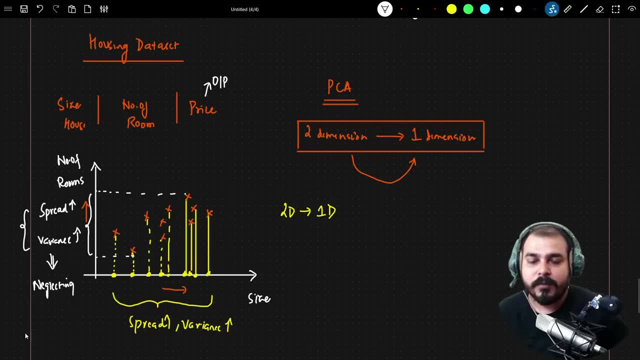 You are neglecting this information when you use this specific approach, Right, Where in you are directly projecting into one axis. So here, with this approach, what is the major thing that is happening? There is loss of information, Right, And in this case you are losing the information about the number of rooms. 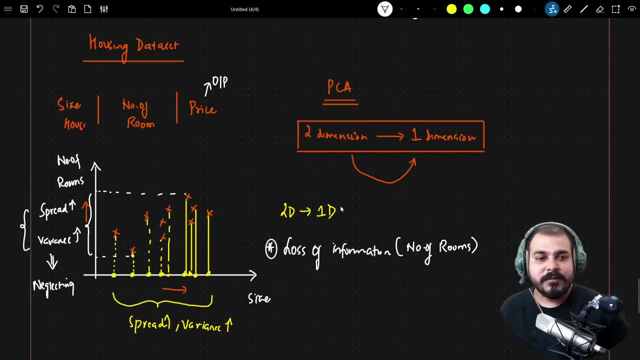 Obviously, you created from a two dimension, you created a one dimension And this is all your one dimension point. But from this, when you converted from this 2D to 1D, you are losing much information from the number of rooms, Right. 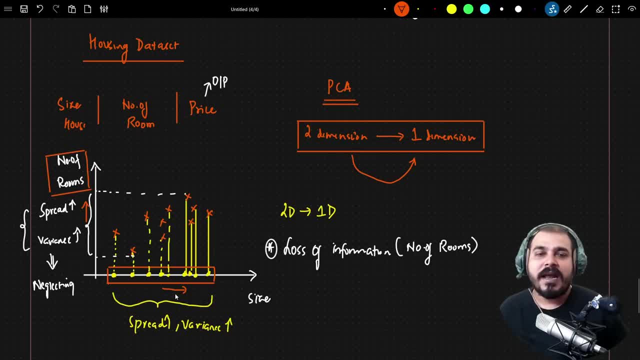 About one specific feature. Now, because of this, what will happen? you, once you lose all this information, You know your model may not perform well with respect to this specific predictions. So here, in short, you are doing feature extraction, But you are doing feature extraction with lot of information that are lost. 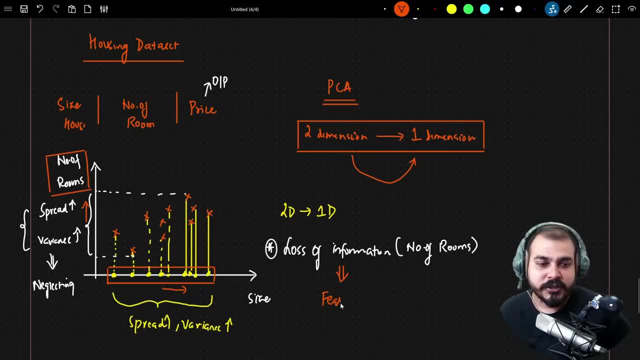 Right, So this in this feature extraction, So this in this feature extraction process, you are losing lot amount of information, Right? So I hope you have got this specific idea Now. you also have to take care when you do this kind of feature extraction. 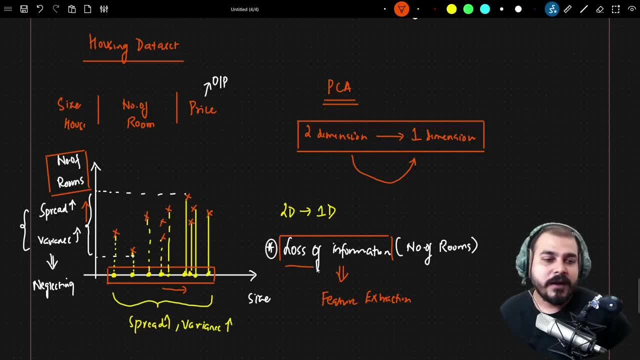 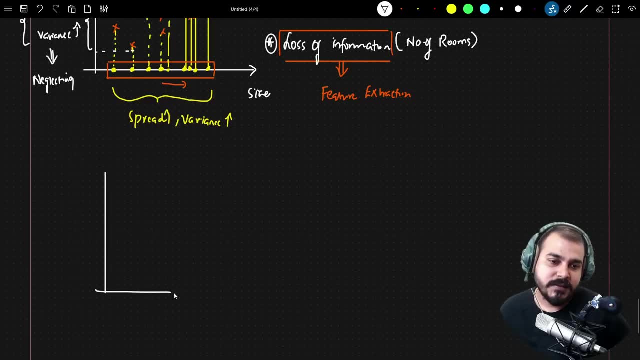 This information need not be lost that much, So how do you prevent it? So, in PCA, to give you a brief idea, let me draw this particular diagram again. Let's say if this is my size And this is my Number of rooms. 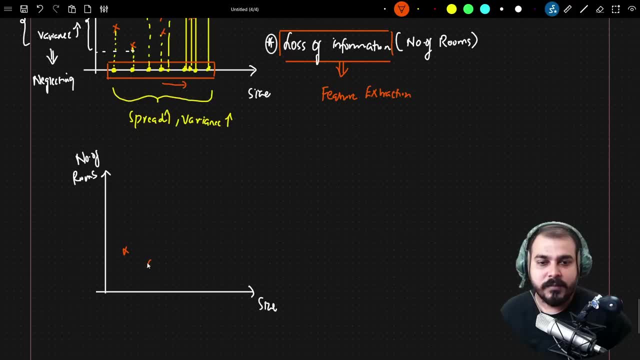 And let's say: these are my data points over here. Let's say: these are my data points over here. Now, in PCA, what you do is that You do some kind of transformation on this axis, On this X axis and Y axis. What kind of transformation? 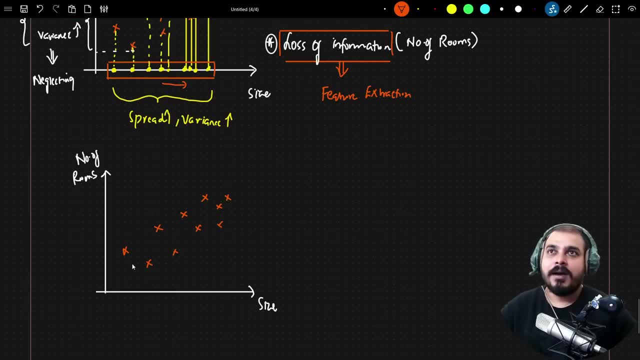 You apply some mathematical equation. I will again not talk about that mathematical equation right now, But I will just name it. You apply something called as Eigen decomposition- Eigen decomposition on some matrix, On some matrix. Okay, we will discuss about this, what exactly this is. 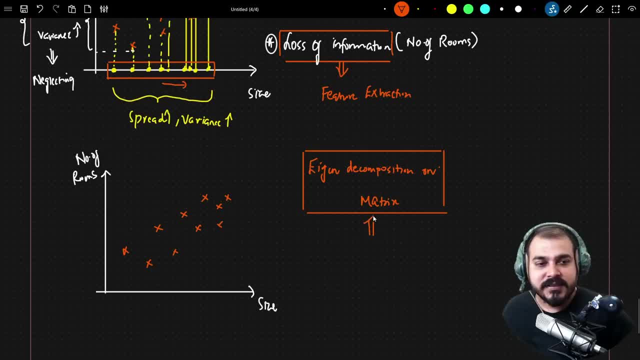 But, in short, you are going to apply some transformation And this is this specific transformation And, with the help of this specific transformation, You will be getting a new axis Which will look like this. Let's say, This will be a new axis. 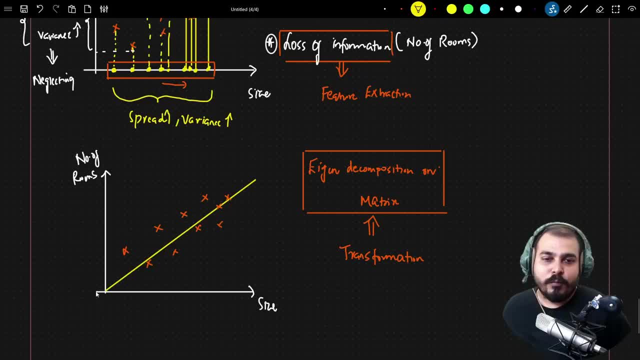 Which will look like this: Okay, And once you get this specific axis, What will happen is that Then you will try to project this information over here. You will try to project all this information over here. Now, when you try to project this specific information, 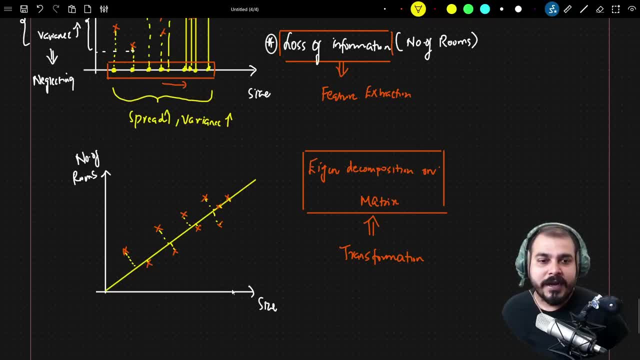 Okay, Now suppose, since you have two features, You will try to apply some transformation Which will change this size axis To some other axis, like size dash, And one more axis will get created. Let's say the other axis will be exactly perpendicular to this axis. 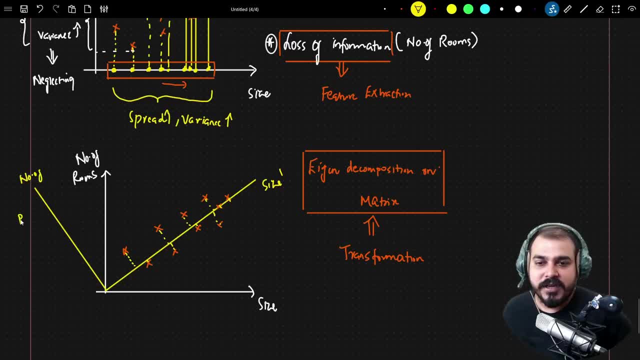 Okay, And this will be your number of rooms dash- Number of room dash- And then you will be projecting all these points over here. So, when you project all these points over here, Here are your data points Now in this projection and in this projection. 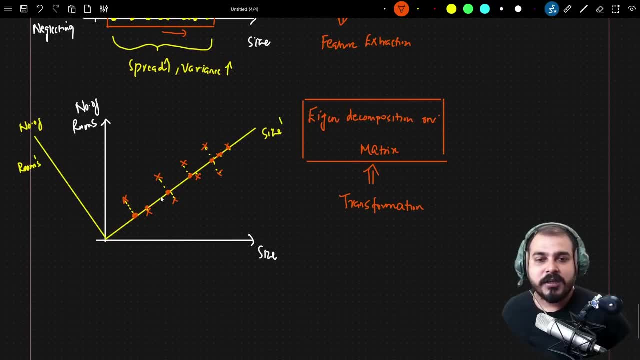 What are the differences In the previous projection and in this projection? What are the differences Now? see In the x axis. If I consider this as my new x axis, Here you will be able to see that The spread is properly captured. 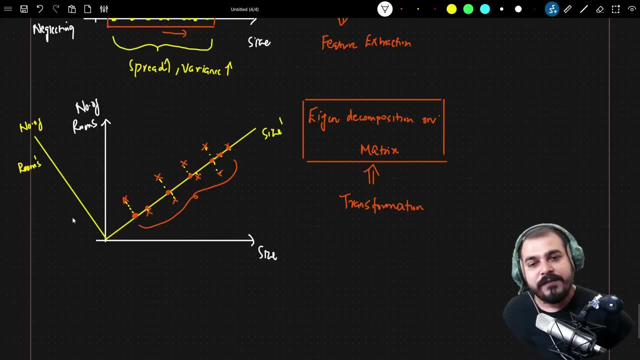 With respect to this specific points And similarly, if I try to plot all this point on this new axis, Here you will be able to see your spread That is going to get lost Once we project over here Will be very, very less. 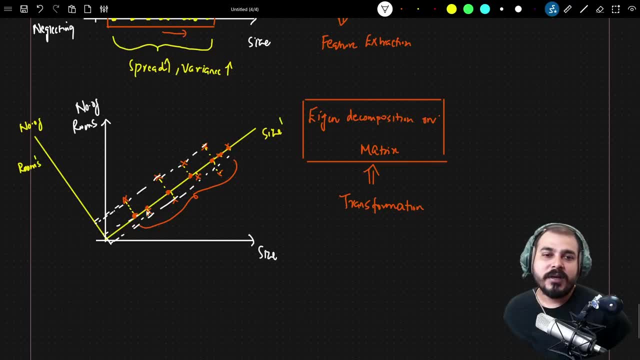 Will be very, very less. So here what you are doing is that You are applying some transformation And you are creating a new axis Like this: size dash And number of room dash. And once you create this new axis, All you do is that you now 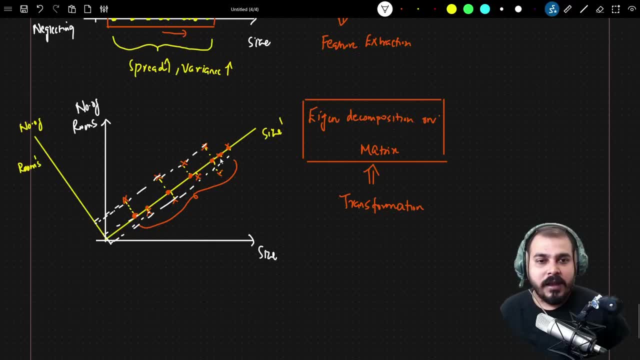 Just project all this point to this particular axis And after projecting this point, You can see that maximum variance is getting captured For all the points over here. So here, maximum variance is getting captured. Maximum variance is getting captured. And why this is better than this. 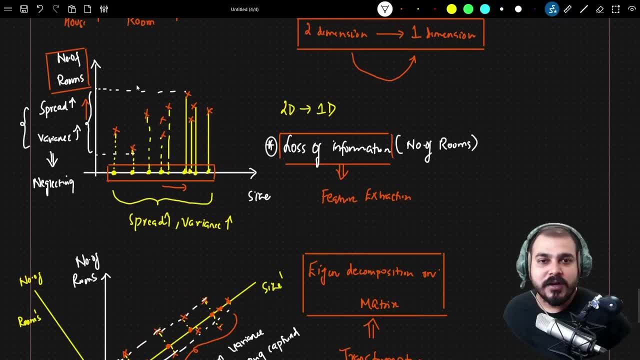 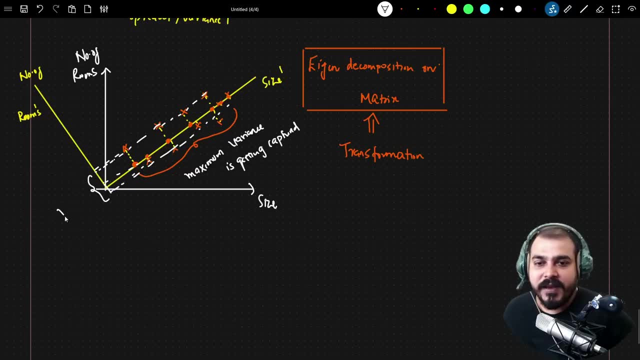 Because in the y axis, You are not losing much information. You are just losing this amount of information, Right? This amount of variance You are basically losing, Right, When you project it on the x axis. Now, with this transformation, You are able to convert your two dimension into one dimension. 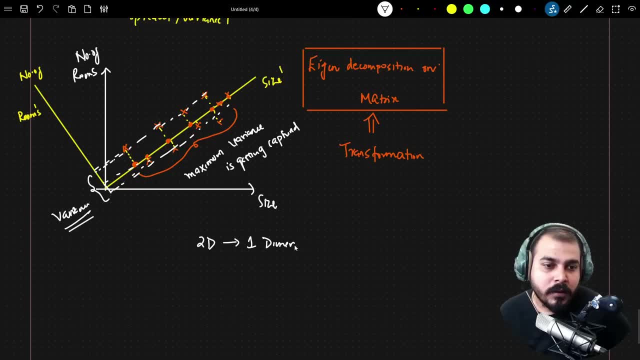 And you are making sure that You are not losing any information And you are making sure that Much information is not lost. Much information is not lost. And how do you, How do you come up with this specific point? Because, see in the y axis- 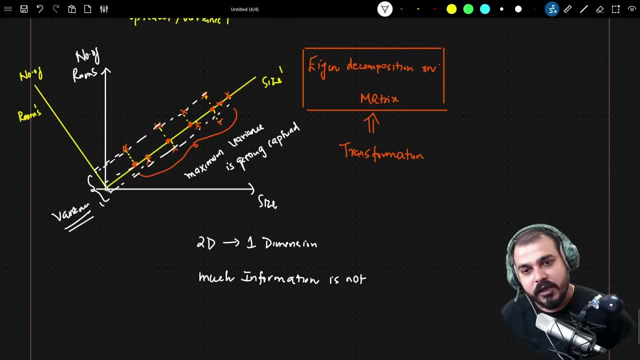 Because of this new dimension Here the variance is less Right. So even though you project this point over here, Most of the variance is basically getting captured by your x axis, So much information is not lost If you compare the previous example here. 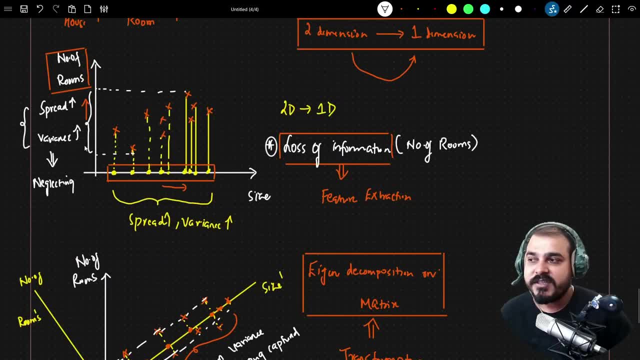 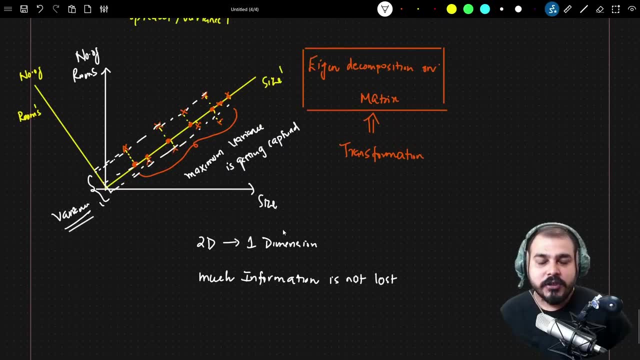 Once you project it into the x axis, Huge amount of information is getting lost, Because here the variance is quite high Or spread is quite high. Here it is not that high, Right? So I hope you have understood. Our main aim in PCA is that. 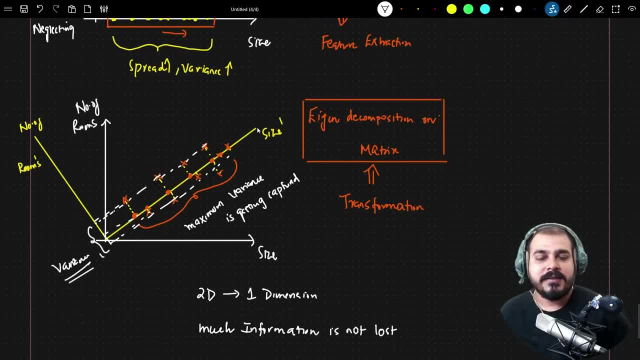 To find out this kind of lines Right. So after transformation, Which is the new axis that is basically getting created Now, since I just had two dimensions, So after I do the transformation, I basically call this as Principal component analysis. one: 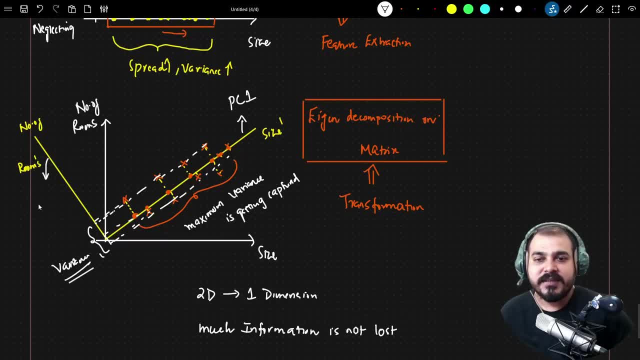 So PCA one, Principal component one And we basically say this as principal component. two: Suppose if you have three dimension, That basically means You will be having Three principal components. Always remember: PC one Will be capturing the maximum amount of variance. 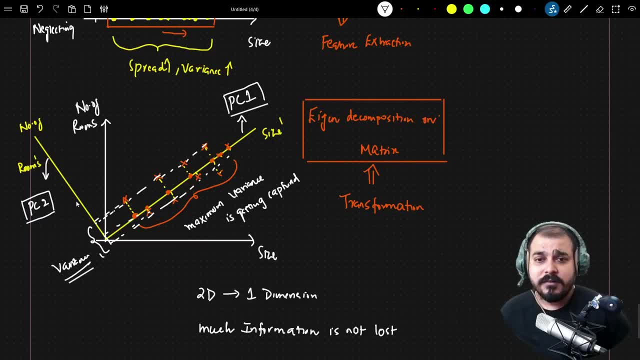 And then PC two will be capturing The next maximum amount of variance. Similarly, If you have three dimension, Then PC three will be capturing The maximum amount of variation after PC one. Sorry, maximum amount of variance after PC one And PC two. 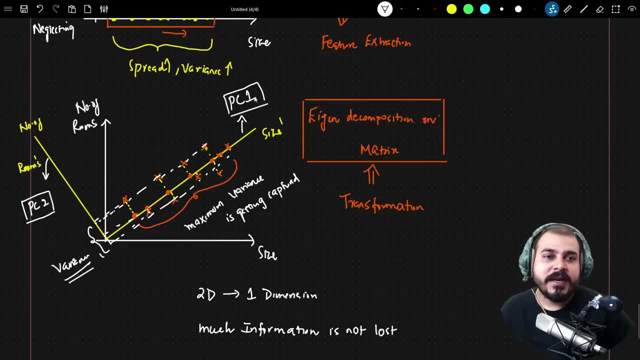 Right. So over here In geometric intuition behind PCA, Our main aim is to basically find out principal components, Right, Like how we find out this, And at the end of the day, We really need to find out one Line That should be able to capture. 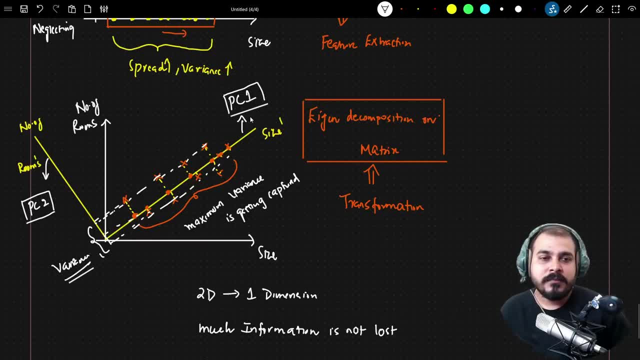 The maximum amount of variance And once we take this PC one And then we can convert this into a From a two dimension. We will just be taking up this specific point Until finally get converted into a one dimension point, Right, So I hope you got an idea about. 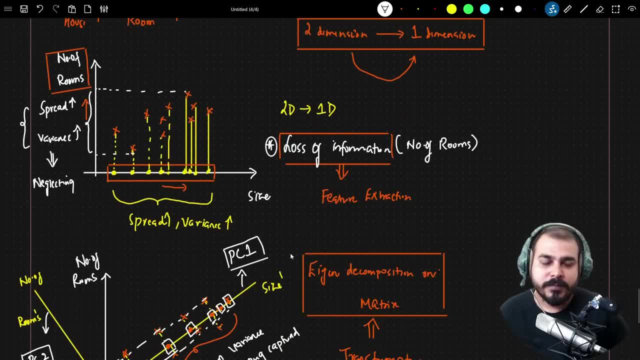 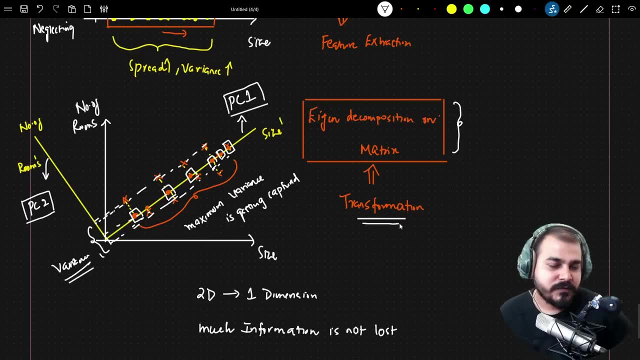 What is the geometric intuition behind PCA? PCA, that is principal component analysis. We'll talk more about what is eigen decomposition on matrix And what is this specific transformation With examples. I'll try to show you, But just understand that Your main aim is to find out. 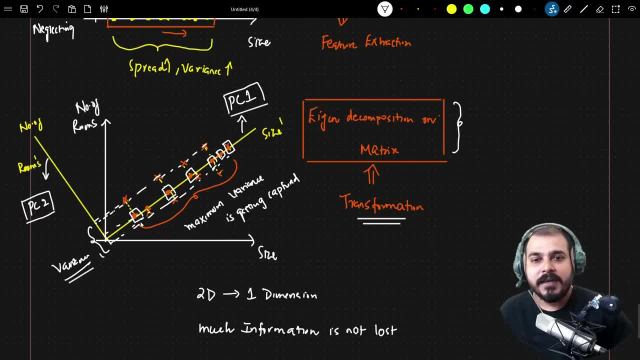 The principal component Which has, After projecting all the points, It should have, captured the maximum variance Or spread. Okay, And why variance is important? Because variance basically talks about The data, How the data is basically spread And, with the help of variance, 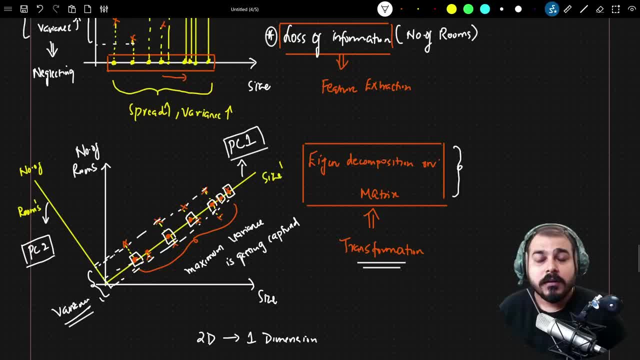 You'll be able to capture more and more information. So, guys, The final goal Of a PCA algorithm will be that To find out the principal components In such a way that maximum variance will be captured. So suppose, if I have Two dimension points, 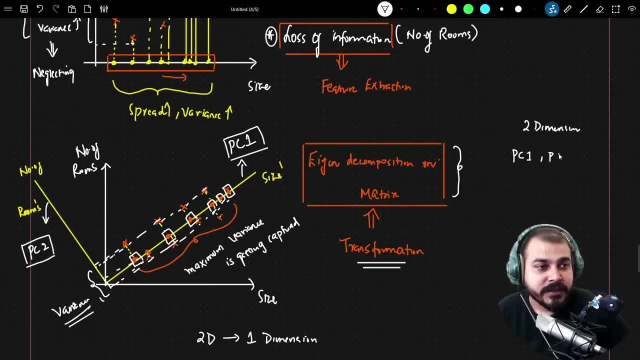 Then I will basically be having PC1. Then PC2.. Right, And we know that The variance with respect to PC1. After we, You know, project all the points in that particular component Will be greater than The variance with respect to the principal component 2.. 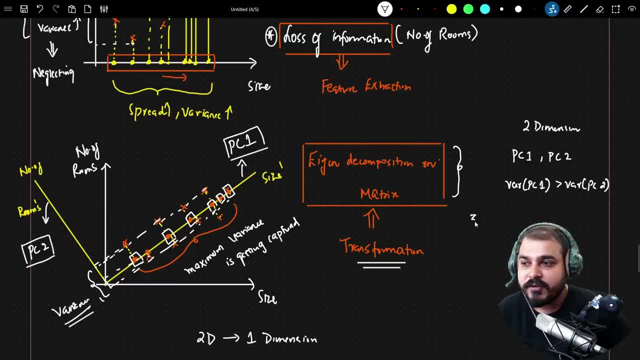 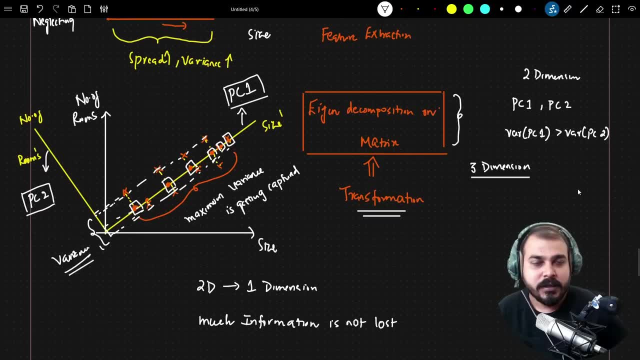 Once we project it. Suppose, If we have specifically three dimensions, Then here You'll be able to see that We will be getting three principal components. Okay, That basically means like We'll be having three different axis. One is PC1.. 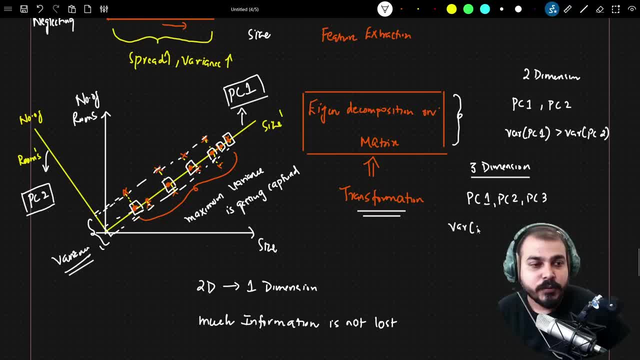 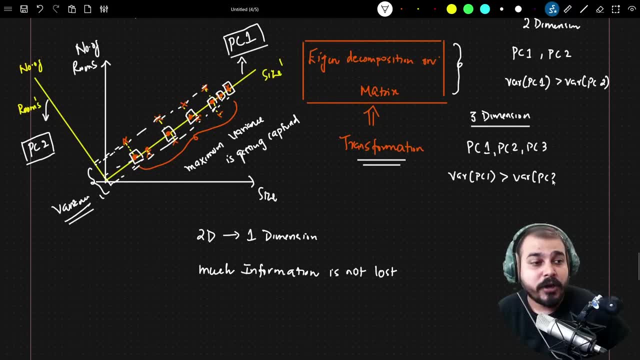 PC2.. PC3. And obviously the variance with respect to PC1. Will be greater than The variance with respect to PC2.. After we project the points And the variance With greater than PC3.. Okay, So this variance will be following this specific approach. 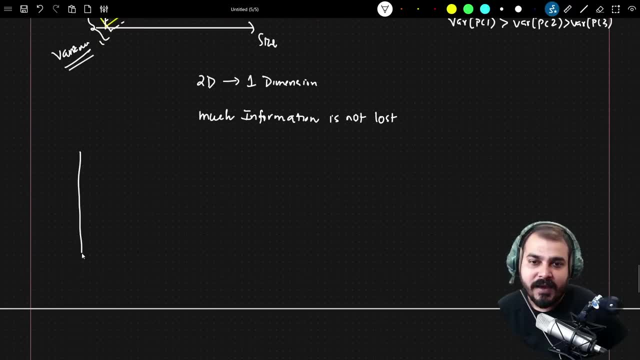 So Let's say That If I have A task Wherein I have two dimension points, Which is like this, And let's say I want to convert this 2D To 1D, So at the end of the day, 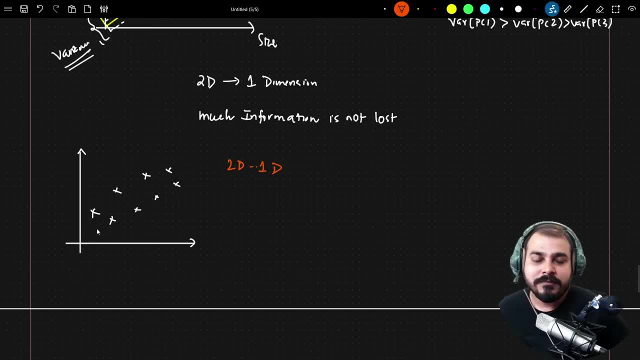 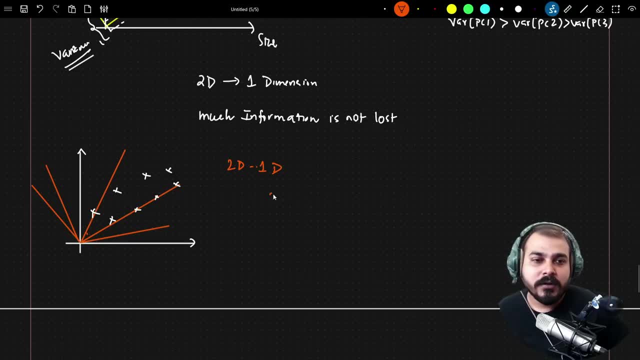 It can be this line, You know, And it will try to select The two Best Principal component lines, Principal component lines And how we say that This is the best principal components line, Because Once we project, Let's say 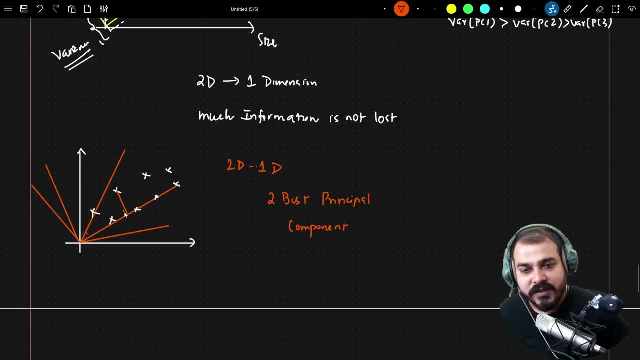 Once we project This specific points On this line Right, We will be able to call This line As the best line Only when The variance That is getting Captured As maximum Okay. So let's say: 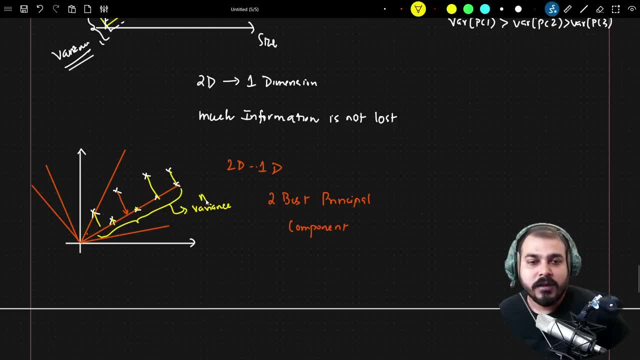 This line Has actually captured The maximum variance, So I will say This as PC1.. Suppose, If this line Has captured The second Maximum variance, Then I will basically Say It as PC2.. So 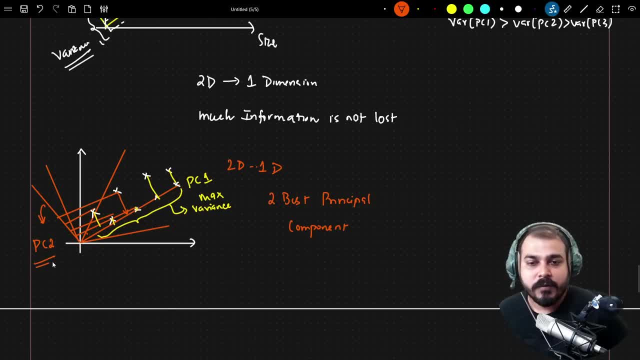 So this specific line Will be my PC2.. Right, And At the end of the day, If I am converting This into 2D To 1D, Then what will happen? I will basically Be taking up. 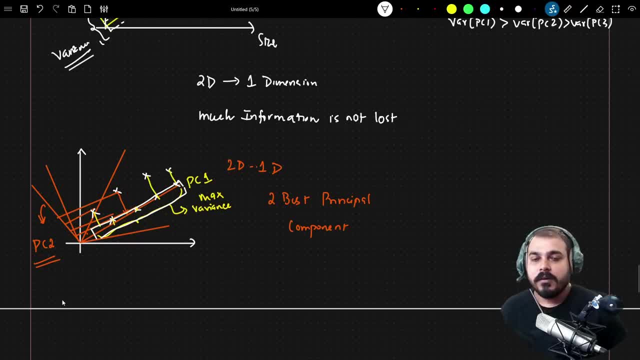 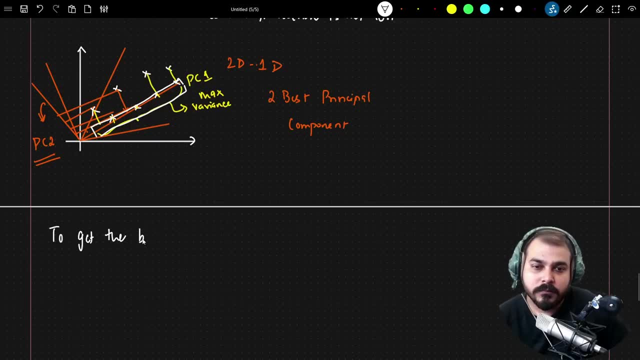 The specific points That I have actually Plotted over here. Okay, So, guys, The final goal Will basically be To Get The Best Principal Component. And how do we say That It is the best? 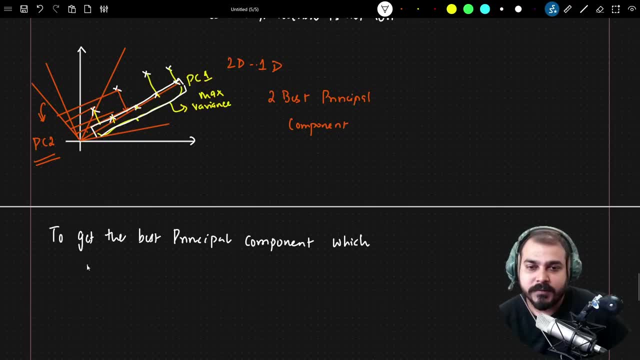 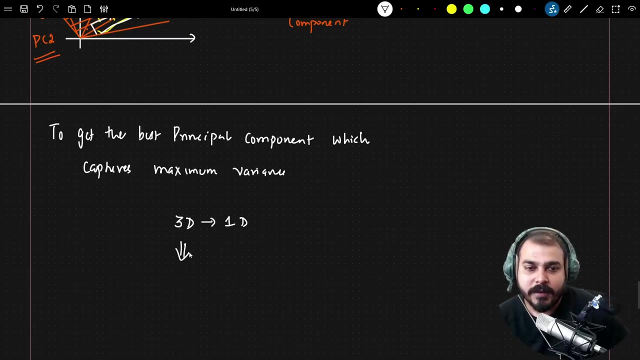 Principal component Which captures Maximum variance. Right, Which captures Maximum variance. Okay, Now Let's say That If I want to Convert A 3D Point To 1D, Now, 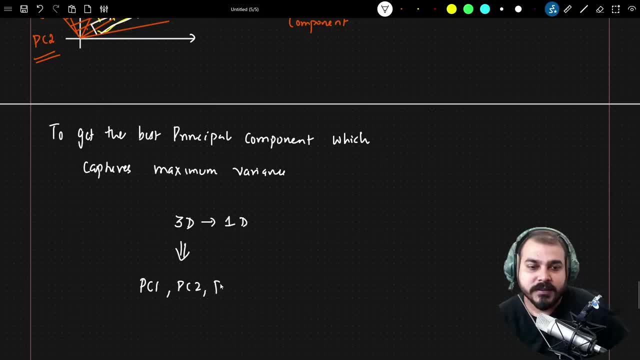 In the case of 3D Points, You know We will be getting 3 components. One is PC1., PC2. And PC3.. Right, And Obviously It can be All these 3 lines. 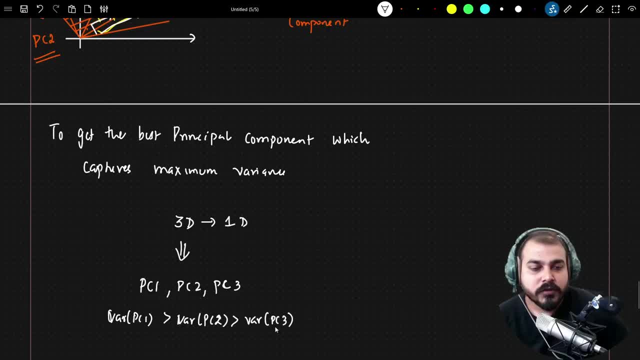 Any of the best 3 lines And you know That The variance Of PC1. Will be In PC1. And I will be taking All these points As my 1D Point Right. 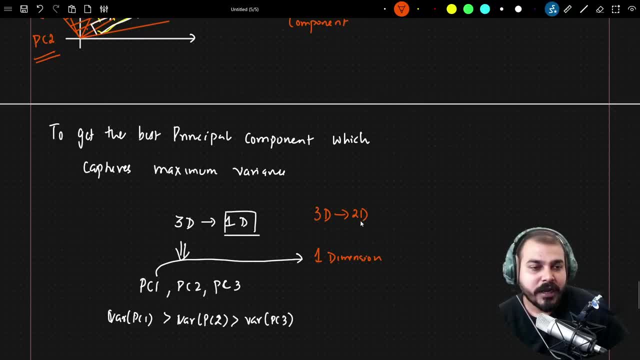 1D Point. Let's say, If I want to Convert This 3D Into 2D, Then What I'll Do, I will Probably Take PC1. And I'll 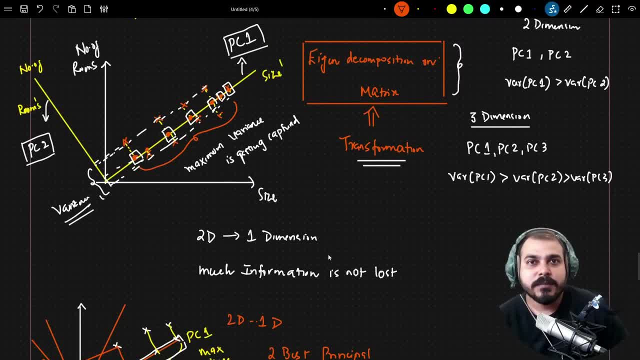 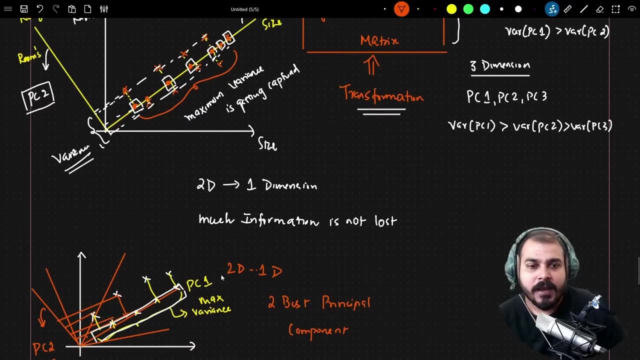 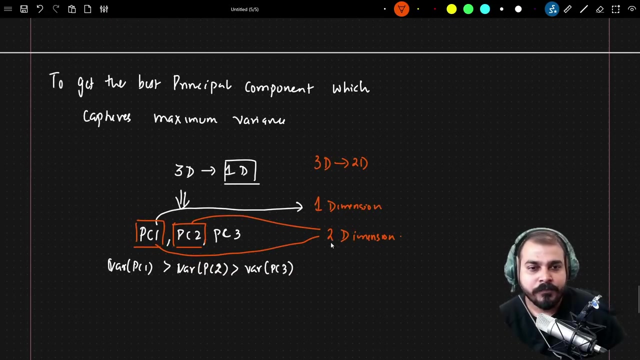 Also Make The Major And The final Aim Of The Principal Component Analysis Is To Find The Best Line After The Transformation Which Will Be Able. 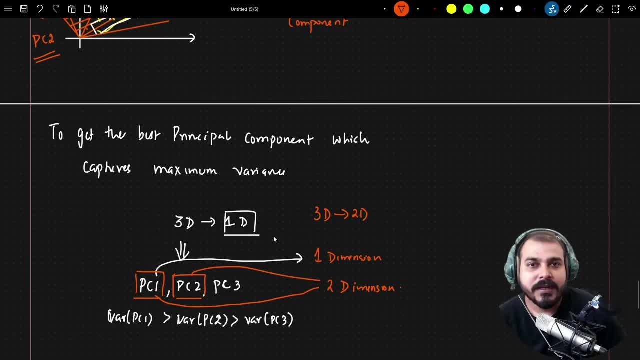 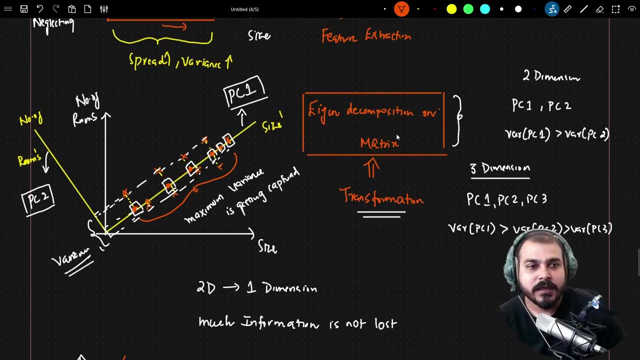 To Capture Maximum Variance, And How This Transformation Basically Happens. And That Is Where We Are Going To Learn About Eigen Decomposition On A. 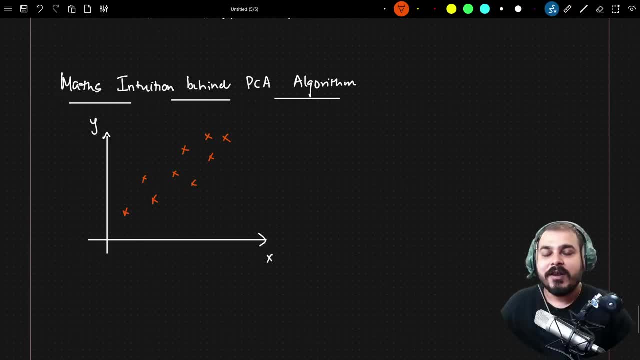 Specific Matrix. We'll Talk About All. What Are The Steps That I Have This To Access X And Y, And I've Just Plotted This. 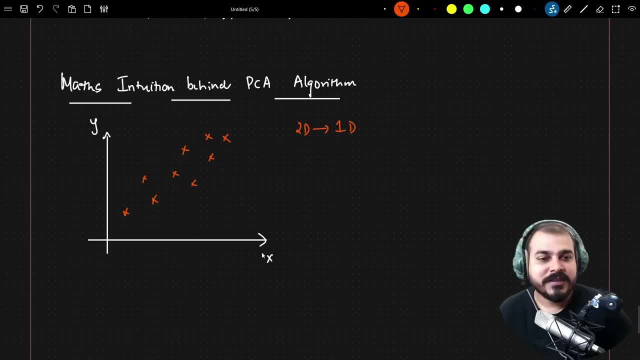 Point. And Let's Consider That My Aim Is To Convert Or Reduce From Two Dimensions, Because As Soon As I Plot All This Point Over, 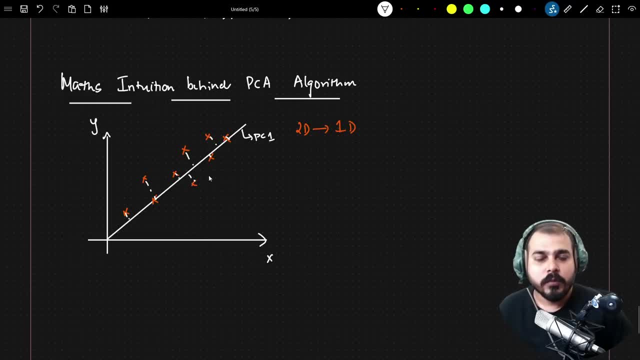 Here You Can See That Maximum Variance Will Get Captured Right. So That Is The Reason Why We Are So. Let's Go Ahead And 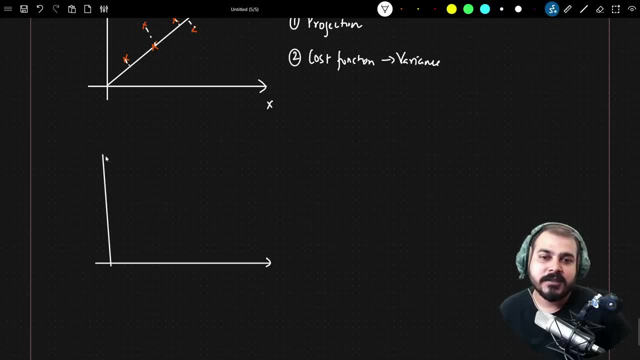 Discuss About Both Of Them, Okay. So, Out Of All These Points, Let's Do One Thing, Let's Take Up One Point, And For Now, Okay. 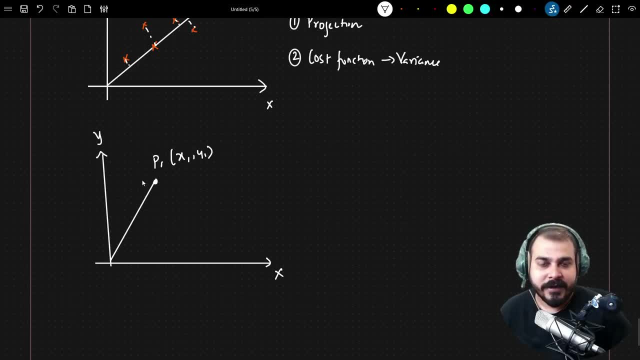 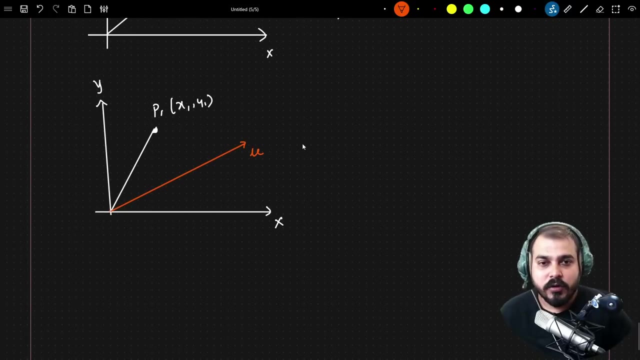 So Let's Say That This Is A Specific Vector And This P1. Is A Vector, And Let's Consider That We Also Have A Unit. 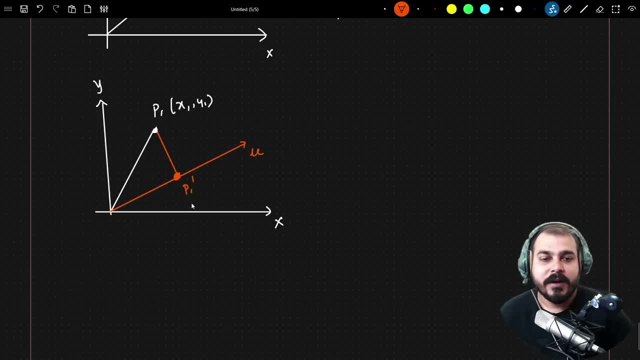 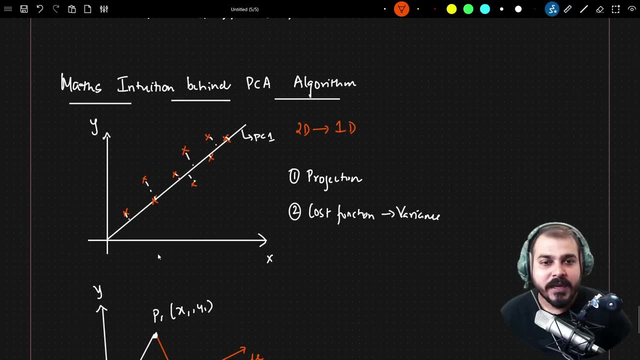 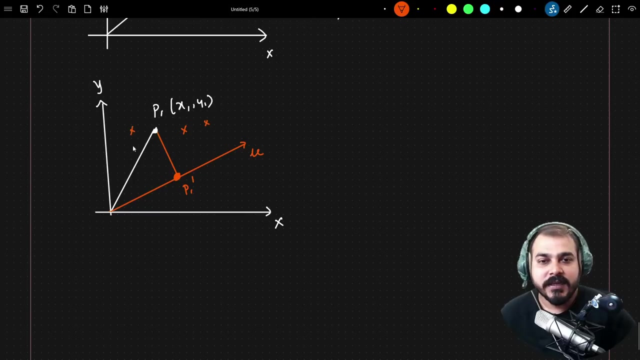 Vector, Which Is Specifically A Vector. Now We Really Need To Find Out What Is This New Projection? Because See Over Here Our Main Image To 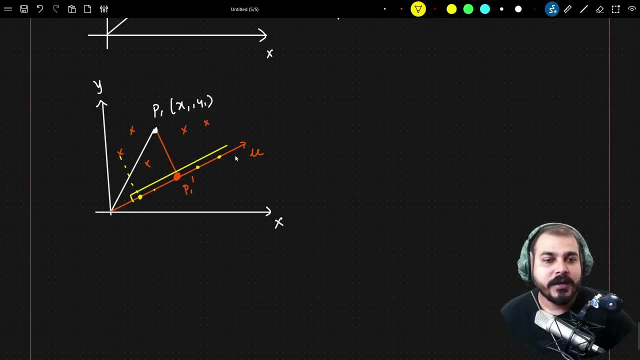 Capture The Maximum Variance, The Maximum Variance To Calculate The Variance Right. So That Is A Reason Why We Really Need To Project This. 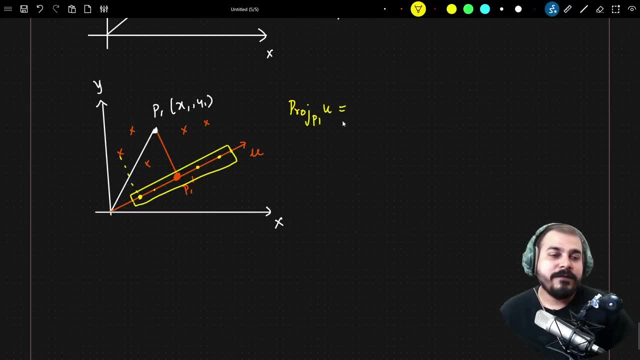 Particular Point Over Here. So Once We Project, Let's Say If We Have A P1. Vector Multiplied By U, Vector Divided By Magnitude, 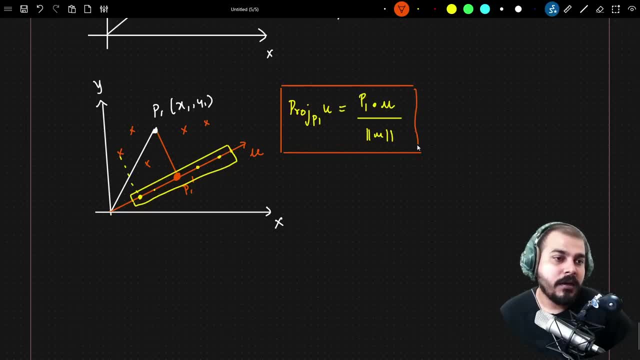 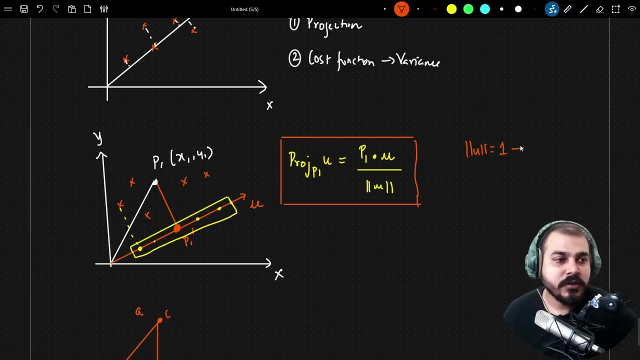 Of U. Okay, So This Is The Equation That Is Basically Used With Respect To The Projection Of P1.. On. U Is Equal To Nothing. 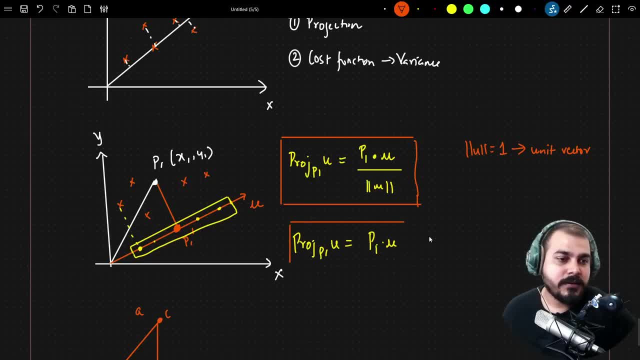 But Dot Product Of P1. Multiplied By U. So This Is The Entire Thing That We Basically Get, So As Soon As Nothing But This. 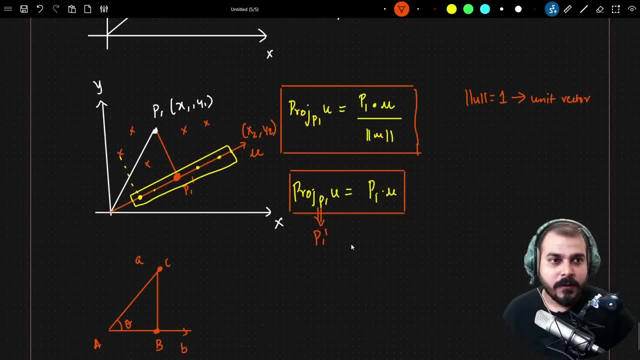 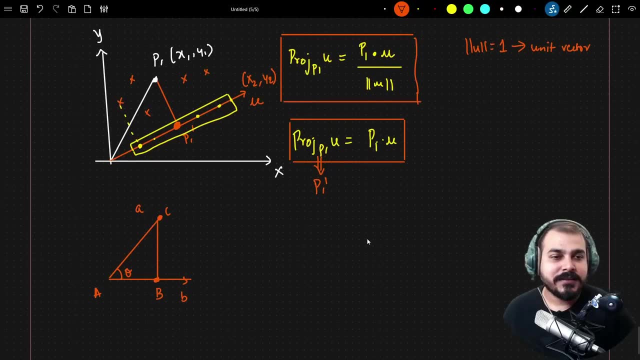 Is P1. Dash. Now, This Is With Respect To The Projection Which Everybody Needs To Understand. Okay, Now Let's Go Towards Understanding Like This: When 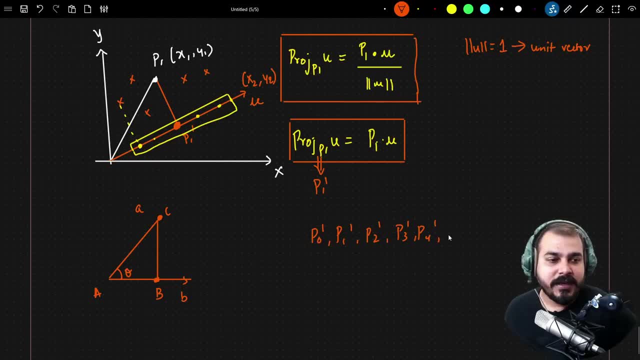 We Project It, Let's Say P0. Dash, Like This: We Have More, All The Points, And We Get Finally Pn Dash. Now, Once We 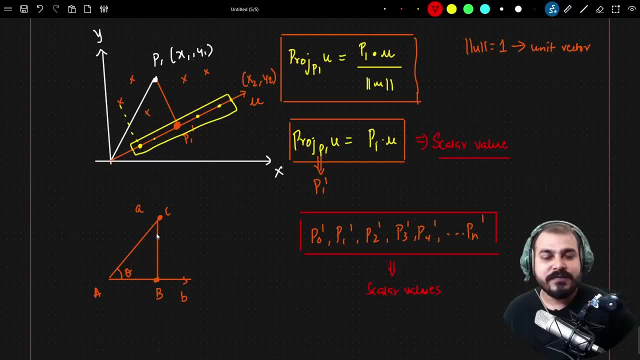 Have All These Points And Remember What Is P1. Dash Basically Talking About. It Is Just Talking About The Distance From Here To This Particular. 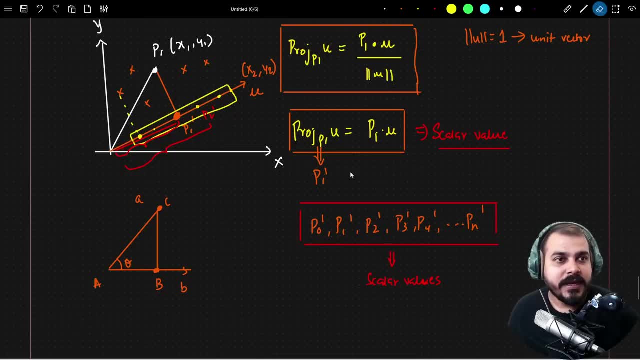 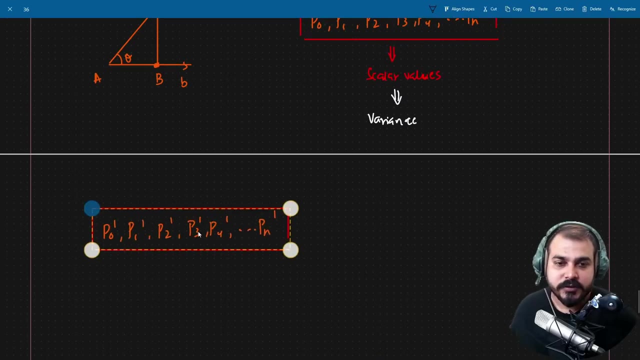 Axis, Right? So Let's Say, If I'm Probably Calculating Distance, So I'm Just Going To Select All These Things. Okay, And These Are My. 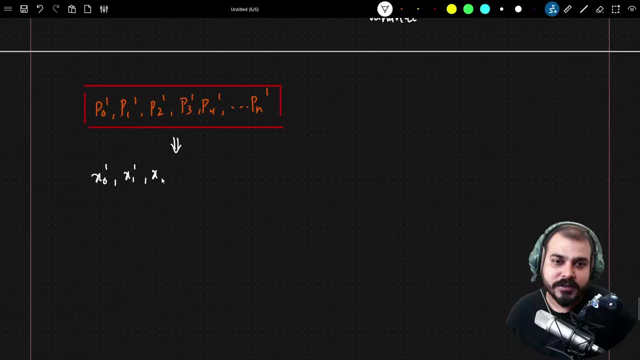 Points P0. Dash, P1. Dash, P2. Dash, P3. Dash. So Let's Say I'm Talking About The Distance From Here To The Distance From. 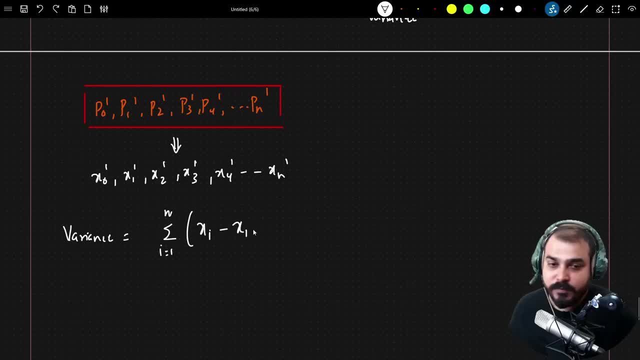 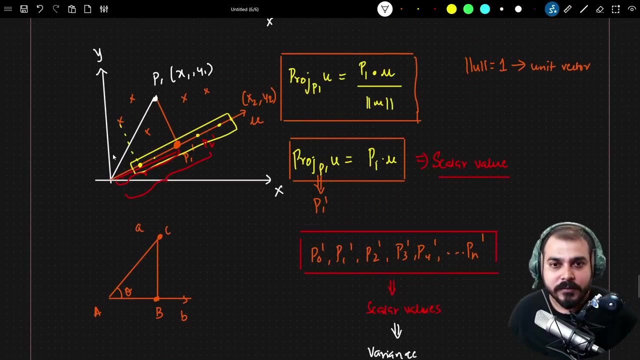 The Distance: P1.. Dash- P2.. Dash- P3.. Dash- P4.. P5.. Dash- P6., P7., P8., P9., P11., P12., P13., P14. 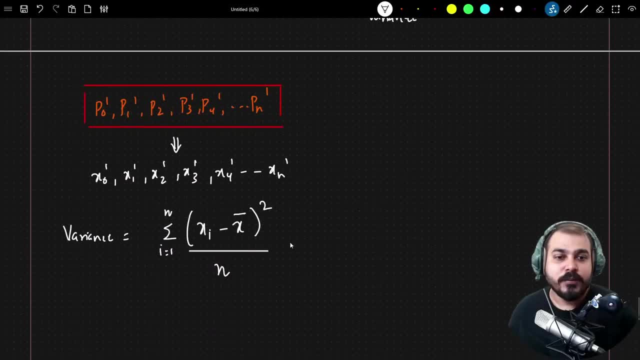 P15., P16., P17., P18., P19., P20., P21., P22., P23., P24., P25., P26., P27., P28., P29., P30., P31. P32., P33., P34., P35., P36., P37., P38., P39., P40., P42., P44., P45., P46., P47., P49., P50., P51. 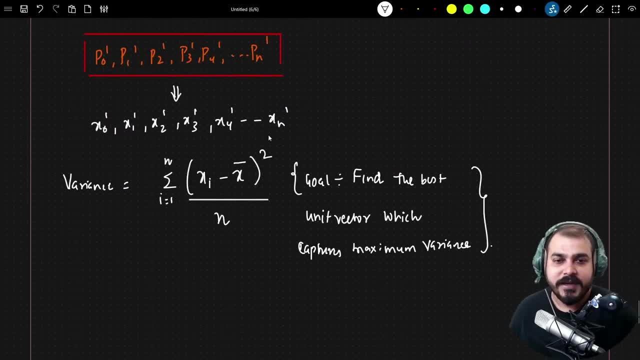 P52., P53., P54., P55., P56., P57., P58., P59., P60., P61., P62., P63., P54., P56., P57., P58., P59. 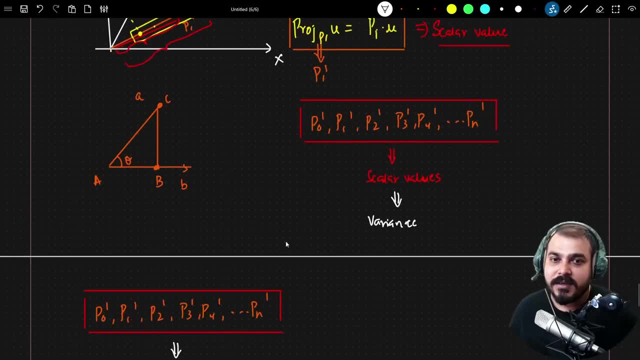 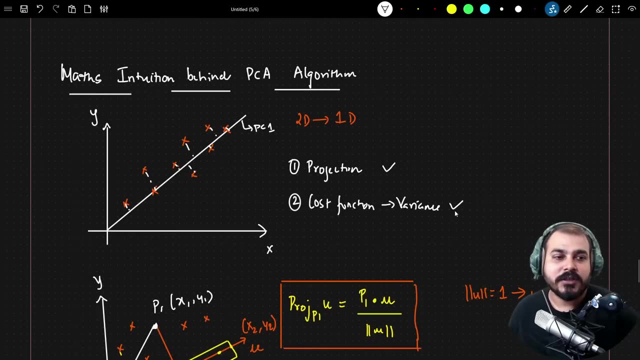 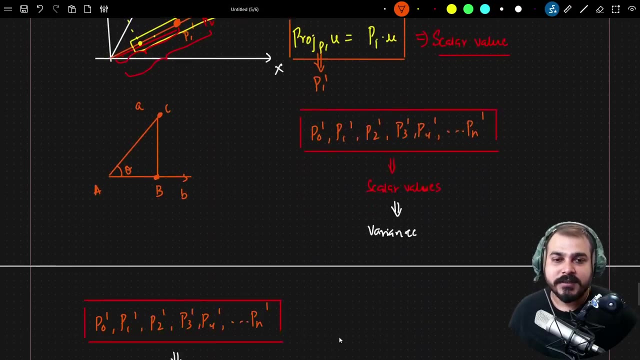 P60., P61., P62., P63., P64., P65., P67., P68., P69., P71., P兩, P52., P53., P52. P investir, P54., P55. 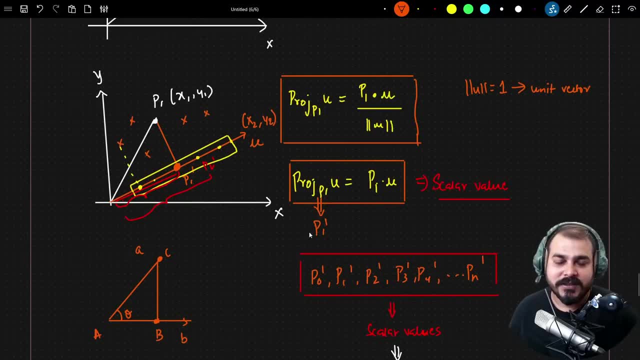 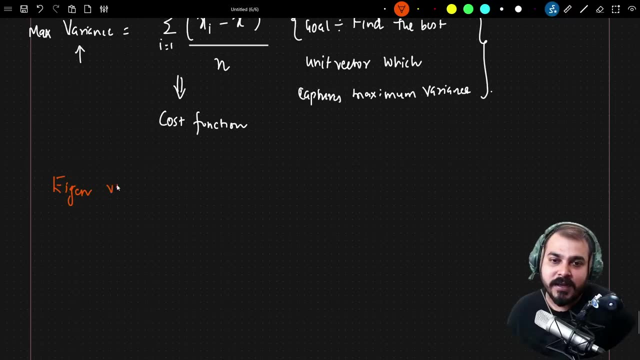 P66., P57., P78., P59., P Gab scan. P58., P95., P30., P41., 12., 11., 12., 13., wishing 12.. okay this, eigenvectors and eigenvalues, because our main aim isn't, as said, right, we really need. 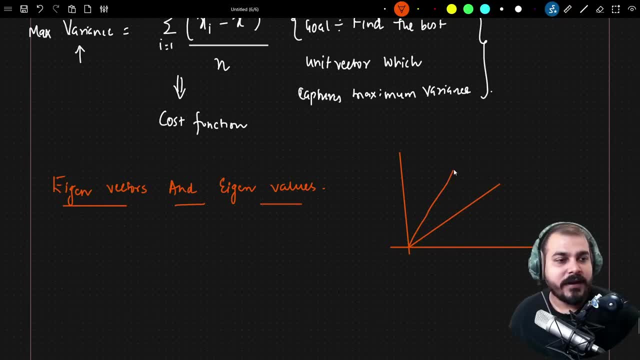 to find out the unit vector, right, whether the unit vector should be this, this or this, or this or this, right? so how do i find out which unit vector we should basically select to capture the maximum variance? so for that we will be using something called as eigenvectors and eigenvalues. 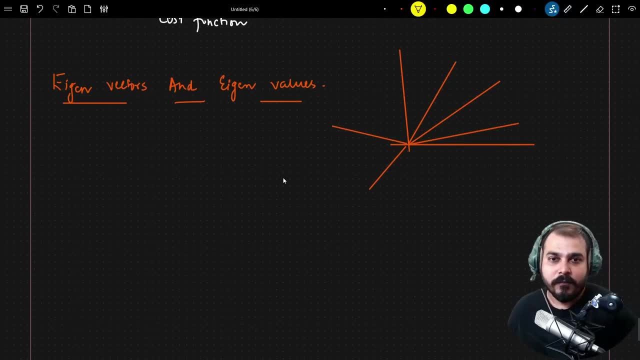 and there are some steps right, that are steps which are involved in this. first of all, the first step will be that i really need to find out the covariance matrix between features, between features, and in order to find out eigenvectors and eigenvalues. what i need to do is that we this. eigenvectors and eigenvalues will be. 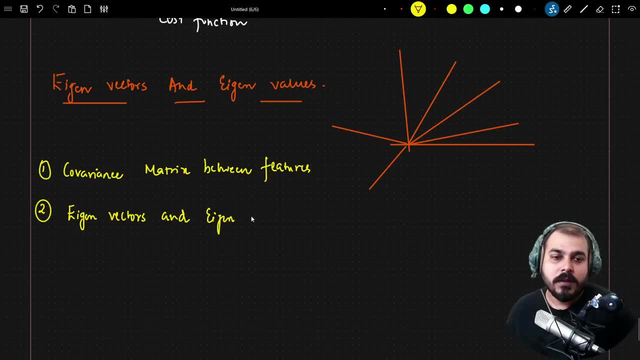 eigenvectors and eigenvalues will be computed or will be found out from this covariance matrix. how that we'll discuss about it, don't worry. and whichever eigenvector will be the largest one? when we say the eigenvector which is largest one, that basically means for the eigenvector where the eigenvalue is high, this: 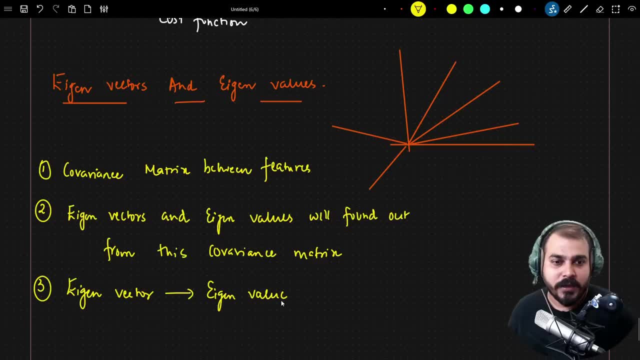 eigenvalue basically talks about the magnitude of the eigenvector. okay, so this eigenvalue is nothing, but this is basically the magnitude of the eigenvector. this will basically capture the maximum variance, capture the maximum variance and this is mathematically proved. guys, i will not be. 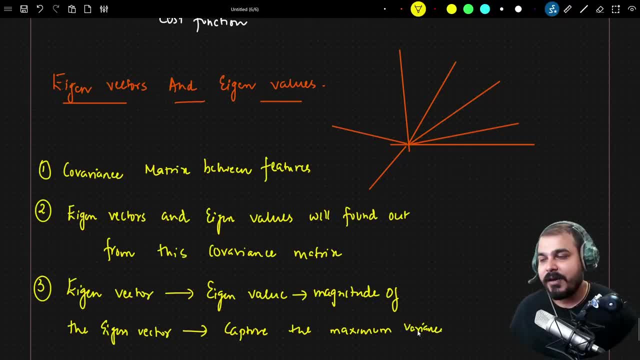 proving you this thing. but here, according to linear algebra and with some of the mathematical equation, we can definitely prove that. so, in order to? why do we compute eigenvectors and eigenvalues? because, see, at the end of the day, i really need to find out the best unit vector such that maximum variance is captured, and we cannot. 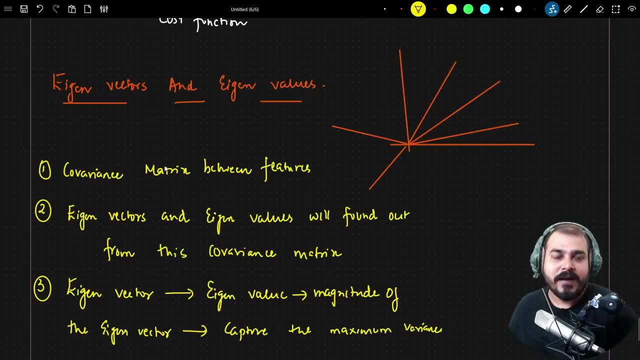 keep on doing hit and trial right. so what we do is that, in order to find out, we really need to go ahead and find out eigenvalues and eigenvectors- sorry, eigenvectors and eigenvalues- and the step is that, first of all, we will go ahead and find out the covariance matrix between the features. okay, 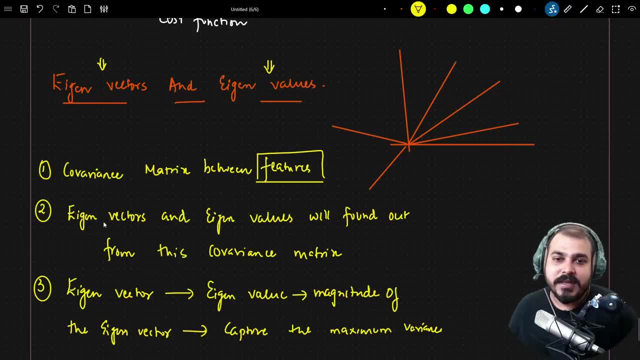 between the features. we'll go ahead and find out the covariance matrix and then we'll try to find that out. so that is eigenvectors and eigenvalues. the eigenvectors and eigenvalues can be found out by the simple equation that is: A lambda is equal to A. sorry, A vector v is equal to lambda. 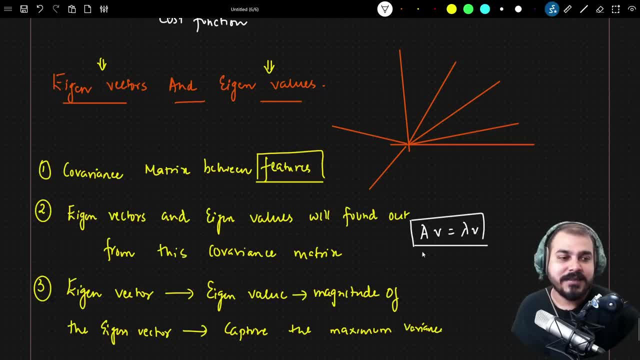 vector v. we'll try to understand this specific equation. what exactly this equation is? this is nothing but linear transformation of matrix. so we will try to understand what exactly is this linear transformation of matrix. okay, so now all of this, that is our theoretical definition, matrix. and then, once we do this, you will be able to get some eigenvalues, whichever eigenvector. 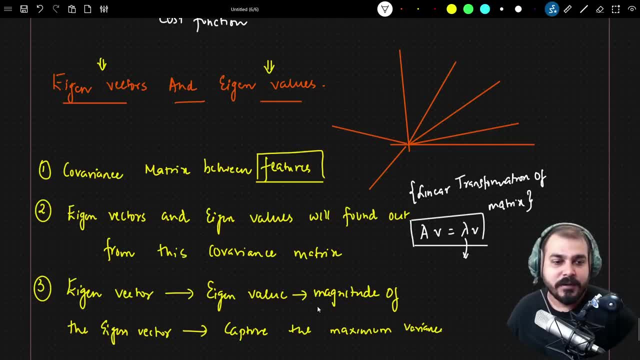 has the highest eigenvalue, which is nothing but magnitude of the eigenvector, that specific vector will get selected. if suppose this is the vector that has the highest magnitude, then this will get selected because mathematically it is proven that whenever we project on this specific line, 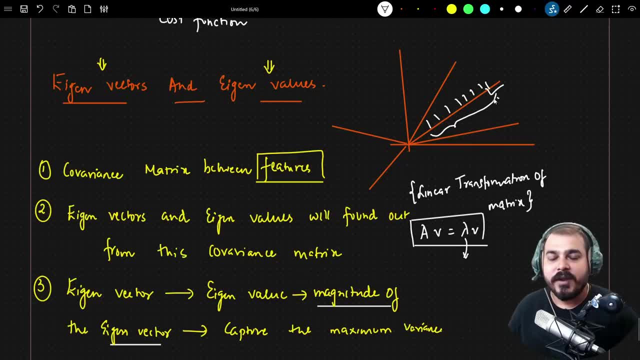 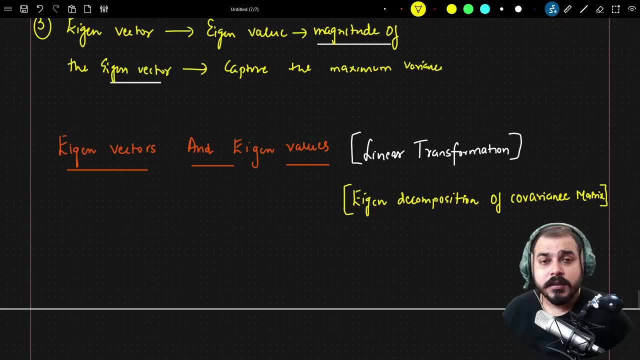 maximum variance will get captured. okay, so this is what we are going to do. in the next step, we'll understand about eigenvalues, eigenvector, eigen decomposition from a specific matrix. in this video, we are going to discuss about eigenvectors and eigenvalues now already in my 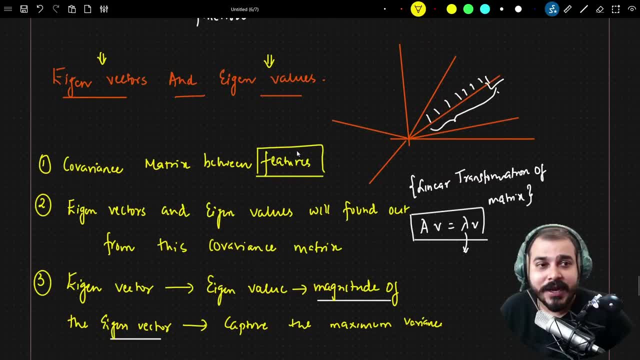 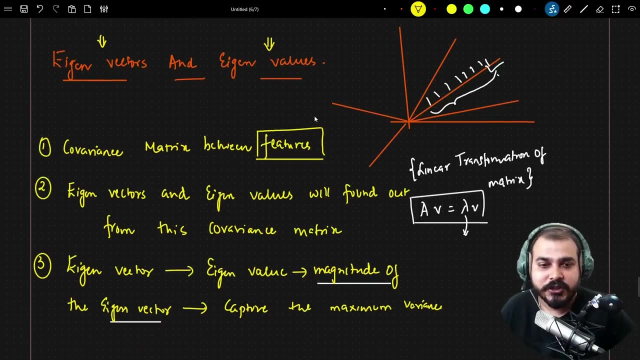 previous video i've spoken about it- what eigenvectors and eigenvalues can actually do. see, at the end of the day, we have to find the best principal component line which will be able to capture maximum variance and in order to find this, we will be using this eigenvectors and eigenvalues because, in short, whichever eigenvector, 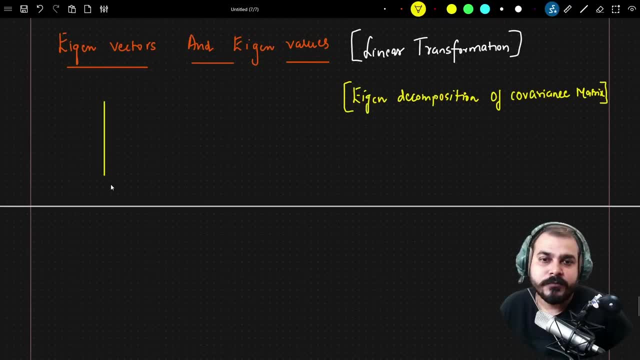 like, if suppose, let's, let's consider that we have, uh, we have some data points. let's say, i have some data points over here and this data points, let's say, i want to find out the best principal component line in such a way that once we make sure we project this right in this right in this particular 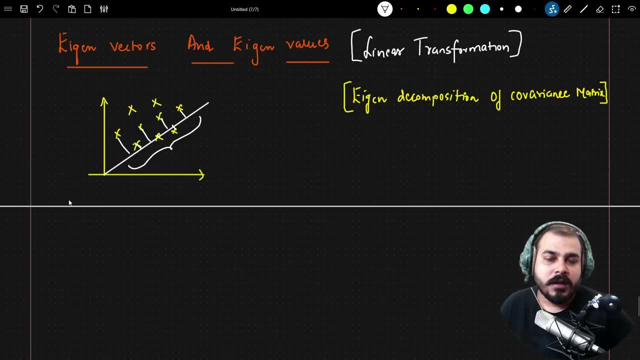 line. we should be able to capture the maximum variance. and we should be able to capture the maximum variance now. what is so amazing about this? eigenvectors and eigenvalues, and we'll also be talking about linear transformation- okay, and we also say it- as eigen decomposition of covariance. 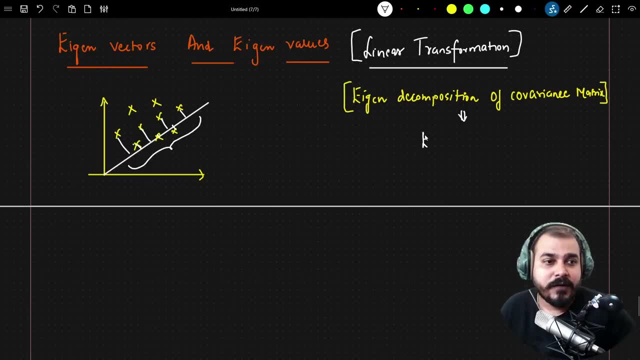 matrix. that basically means for this particular matrix. we will try to find out the eigenvectors and eigenvalues, okay now. now, the most important thing about these vectors is that suppose let's say i have a specific matrix, okay, i can have any specific matrix on this matrix. or if i have a vector, let's say the vector is v, okay, and this vector will have a. 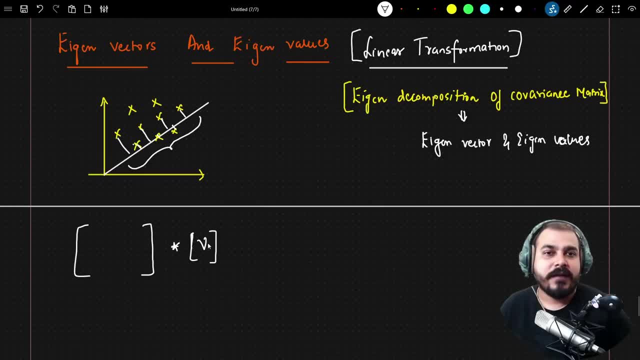 different coordinates. let's say, if this vec, on this particular vector, let's say, if i apply some linear transformation, okay, what does this linear transformation basically mean? i'll give you an example. that basically means: on this particular vector, let's say, if i apply a linear transformation, 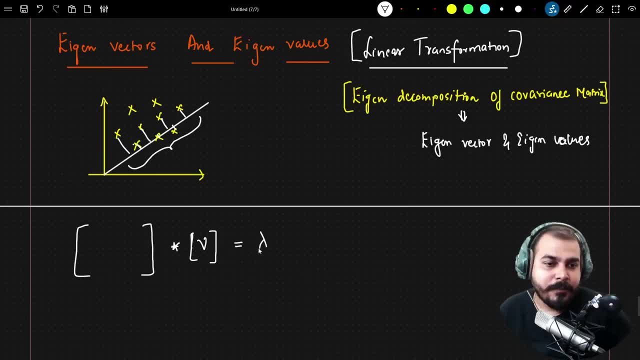 with this specific matrix, then i will be getting one lambda value, and this lambda is nothing but my eigenvalue multiplied by the same vector. so here you can see that this basically means that suppose i have a vector with this particular dot. on top of this, if i apply linear transformation, 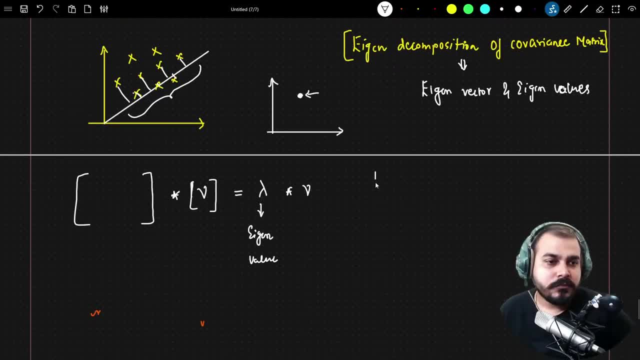 what does linear transformation basically mean? let's say i have my coordinate system and right now it is in this grid manner. okay, let's say this is entirely. all my data is in this grid manner. right? when i say linear transformation, you know this entire data can be moved, or this entire plane can be moved in different, different direction. 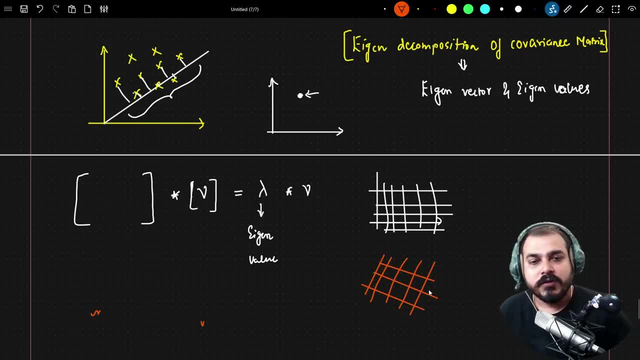 okay, i'll just show you one, one example directly, so always understand, in order to compute the eigen values and vectors. so what we do is that let's say, if a is my matrix, okay on top of it, if i apply this matrix on on the top of this specific vector, like if i apply the linear transformation on top. 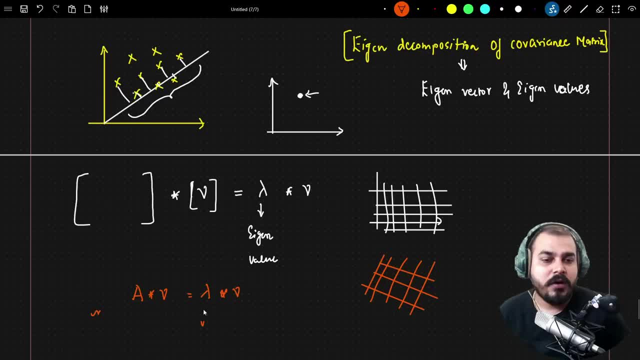 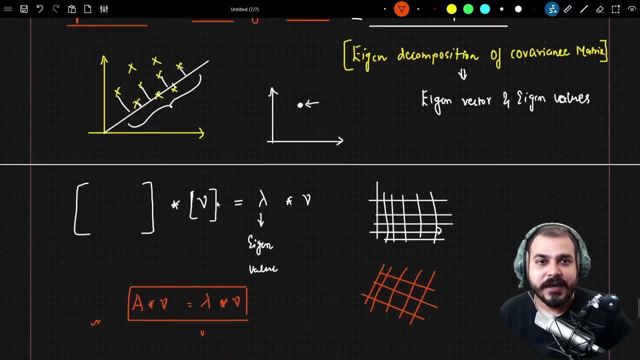 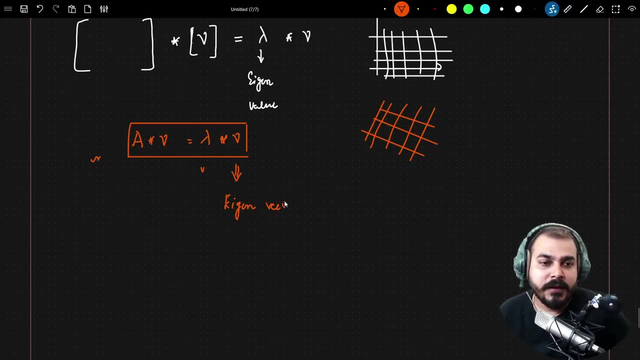 of this specific vector, I will be getting lambda, which is my eigenvalue, along with that same vector. So this is the equation that I will specifically be using in order to find out eigenvalues and eigenvectors And, from this equation, whichever eigenvector has the biggest magnitude or has the maximum magnitude. 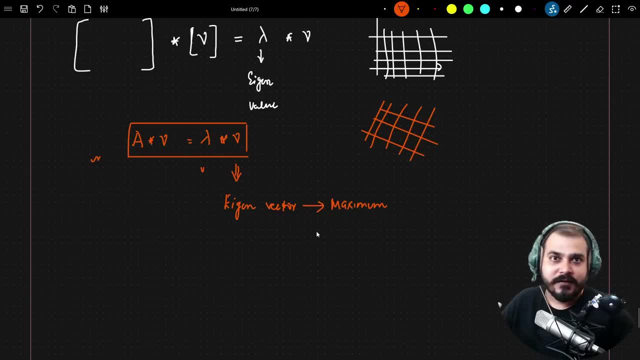 because for a space for a matrix I can definitely have multiple vectors. So from this, whichever has the maximum magnitude, that will be used as a plane or principal component, because it is practically proved through maths- Again, I'm not going to go towards that particular proof, but this principal component will be able to capture maximum variance. 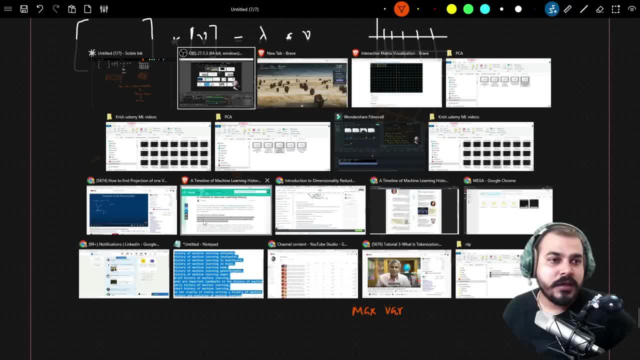 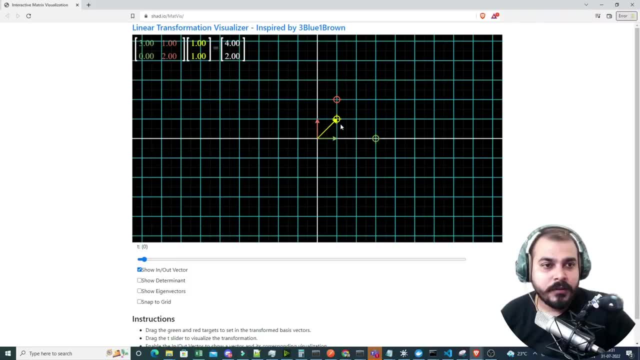 So let me go ahead and show you one example. So here I will just show you one example. So this is a linear transformation. Let's say I have one vector over here. OK, I have one vector. So this vector is nothing but one comma one. 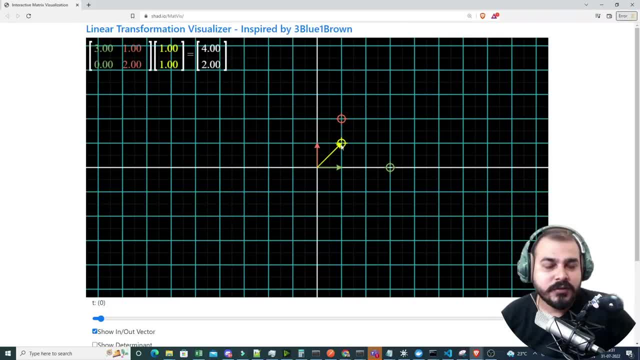 Right, So here, I hope everybody is able to see this. OK, one comma one. So this is my vector. Now, on this particular vector, if I apply a linear transformation with this matrix- OK, with this matrix. now what will happen? 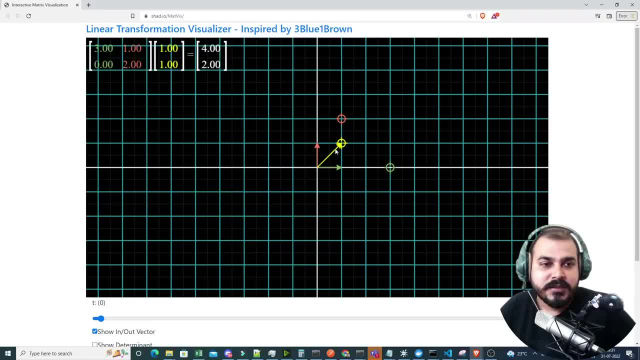 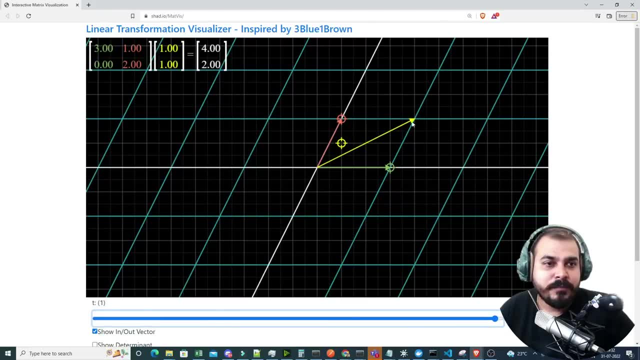 You see, because once we do the linear transformation, this particular line will now get changed and it will display something like this: See, after I apply This transformation, my new points that I'm going to get is something like four, four, two. right now four two is nothing, but here you can see, the lambda value will be four comma two, because one, one zero, one zero, one point zero. one, one point zero is my vector right. 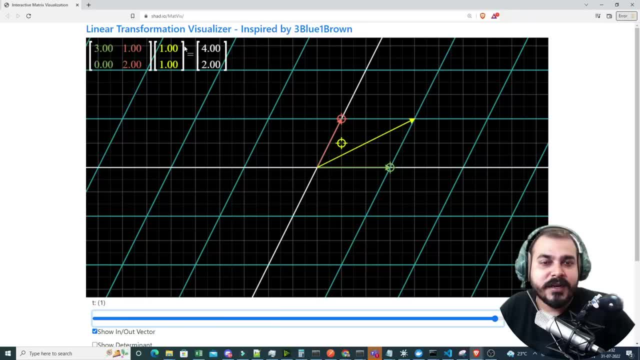 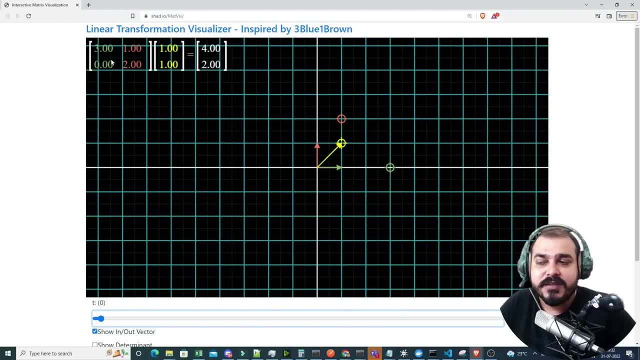 So here also you'll be able to see, I can multiply lambda multiplied by this particular number. So here you can see four comma two. That basically means for a vector, If I apply a linear transformation with this particular matrix, I'm going to get a lambda value with four. 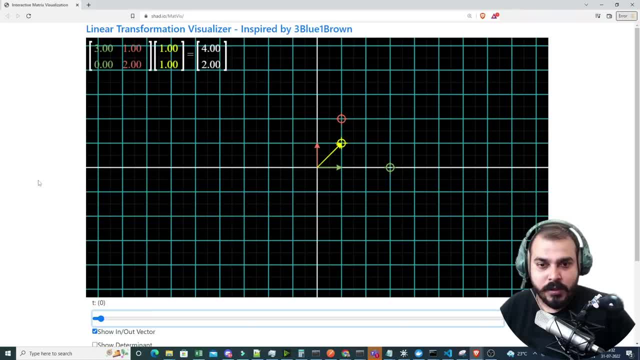 And two as its lambda, as its eigenvalue. Now let me just show you the eigenvectors also. Let's say, here I've checked on eigenvectors, and let me also show the snap grid. OK, so here you'll be able to see what is basically happening. 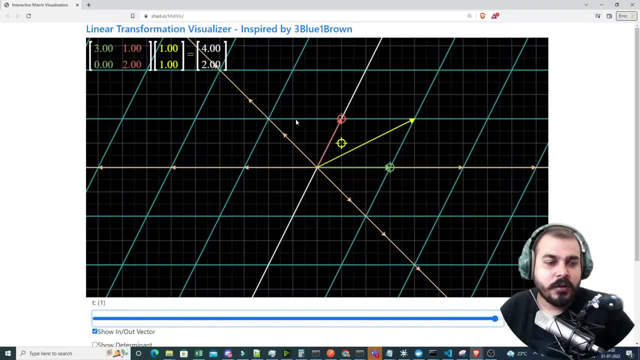 This line that you see right, This is basically my vector. OK, now, here you can see. for this particular point, when I apply this transformation, the vector is in another direction, and this is in another direction. right Now, let's see. 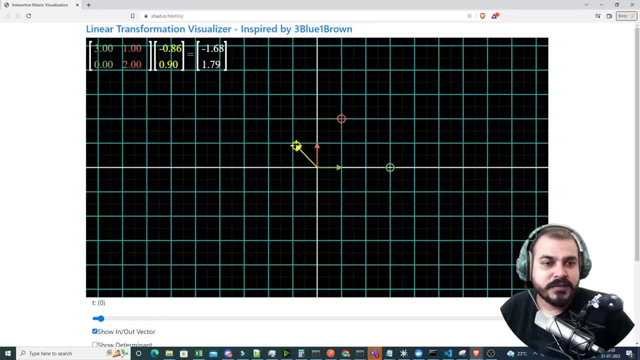 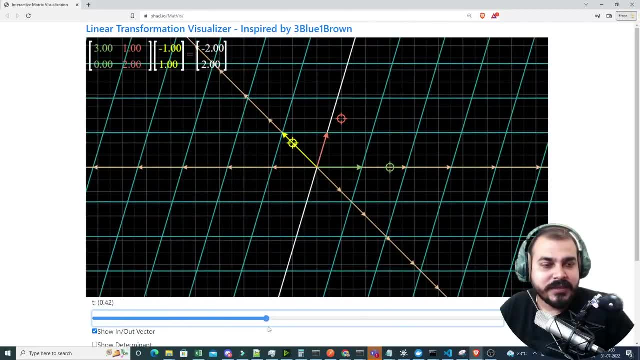 Let's say my initial point was somewhere here. Let's say my initial point was somewhere here, And if I probably apply the same operation now, it is minus one zero, right. Then what will happen is that you can see the new transformation, right. 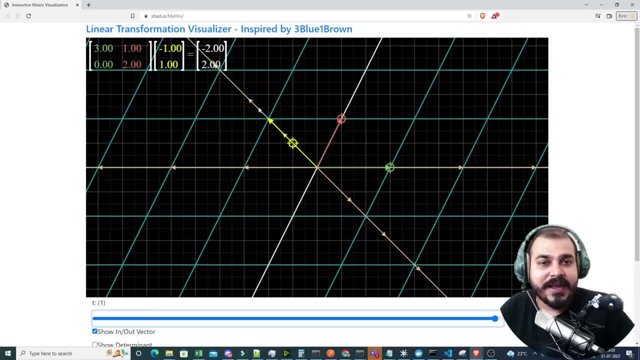 I'm actually getting minus two comma two, And here you can see this is in the direction of the vector. So what I can do is that I can project this particular point into this plane, right? So here this will be my longest vector with this longest magnitude. 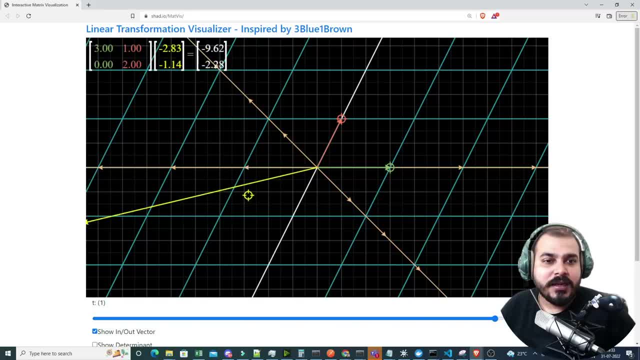 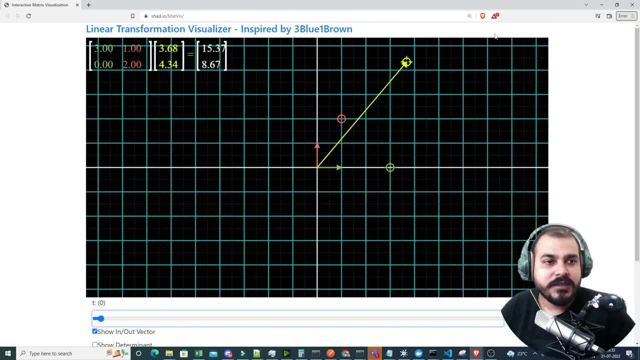 Just for an example, I'm considering like that: If I keep on doing another and other points, right, If I keep on doing, let's say I'm putting it over here, right, And if I go back here you'll be able to see this was my initial vector. 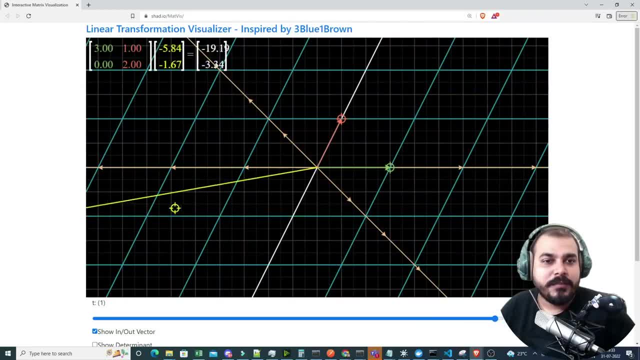 Now, after applying linear transformation, it has gone outside the plane. Similarly I can- And this time vector did not match- Suppose. if I have this point over here and if I try to apply it here, you can see again: this will get transformed to different, different values. 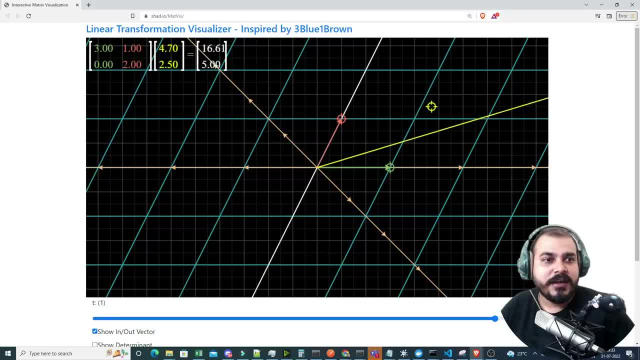 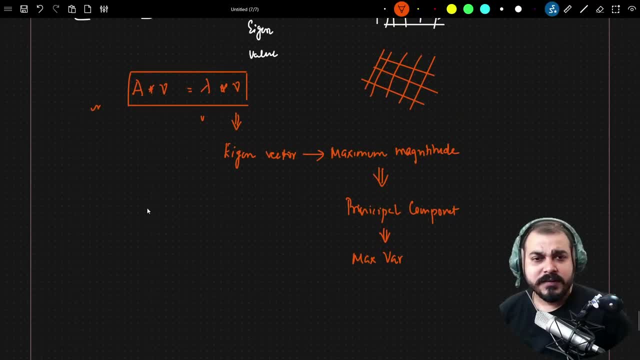 So your lambda value will keep on getting changed based on the different, different vectors. OK, so from this I can- We can definitely see that what is happening is that from this specific equation we will be able to get the eigenvectors. 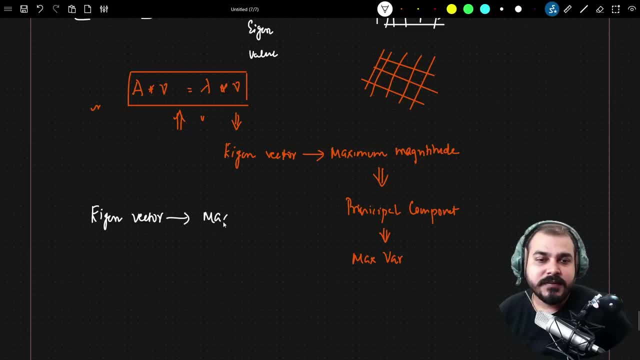 And this eigenvector which has the maximum magnitude. When I say maximum magnitude, that basically means the max eigenvalues That will be selected as the best principal component line. OK, In this particular case It is PC1. Because it captures maximum variance. 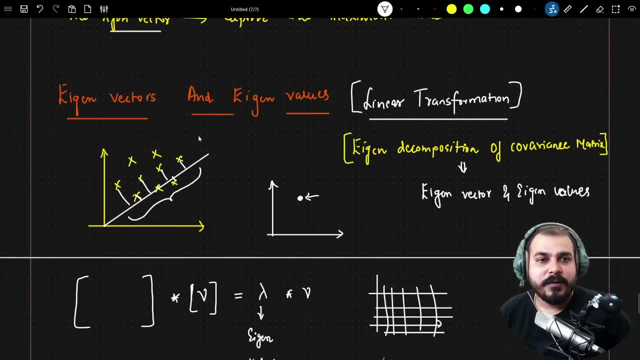 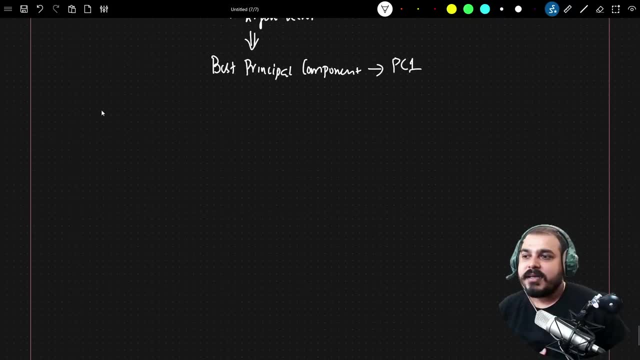 OK, so at the end of the day, you'll be able to see, with the help of this, eigenvectors and eigenvalues. You'll be able to see this. OK, and the same thing is happening Now. let's go ahead and understand the steps to calculate eigenvalues. 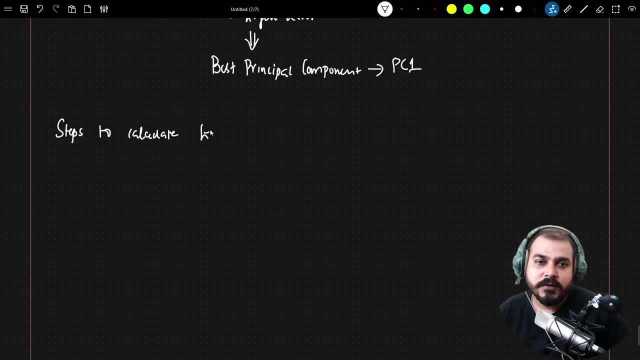 Steps to calculate Eigenvalues and eigenvectors. Value and eigenvector Because, as I said, that you require a metric Right. In this specific case, we have to calculate the covariance of The features Right Now. let's say, if your features were X, Y, your independent feature, and this is your Z as the output feature. 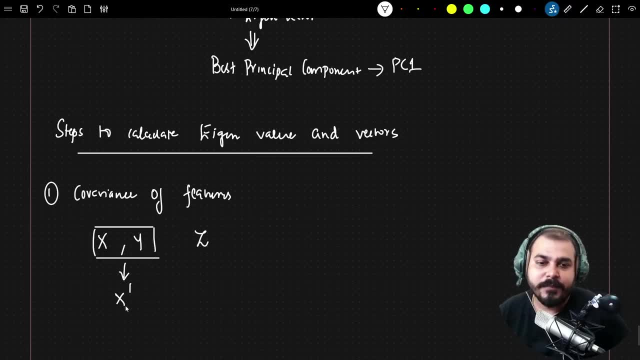 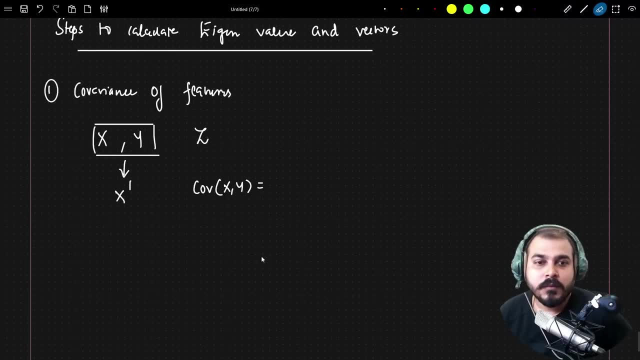 So for this I want to extract another feature which will can be X- dash. So what I'll do is that I will try to find out the covariance of X- Y. So let me write down the equation of covariance of X- Y. 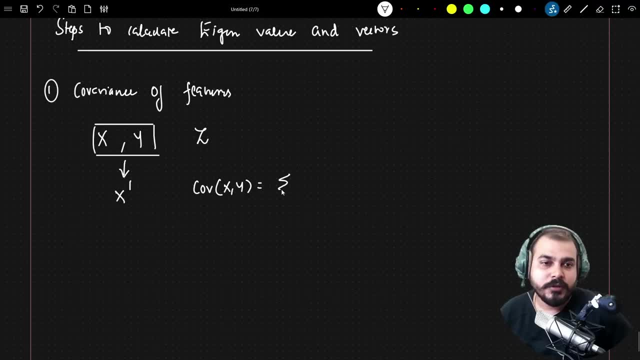 So here you can see That I will be able to write: summation of I is equal to one to an X of I minus X bar multiplied by Y of I minus Y bar divided by N minus one. OK, now, here you can definitely see that if I really want to find out the covariance of X- Y, usually we get two cross, two metrics. 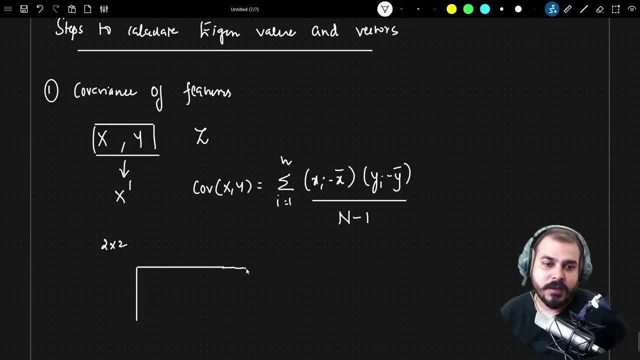 OK, now this specific metrics looks something like this: OK, let's say, I'm just going to divide like this. So this will be a two cross, two matrix. This will be X, This will be Y, This will be X, This will be Y. 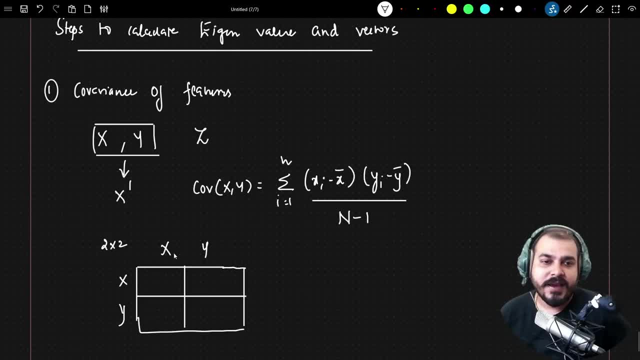 So if I try to find out the covariance of X comma X, then what it will become. So if I try to find out the covariance of X comma X here, you'll be able to see. I will. I can also write this as variance of X. 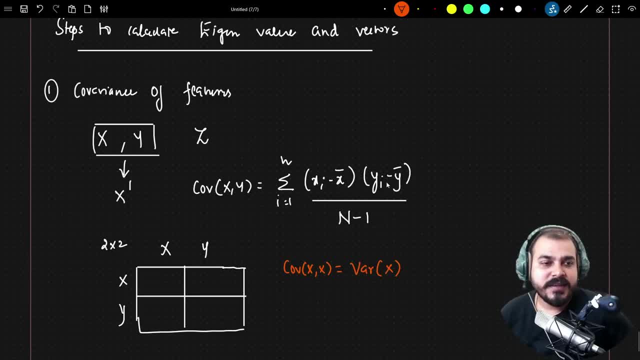 Why? Because X comma X basically means X of I minus X bar, Right. So X of I minus X bar will be nothing but X of I minus X bar whole square, which is nothing but variance of X, Right. So here you'll be able to see that I will write variance of X here. 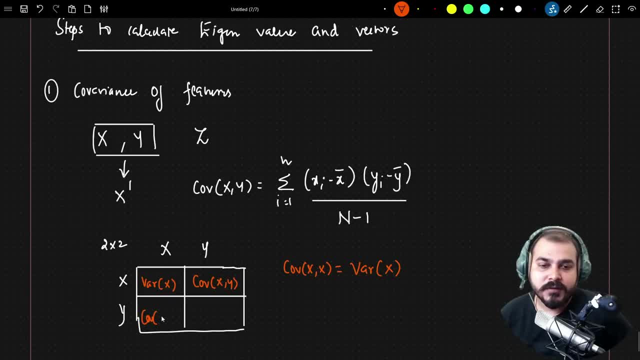 This will be covariance of X comma Y, here It will be covariance of Y comma X, And here it will be variance of Y. OK, because covariance of Y comma Y is nothing but variance of Y. Right Now, this is the first step. 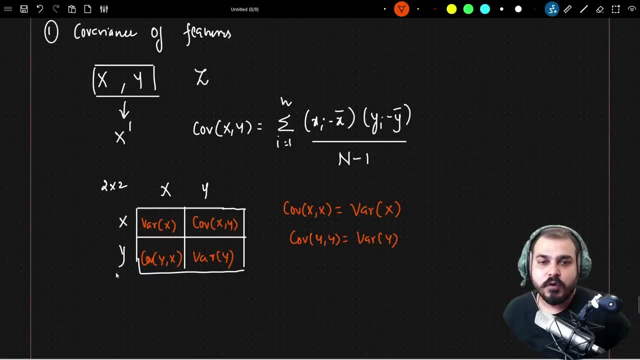 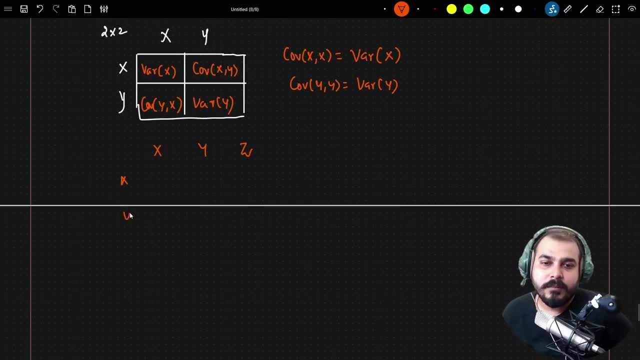 We have to compute this specific metrics And this is for a two cross two metrics. If suppose if I have three, If suppose if I have three independent feature- X, Y, Z- then I have to probably create three input, three cross three metrics. 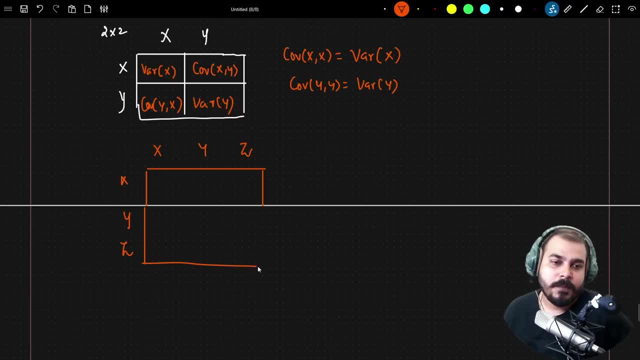 Right, I have to basically create, like this, three cross, three metrics. Now here you'll be able to see that I will be creating this kind of lines, And here will be one, Here will be another Right Now, again here, all in the, in the diagonal element, it will be the variance of X, variance of Y, variance of Z and remaining all. you'll be able to see this. 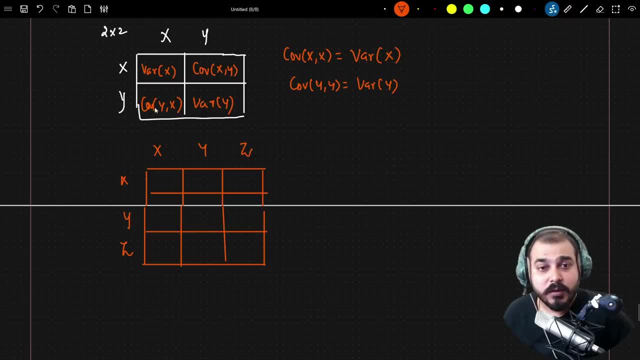 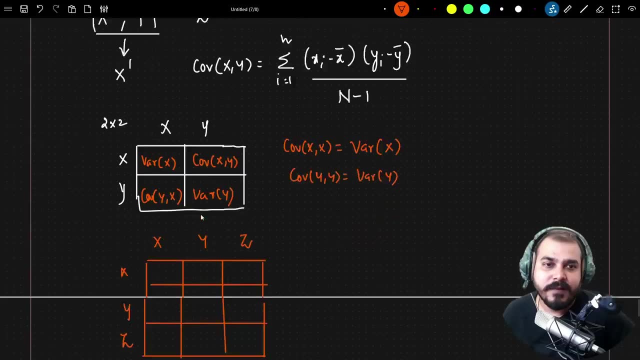 And one more thing: That variance of covariance of X comma Y is equal to covariance of Y comma X. This both will be equal. Right Now what we are going to do: in order to find out the eigenvalues, we will take up this covariance metrics. 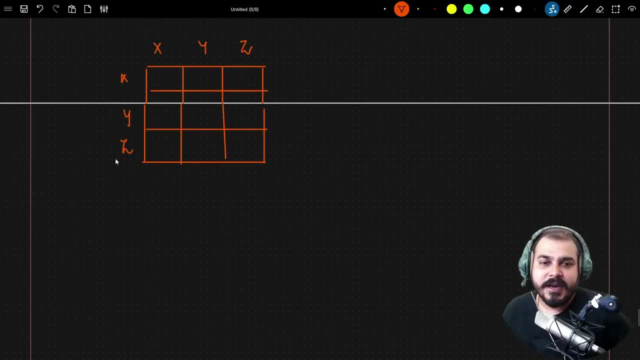 This. let's consider it is A And we will try to take a vector V And this A will be taken, which will be my covariance metrics, And I will try to apply a transformation of the vector And, finally, we will be getting lambda. 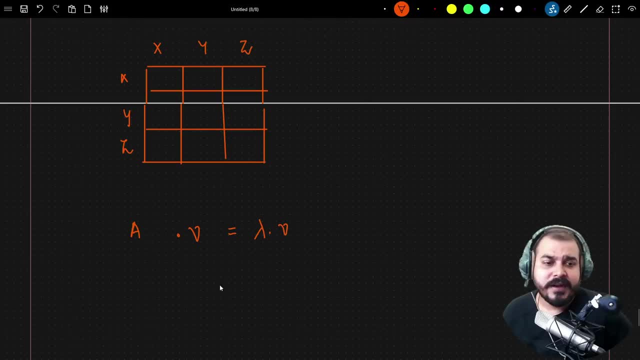 Lambda over here And this vector. This vector will be given back Now, since I have two features over here, F1 and F2,. let's say, then I will be getting two lambda one, values like lambda one and lambda two. 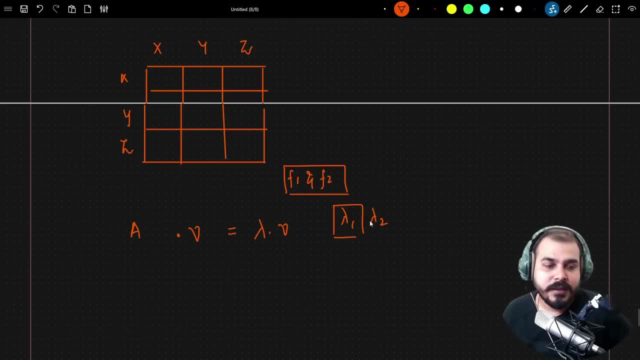 Lambda one will basically be giving my principal component line one magnitude, And whereas my lambda two will be giving me the principal component to magnitude Right. So this will be PC one Right. So like this, When you have three features, you are going to get all lambda one. 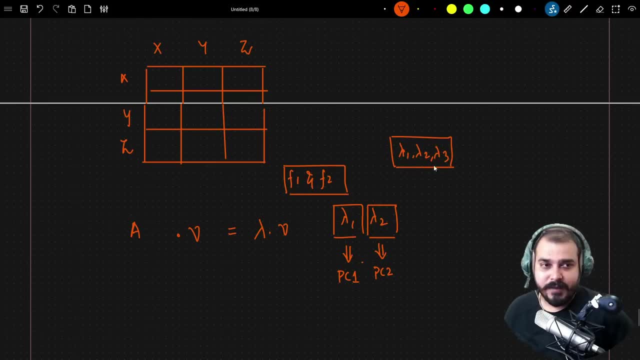 Lambda two. Lambda three, Which will specifically talk about the eigenvalues. So just by using this equation, at the end of the day you will be getting an eigenvector And that eigenvector will be giving you two or three, based on the number of features that you have, that many lambda values. 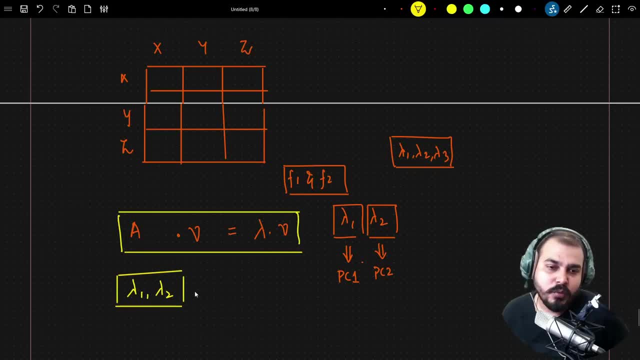 Let's say, if it is giving lambda one and lambda two, that basically means you have two eigenvalues And whichever eigenvalue is the highest over here, that will be And it will already give that And that specific value in. like the lambda one will be the highest and lambda two will be the highest. 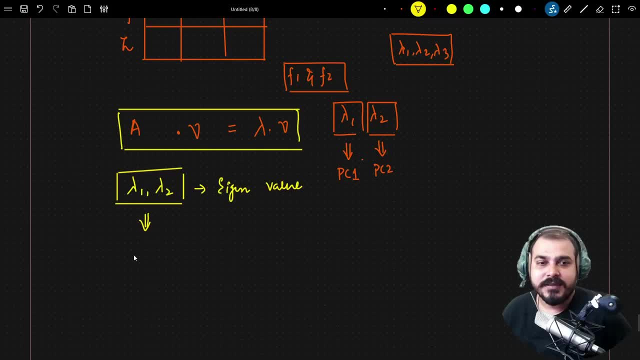 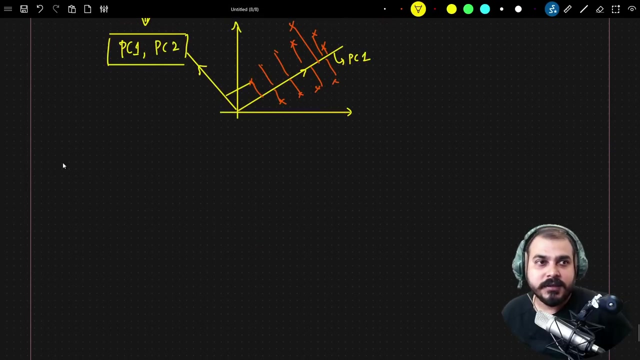 So this way, you'll be able to get this lambda one and lambda two, which are specifically the eigenvalues, And then this can be considered as PC one and this can be considered as PC two. So, guys, just to revise all the steps. now, what we are going to do is that let's consider the first step over here. 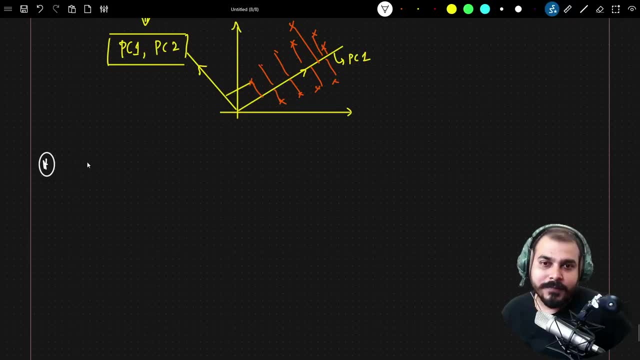 So I'm going to write it down, The first step that again we are going to do. Let's say that I have my data points over here, So let's say this is my X and Y. And let's say I want to probably first of all convert this into 2D, from 1D to 1D. 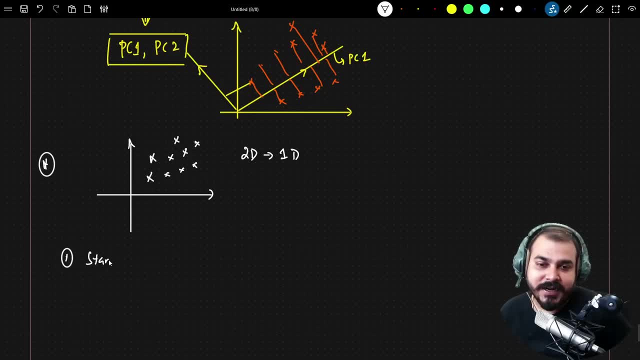 Then the first step that I am actually going to do is basically standardize this data. Now, once I standardize this data, what will happen is that all these data points that you will be seeing it will be zero centered. So here you will be able to see all the data points like this: 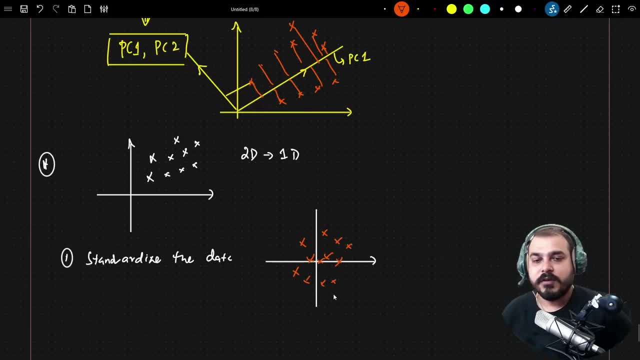 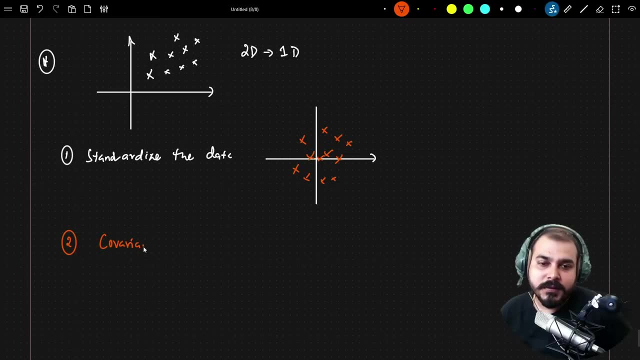 OK, Let's say these are my data points, that I've got zero centered. After this, the second step is that we go ahead and find out the covariance matrix of this X and Y. OK, Let's say this is my X and Y. 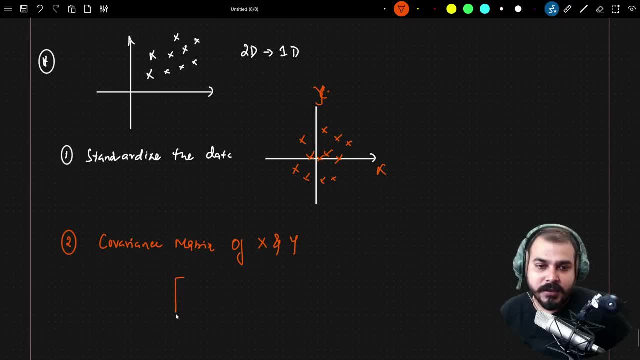 So we basically find out the covariance matrix And again, in the case of two independent features, two independent features. I'll be getting a two cross, two matrix, Right? So this will basically be my two cross, two matrix with respect to X and Y. 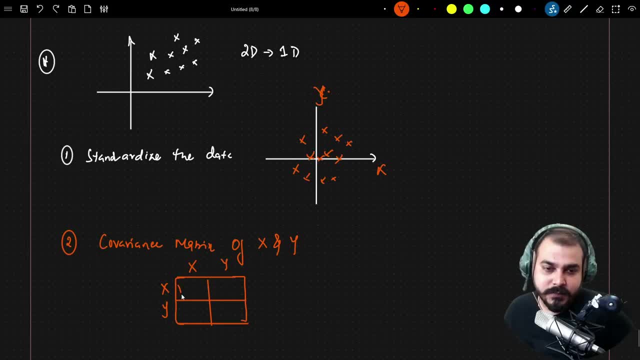 X and Y. Here I'm going to get the variance of X, And here I'm basically going to get covariance of X comma Y, And here I'll be getting covariance of Y comma X, And finally I'll be getting variance of Y. 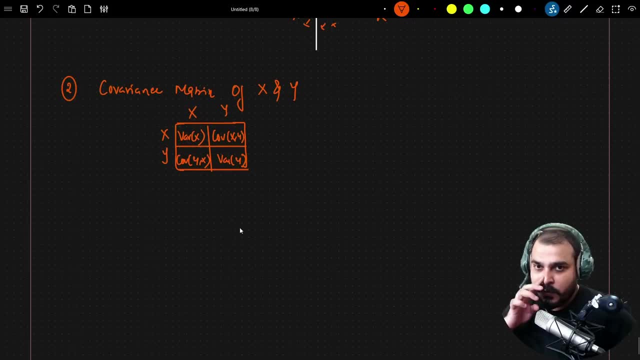 Right Now, after I get this covariance matrix, all I have to do is that: find out, find out eigenvectors and values, Vectors and values. And how do I find it out? by just applying. Let's say, this is my matrix A. 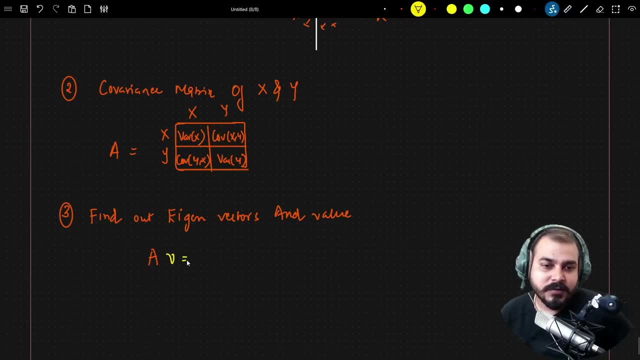 So this: A, when we apply a transformation on vector B, I'm going to get this eigenvalue of V Right. Since this is a two cross, two matrix, here I'm going to get lambda one and lambda two. OK, So this two values are my eigenvalues and eigenvalues. 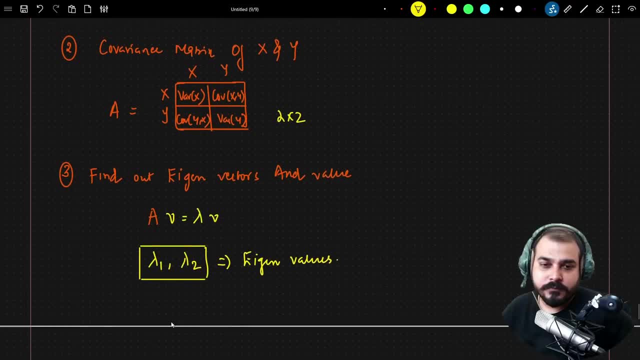 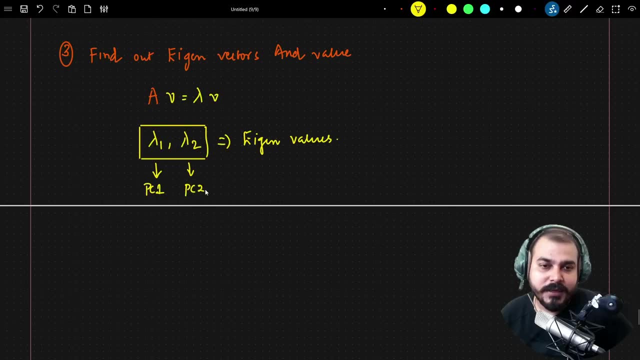 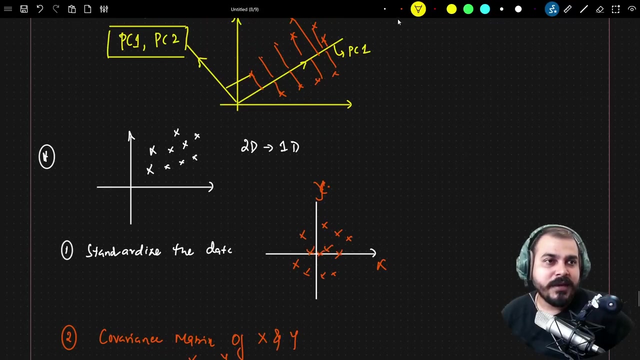 OK, And this, This lambda one, will basically be indicating me by PC one, That is, principal component, one line, And this will be my PC two line. So, in short, after this particular points, what we are going to do is that let's say that we will be creating two different line. 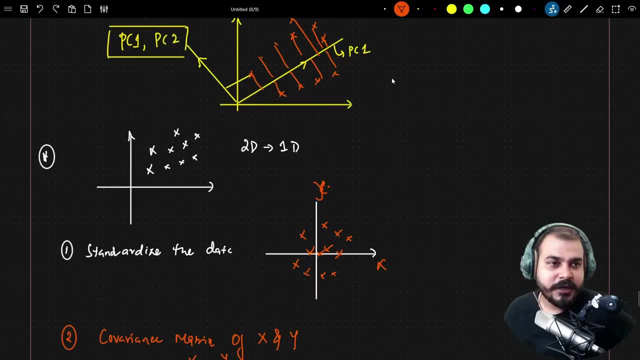 One line may be this. One line may be this- Let me just draw it in different color. So let's say this may be my PC one, OK, So this may be my PC one And this may be my PC two, OK. 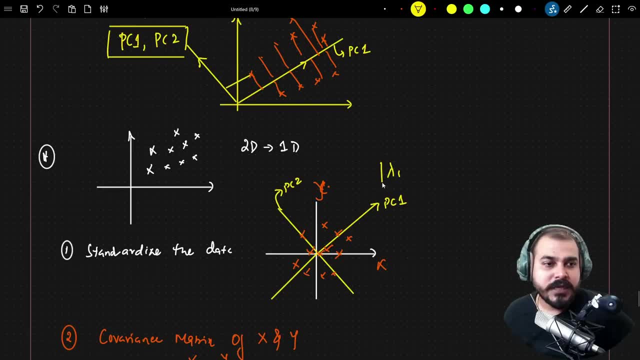 But as we know that the first lambda one value which I'm getting, which is nothing but the magnitude of the eigenvector, Magnitude of the eigenvector, Here it will capture the maximum variance. So this variance that is getting captured will be maximum. 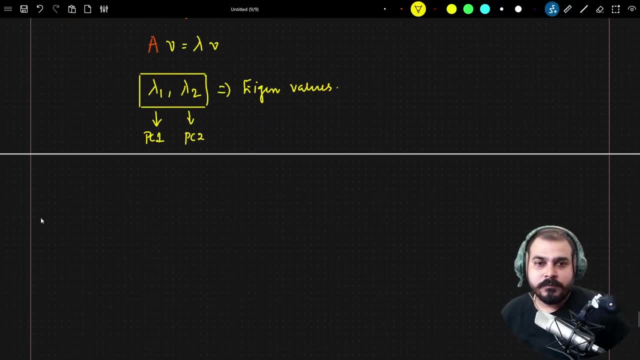 So we go ahead and select this. Now, let's say, if I want to convert from a three dimension to one dimension, Then what will happen? I will get three lambda values, That is, three eigenvalues. Now what I can do? I can combine this two- lambda one and lambda two- and probably take 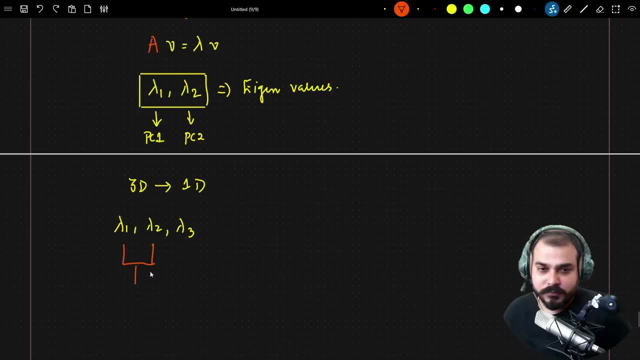 OK, Since I have already explained you this lambda one is nothing but PC one, This is PC two And this is PC three. Right, So I can combine PC one and PC two and convert this two dimension into one D, And then this can also be taken as one D. 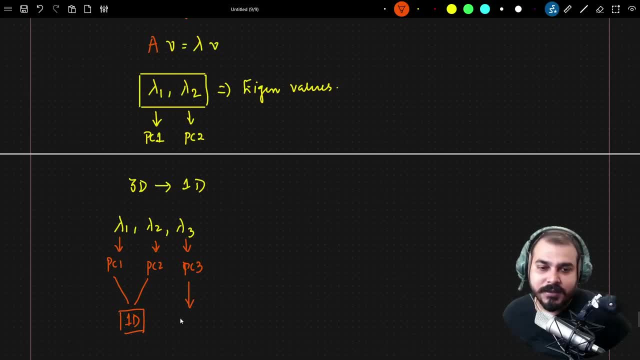 OK, And this can also be taken as another one D. So when I combine this two right, it becomes a two D Right. So if I probably want to convert from three D to two D, I'll be going in this way. 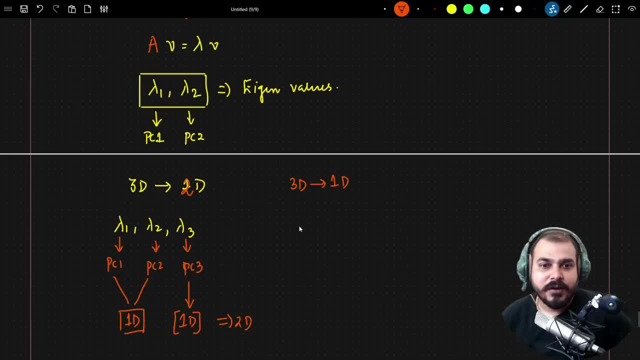 So let's say, if I want to convert from three D to one D, So once I find out my eigenvalue and vectors, I'll be getting lambda one, lambda two, lambda three. I have to combine all these three and probably get one dimension in this case. 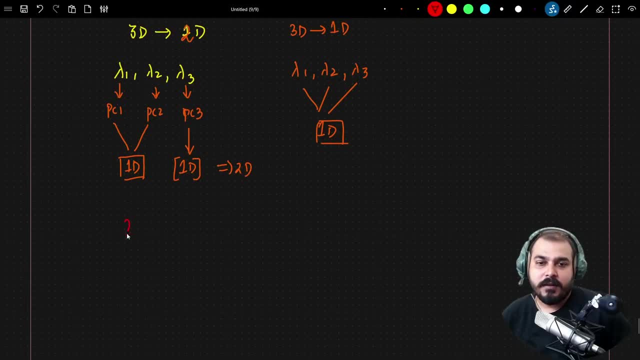 Similarly in the case of two D to one D. So let's say, if I want to convert from two D to one D, here I'll be getting lambda one and lambda two. This is nothing but my PC one. This is nothing but my PC two. 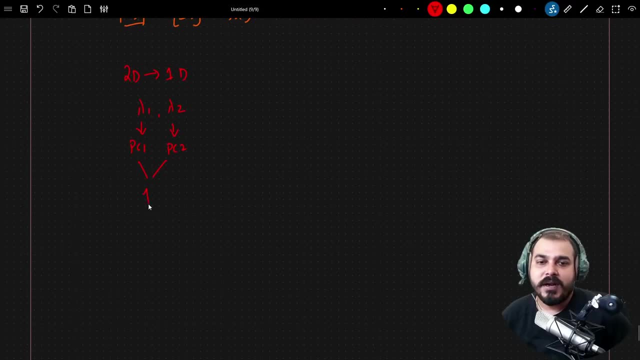 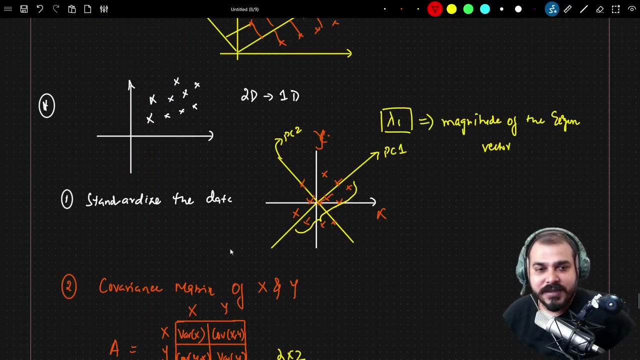 So we can combine this two both, and we can get a one dimension point Right? When I say combining, that basically means I'm talking about projection. Once I project all the point, I will be able to get that specific dimension. So I hope you have got an idea, but these are the steps that we basically follow in. 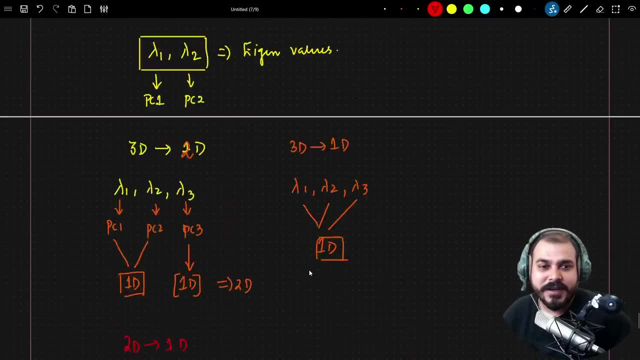 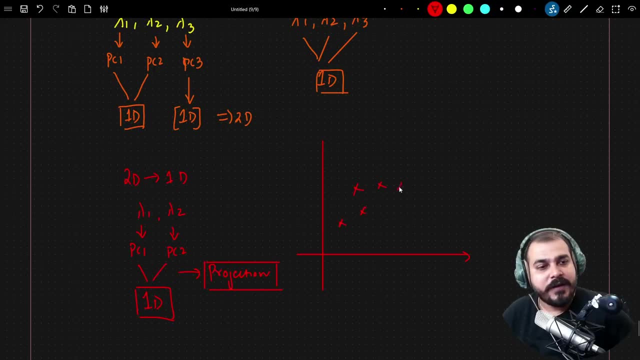 order to find out the projection. But at the end of the day, you know you are trying to find out. you are trying to find out with respect to any data points. you're trying to find out the best principal component line that can fit on this data such that it captures maximum variance. 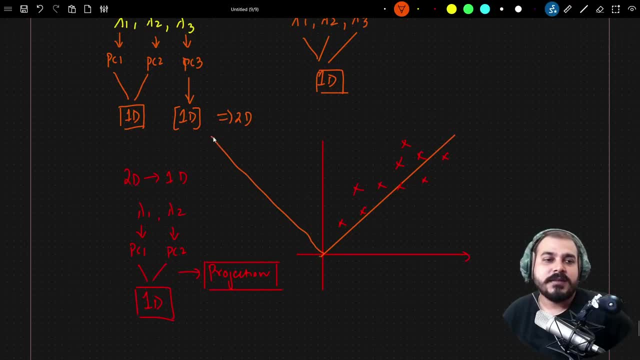 Now, in this case, this can be, or in this case, this can be right. So this can be my PC one, This can be my PC two. I'm saying this because maximum variance is captured. See, maximum variance is getting captured. 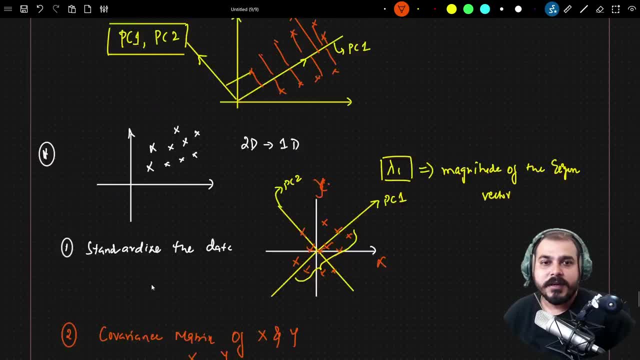 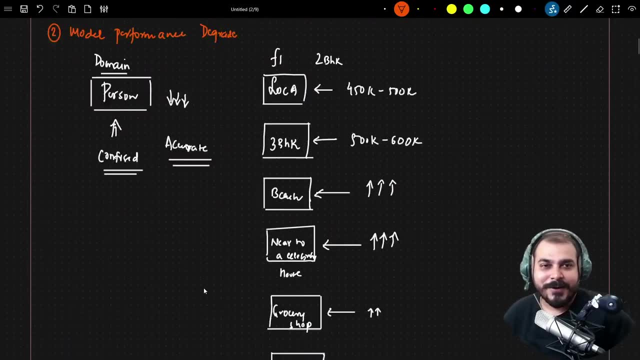 Right. So this was the idea behind principal component analysis. I hope you have understood the math behind it. If not, I would suggest please revise it. I've written on nine pages just to make you explain about principal component analysis. Hello all. 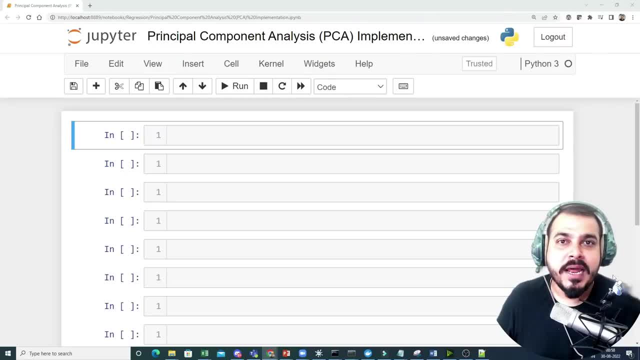 So, guys, in this video we're going to implement the principal component: analysis implementation, where we'll focus on doing dimensionality reduction Or we can also say feature extraction. We'll try to see that, how we can implement this with the help of a scalar and Python. 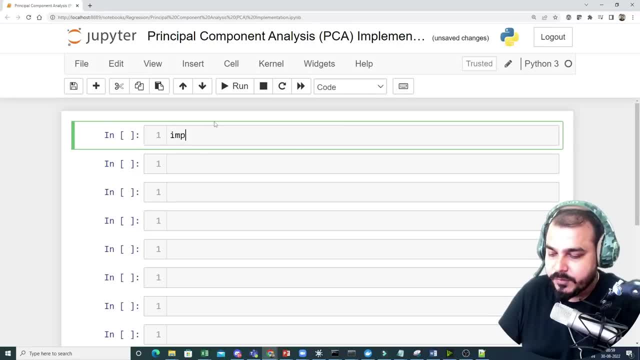 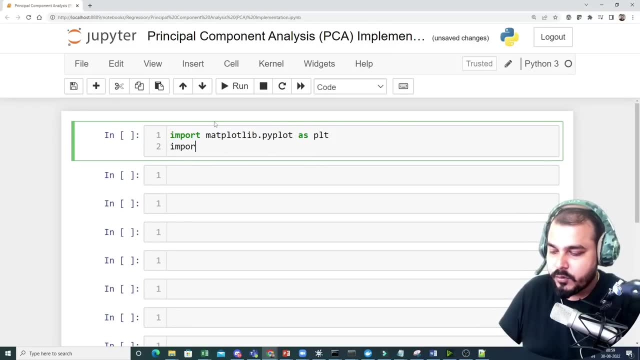 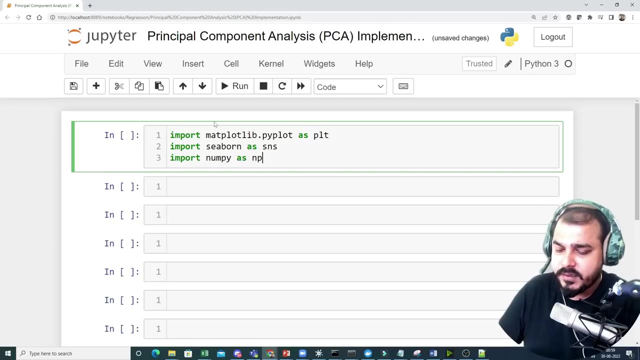 So, to begin with, what I'm actually going to do quickly is that import some of the libraries like: import matplotlibpyplot as PLT, Okay, Import cbon as SNS, Import numpy as NP, And I can also import pandas as PD. 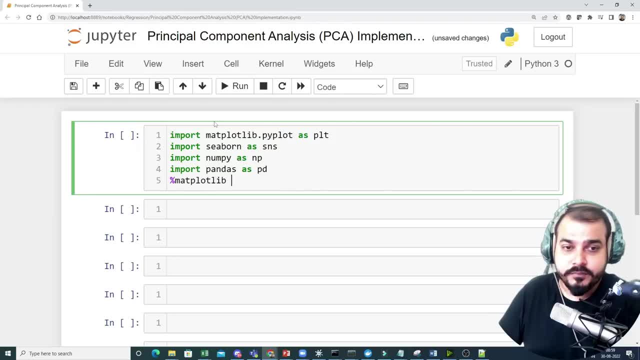 Along with this. I'm just going to say matplotlib, inline, Right? So all these things, we are basically going to import it. Now, what we are actually going to do is that we are going to first of all load our data set. So, load the data set. 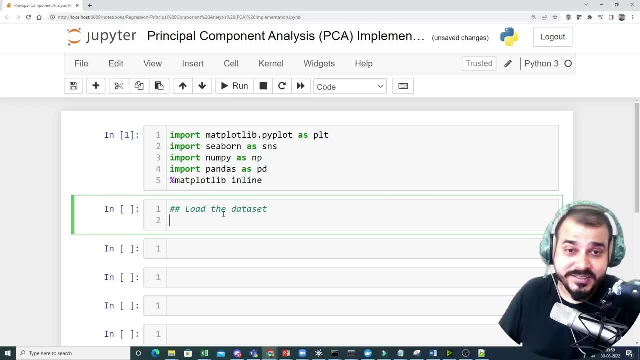 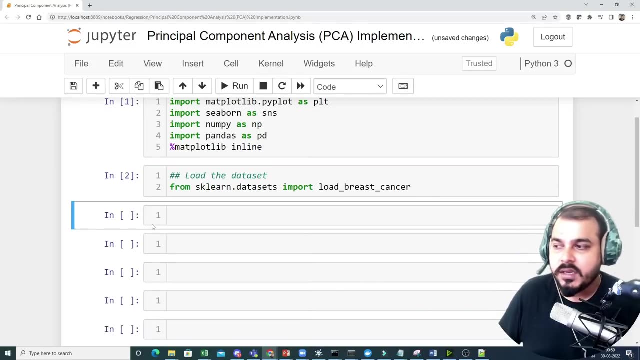 And the data set that we are going to play is with the breast cancer data set. So over here you'll be seeing from sklearndatasets if I write, we'll be able to import load breast cancer. So here it is, And what we're going to do is that, with the help of this specific data set we're just going to, I'm just going to write something like cancer underscore data set is equal to load breast cancer. 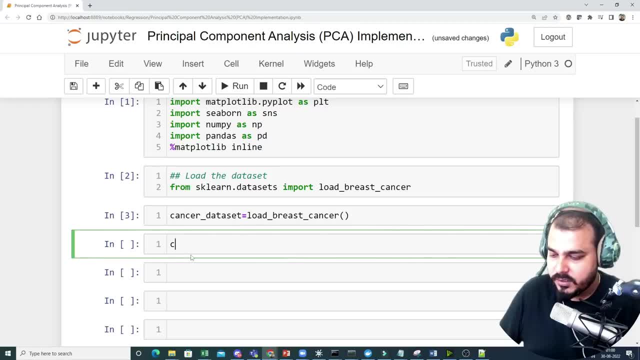 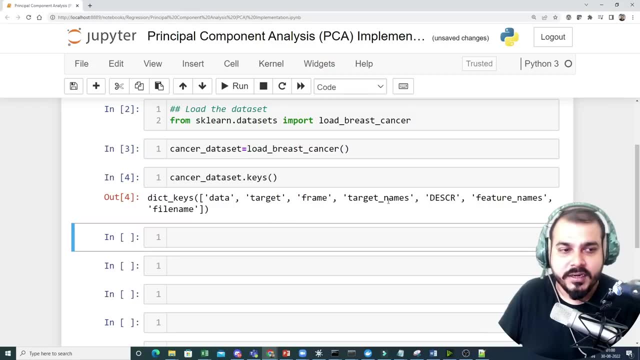 Okay, And here we go and import it Now. finally, if you probably go and see my cancer data set dot keys, you'll be able to see various keys like data target, frame, target names. Okay, So over here, and if I probably just go ahead and probably print cancer underscore data set, dot D, E, C, R, 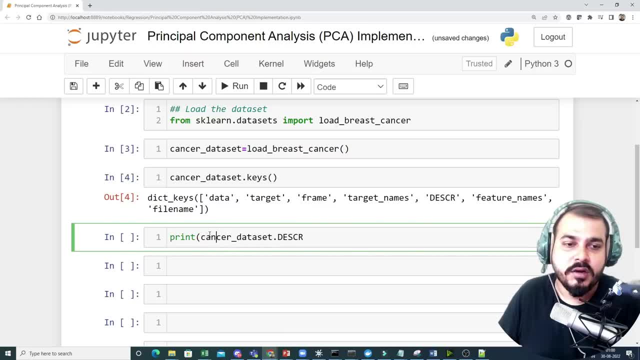 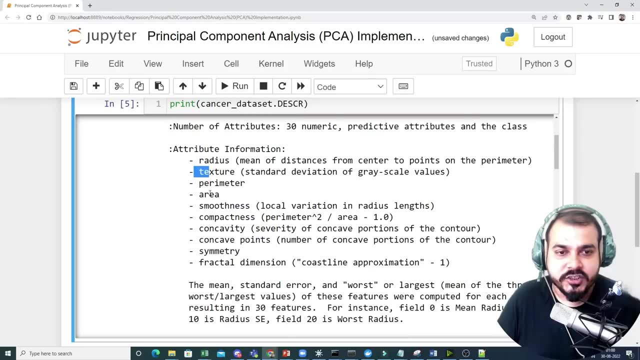 If I probably print this, you'll be able to see this entire information, how your data set looks like. Okay, So here is how your data set looks like. You can see this. You have features like radius, texture, perimeter area, smoothness, compactness, concavity, concave point, symmetry, fractal dimension. 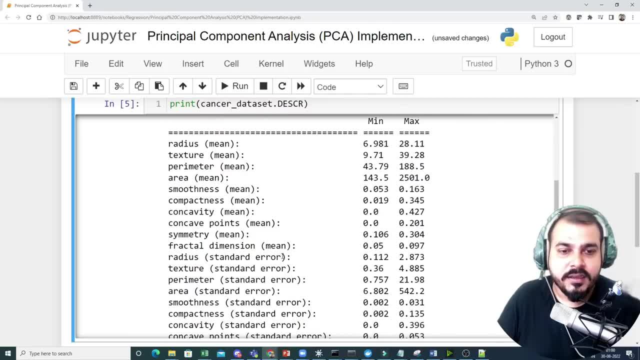 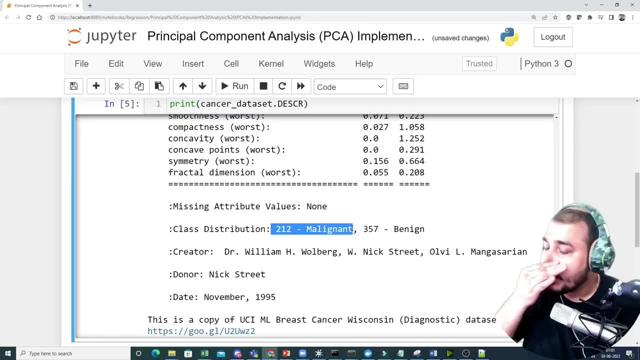 And your class is basically like this: This is basically malignant and benign. This is the output feature And, with respect to this, you have so many number of records that are having malignant as output and 357 records that has benign as the output. 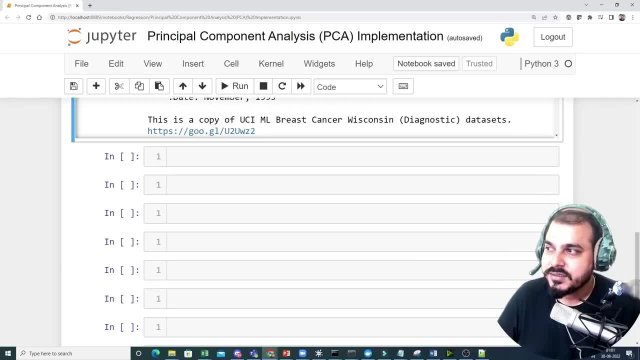 Now, in the next step, what we are going to do quickly is that I'm just going to create a simple data frame. So here I'll just go to write: D F is equal to PD dot data frame. And here, first of all, I'm just going to use my cancer data set. 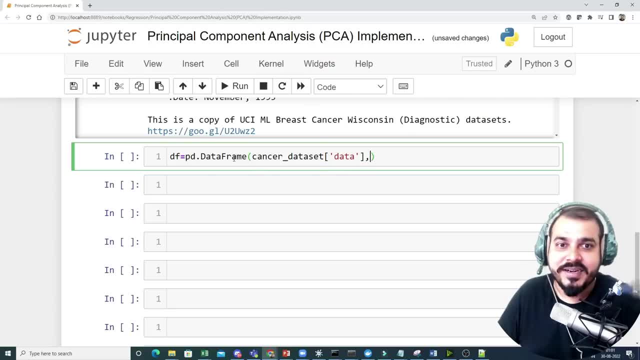 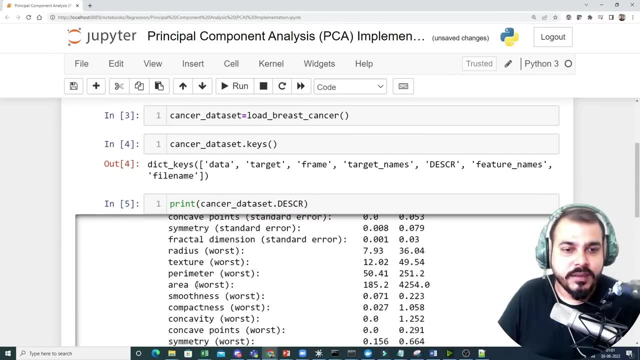 And here I'm just going to take all my data, Because that data key has the entire data over here And you can definitely check out over here itself. Right, With respect to all the attributes, you'll be able to see something like data key over here. 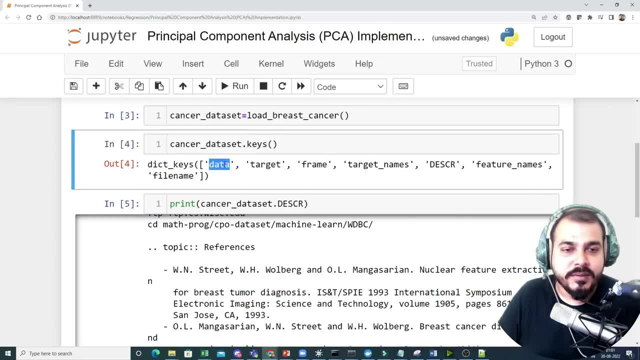 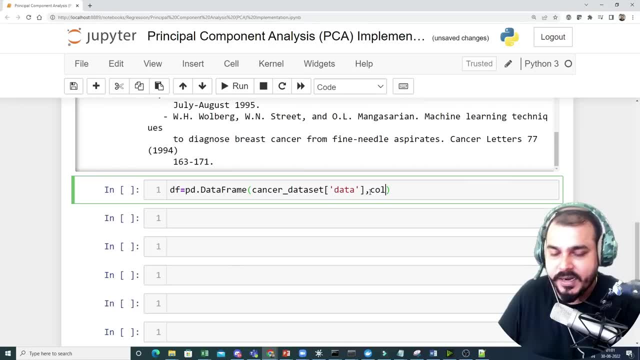 So this data key that you are able to see, right, it will basically be having that. So here, cancer of cancer, underscore data, of data, you'll be able to get that, And the columns that I'm basically going to take is nothing but my feature names. 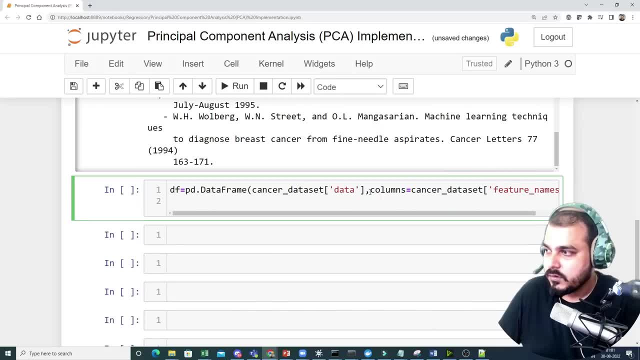 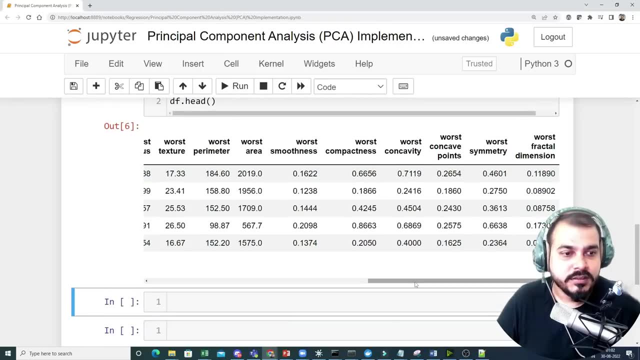 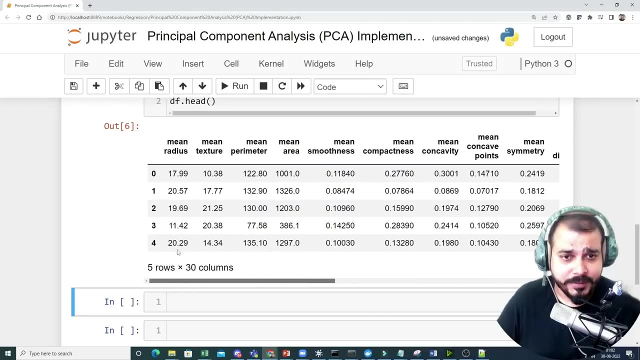 Okay, So here is my D F dot head, Right. So these are all my features that are there with respect to all this. Now, what I'm going to do is that I'm not going to just solve some classification or regression problem statement. 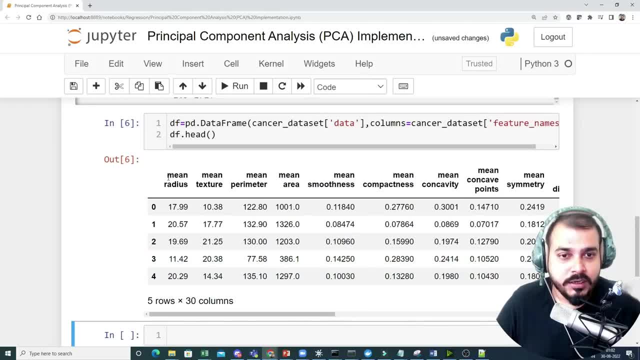 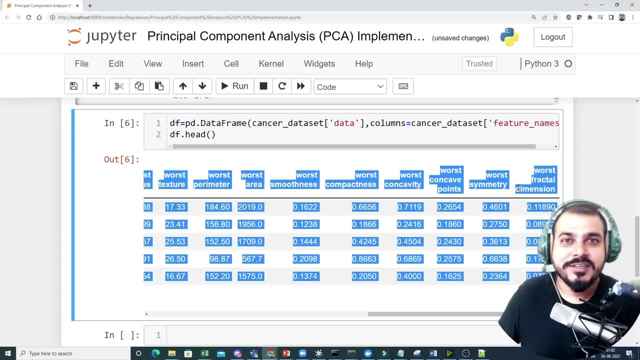 Principal component is more about dimensionality reduction. Now, let's say, if I have probably 10 to 11 features- And obviously I cannot visualize this- I have to basically convert this into 2D or 3D, True dimension or three dimension. 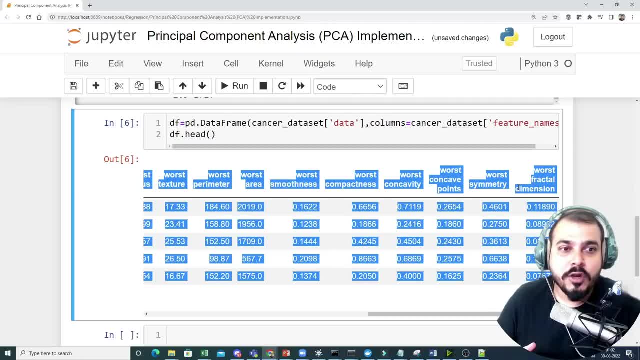 And then probably we'll be able to visualize it. But here our focus is not to remove the features, but we are going to extract some features, Making sure that some of the variance is basically getting captured And again, whatever theoretical concept we have learned in principal component analysis. 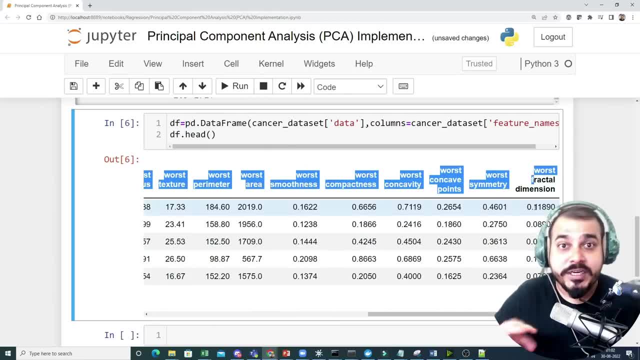 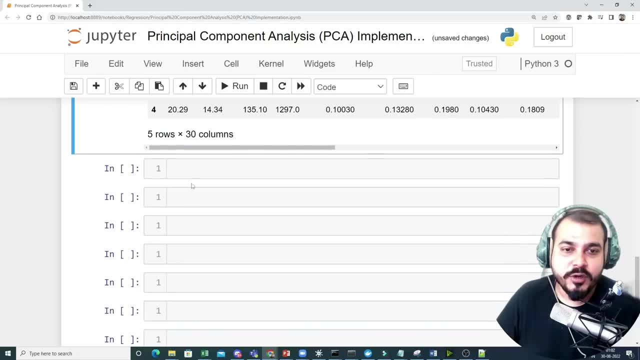 we will try, just try to take all these features and try to extract only two features. that captures the maximum amount of information out of it. Okay, Now to do this. what I'm going to do? first of all, I'm just going to apply standardization. 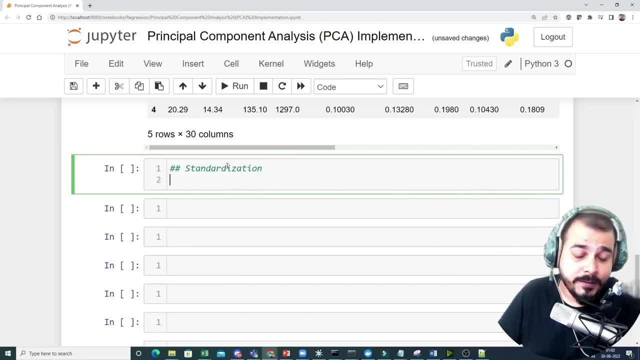 This is a good step to do in feature scaling also. Sorry, in PCA we have to definitely do feature scaling And for that we are going to use standard scalar. So I'm going to write: from sklearnpreprocessing: import standard scalar. And here I'm basically going to write: scalar is equal to standard scalar. 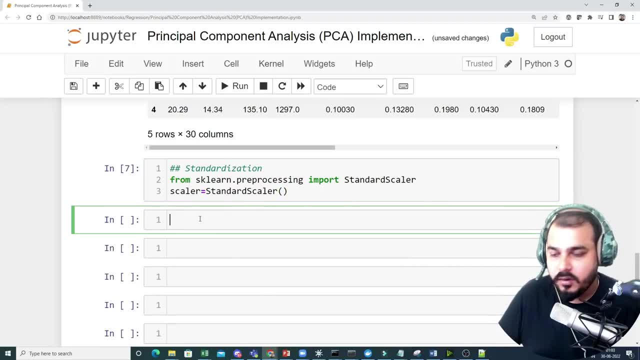 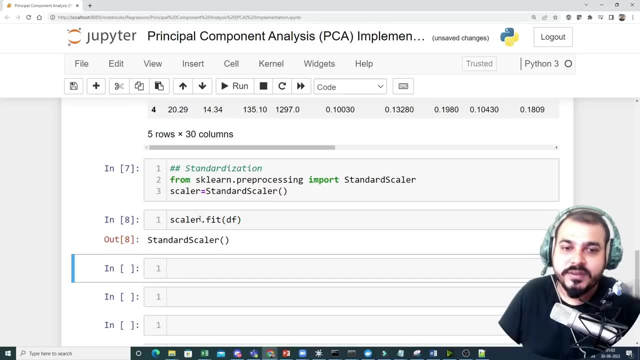 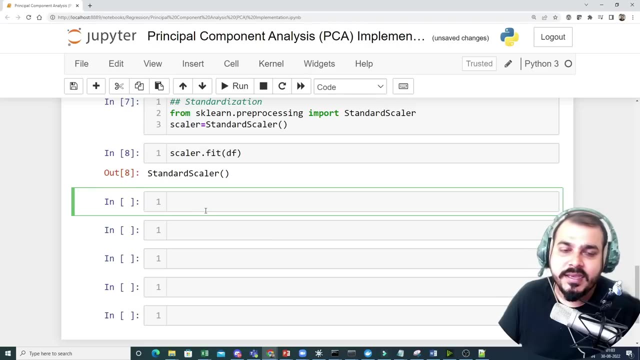 Right, And once I execute this, All I have to do Just write scalarfit on my entire DF Right. So once I do this, once I execute this, that basically means my entire fit has actually happened on the data frame And then I can transform this entire data frame based on the standard scaling. 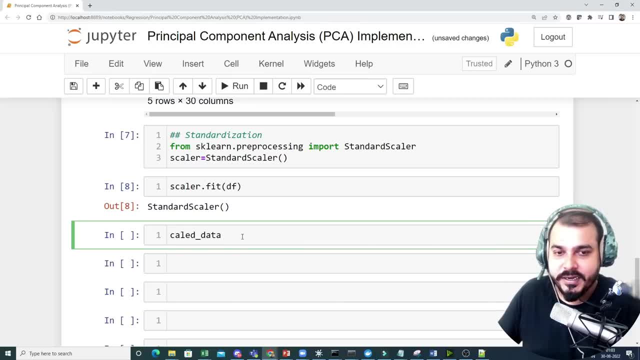 And I'll try to save it in a variable which is called a scaled data. Okay, So here, in order to perform the transformation, I'll just write scalartransform. Okay, And here you'll be able to see DF And finally, you'll be able to see my scaled data in the form of standardization. 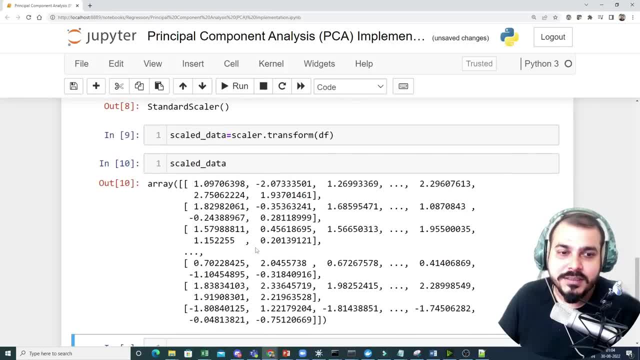 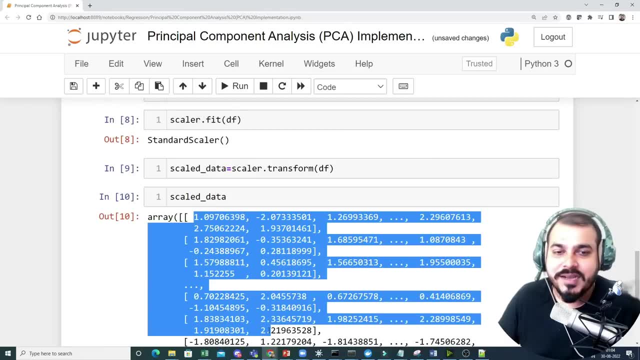 It is basically in the standardization. That basically means the mean is 0 and the standard deviation is 1. So most of your data will be ranging between minus 3 to plus 3.. Right, So that is how this entire standardization process have actually taken place. 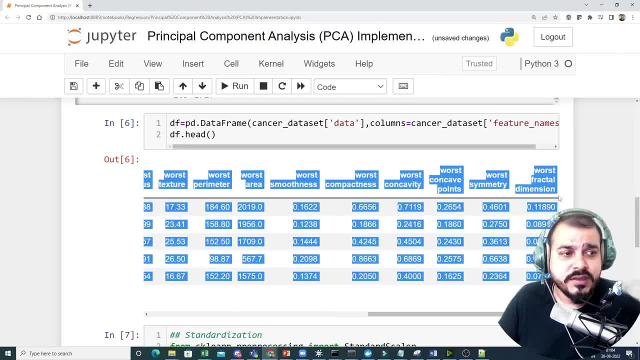 Now, what we are going to do is that, out of all these particular features, we are just going to extract two features. So, in order to do that, what we can do is that we can apply this. So what we can do is that we can apply PCA. 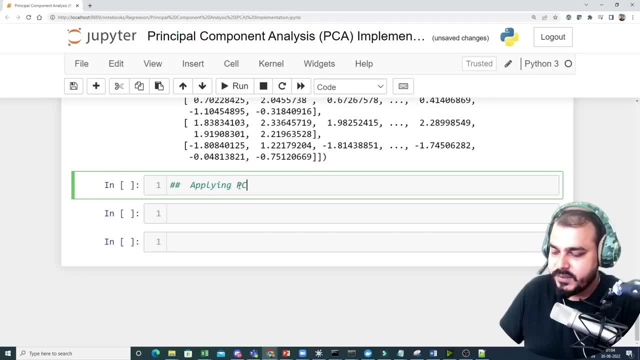 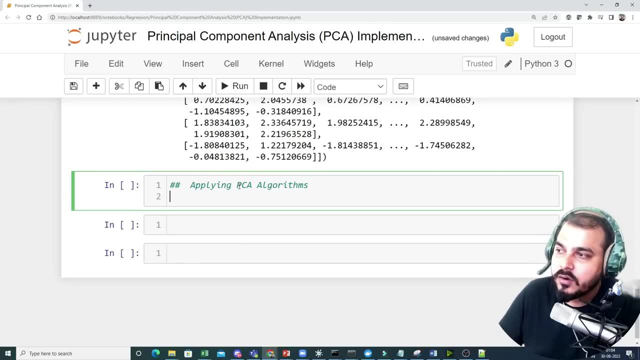 So here I'm just going to write applying PCA algorithm. Okay, And for applying the PCA algorithm, here I'm just going to use from sklearndecomposition. I'm going to just import PCA and I'm just going to execute it, And here we'll be writing: PCA is equal to principal component analysis. 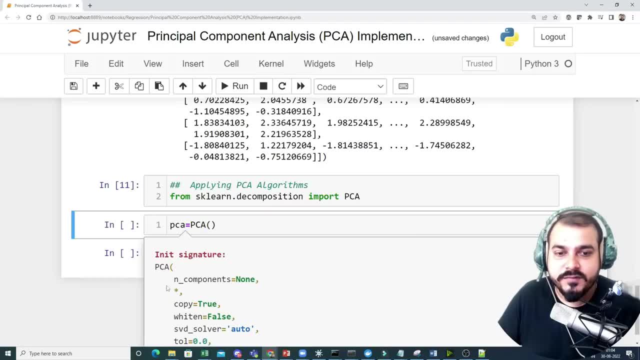 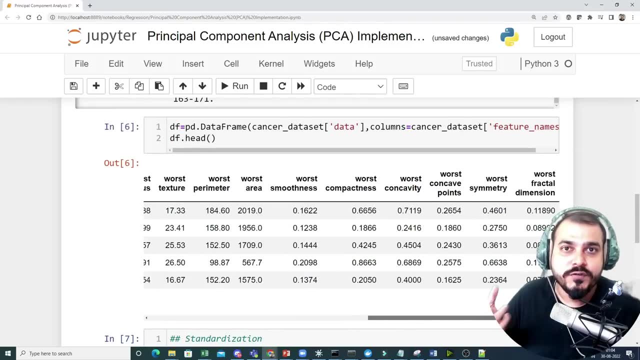 And here by default, if you probably go and see, I have to give this value, which is called as N, underscore components Right now, let's say, if I have this many number of features, I want to convert this into two features. 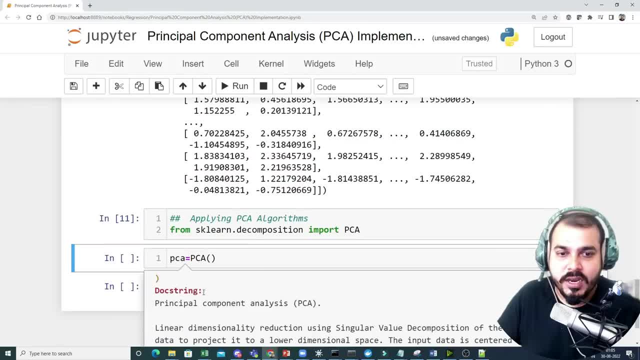 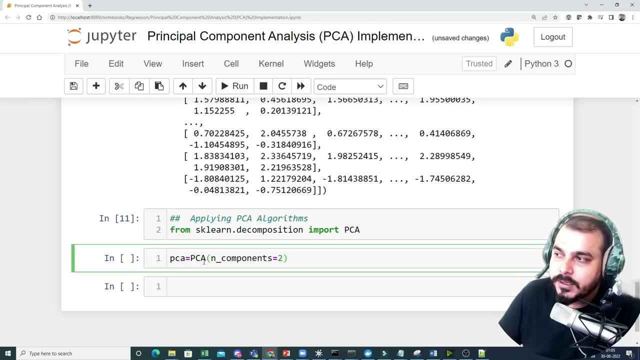 I want to extract two features out of it, which captures maximum variance. So all I have to do is that just go ahead and write this N underscore component as 2.. Okay, So once I probably do this and probably execute it, then all I have to do is that just write PCAfit underscore transform on my data. 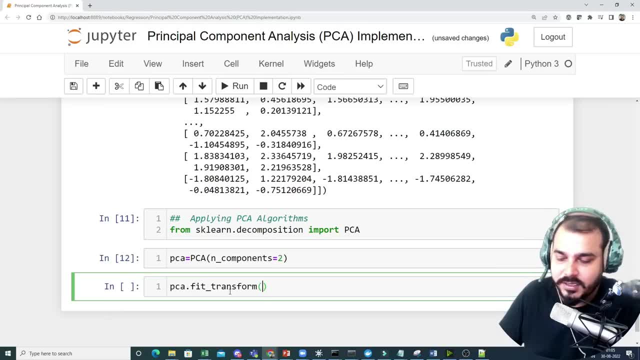 Okay, That data specifically is the entire scale data. I'm just going to give my scale data over here. Okay, And probably once I transform this particular data and if I write this, is my data underscore PCA. Now, here you can see that once I execute this code, what will happen is that my data underscore PCA will just have two columns now. 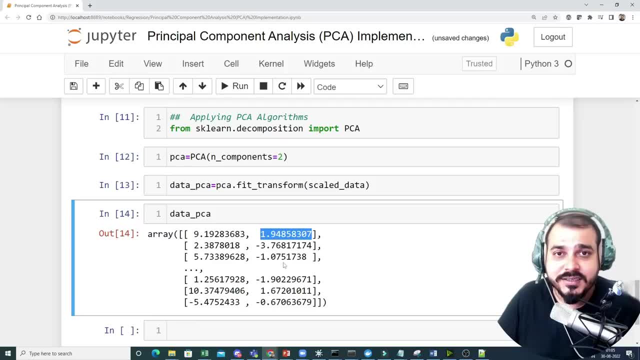 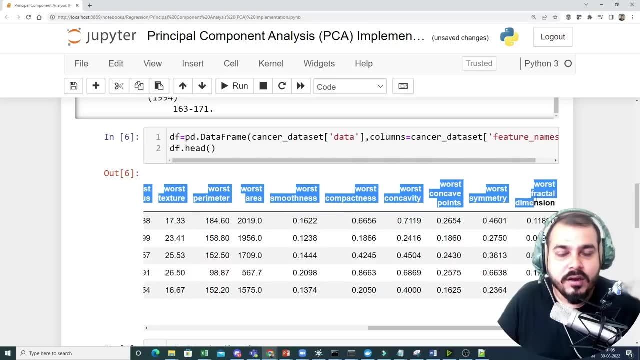 One column and two column Why we have basically converted this into two columns so that we will be able to visualize it. That basically proves it. It means, out of all these columns that we specifically had Right Now, what has happened is that after applying PCA, you know, is that transform the entire data into two columns. 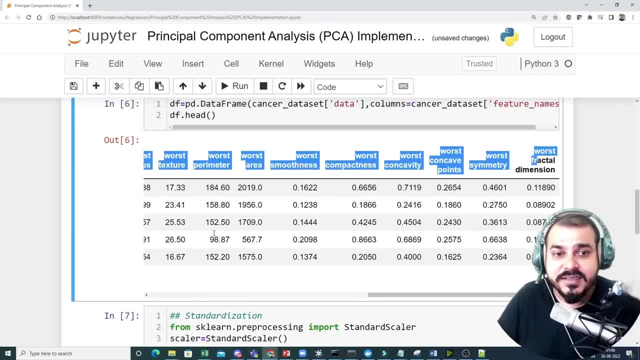 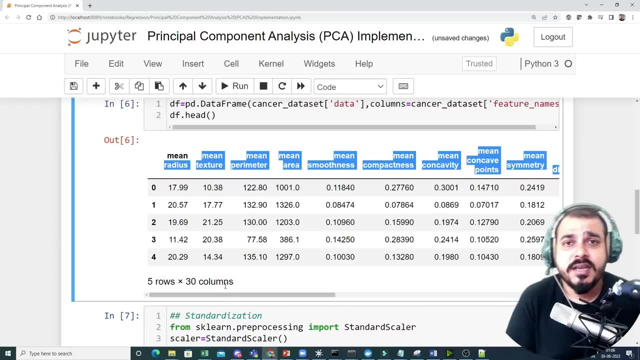 Right. So two feature columns. we are able to get it and it is converted in such a way that maximum variance is basically getting captured. And again for that you have eigen decomposition concepts which we have well discussed in the theory part. 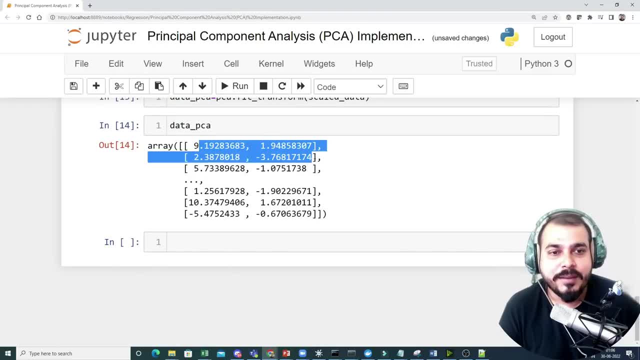 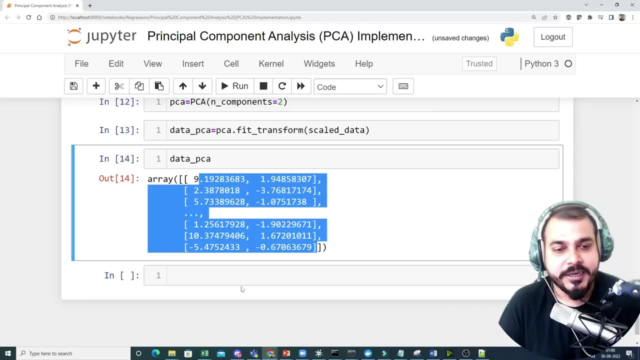 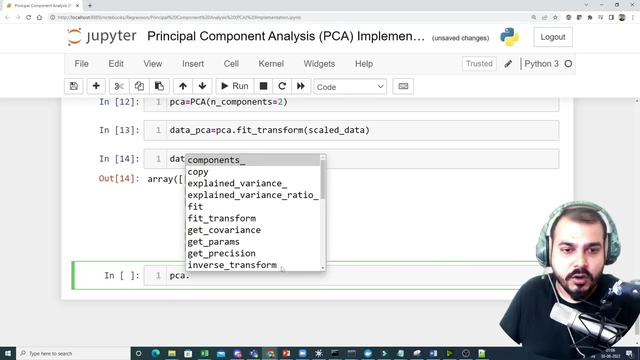 Okay, So now here you'll be able to see that we are able to capture this. two features- Okay, We have two features out of that, entire two, And this process is basically called that dimensionality reduction. Okay, Now, if I probably go ahead and write PCA dot. 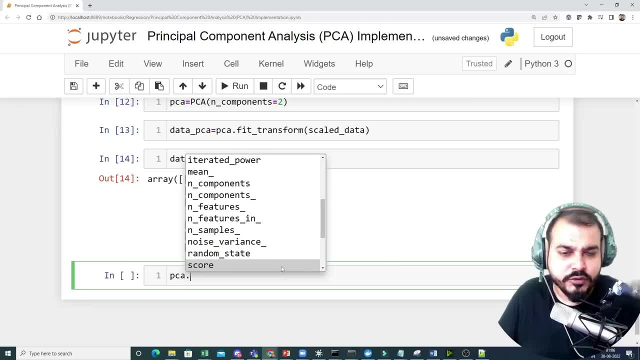 Let's see. there is one more important function I just need to show you, to you, Let me just have a look. Explain variance Right. So once I execute this here, you'll be able to see. this is the explain variance off. 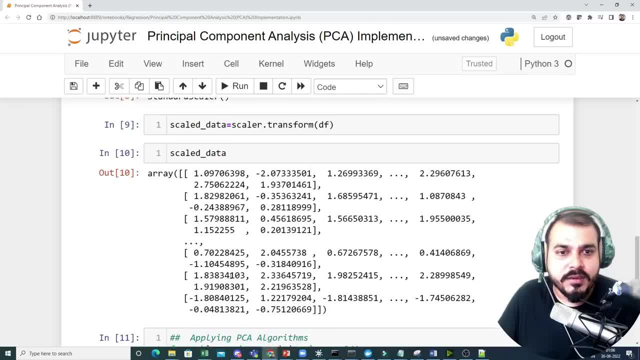 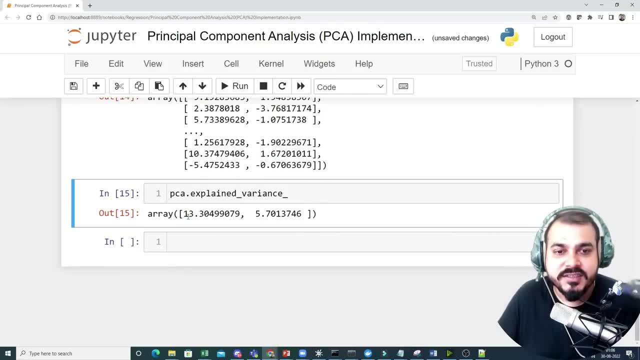 Feature one and feature two. you know, and probably if I, if I don't exactly use an underscore- component is equal to two. So here, why to explain variance? It is saying that because from this two feature, this much variance is being able to get captured. 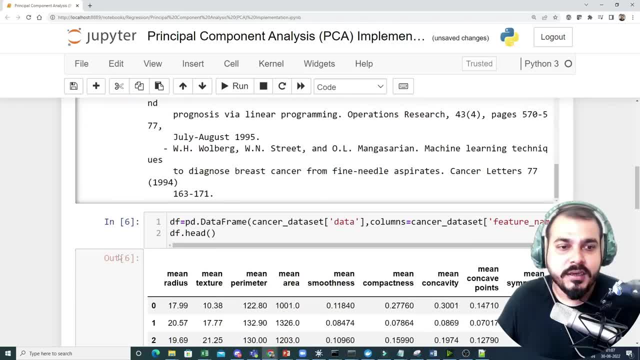 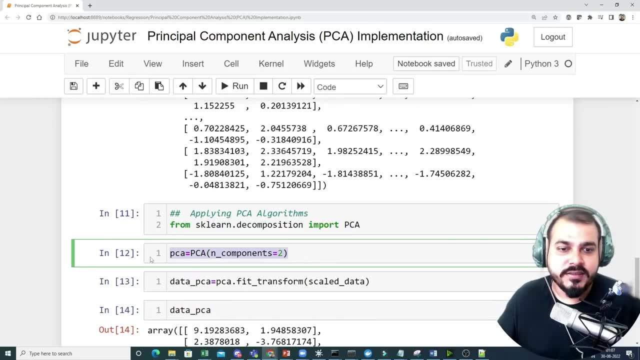 Right. And now here, if you probably know, if I probably take this up and apply the PCA without giving an underscore components, Right? So let's say, if I probably just give over here And I don't give my X underscore components, 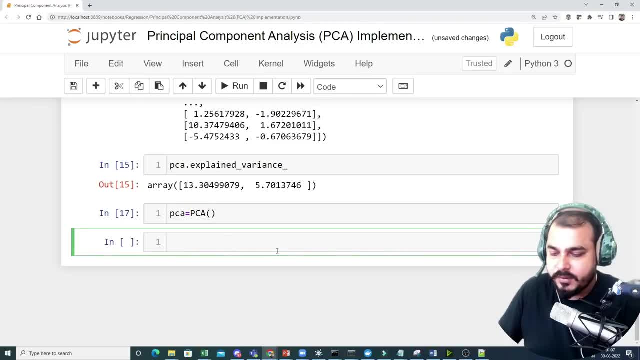 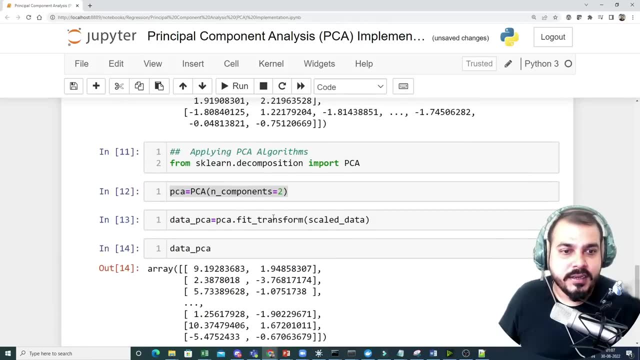 Right, Oops, Let me just write. Okay, And probably then, if I write PCA, dot fit underscore, transform on my data and that data- let's say a scale data- Then what I'm actually going to do, it is just going to create that many number of components. 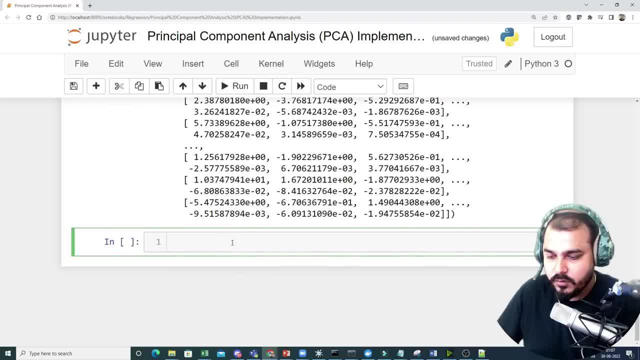 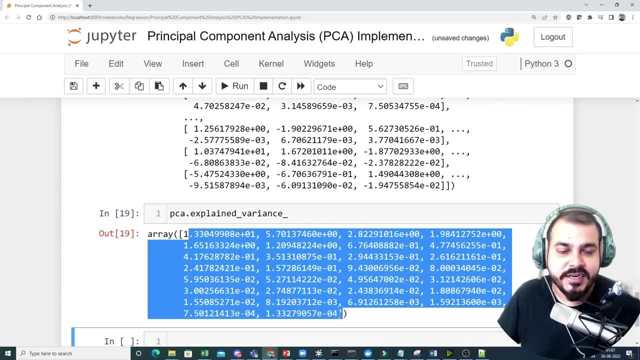 How many number of features were there Right Now. if I probably go and search for PCA, dot explained variance. So here you'll be able to see, with respect to every feature, How much variance is basically getting captured Right, And probably, if I try to add this up, we will be getting some value that is near 200. 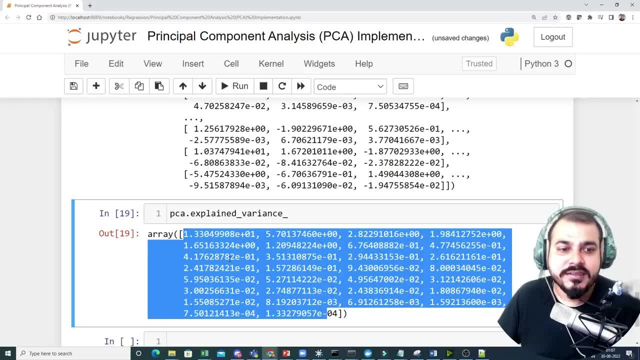 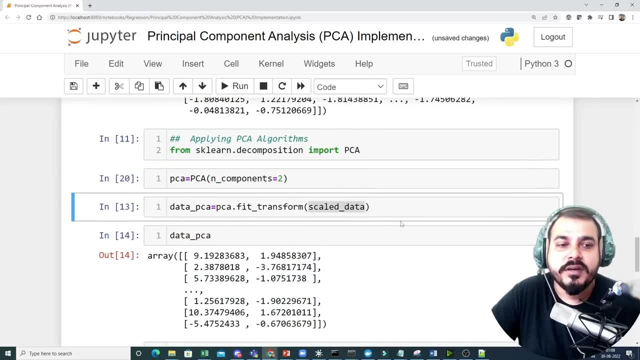 Okay, So here you can clearly see this many number of features, So that many number of explained variance are there. Now you know that what we have done is that we have basically applied and risk component is equal to two, And once I do this, I'm getting two features as my extracted. 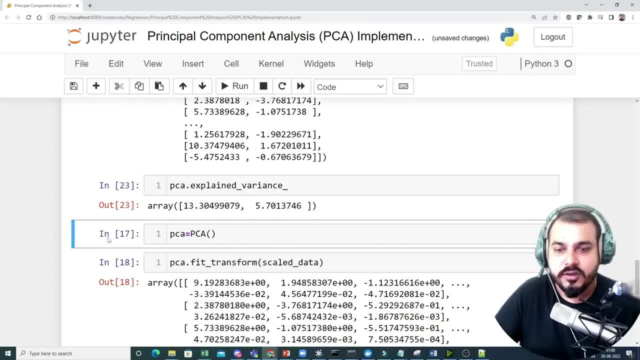 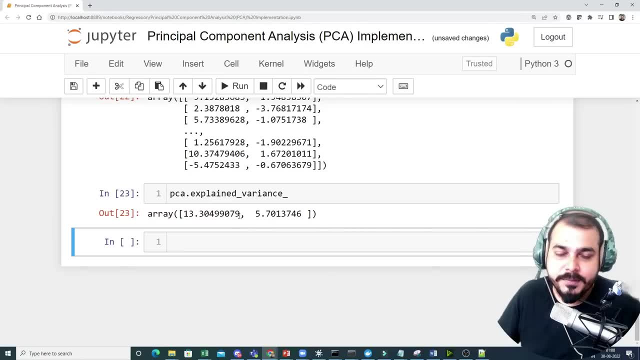 And if I probably see my explained variance, this is how much it is getting captured. Okay, So I'm just going to remove this, since we need to just focus on two, Two variables or two features Right Now. we will try to see that with the help of these two features, will we be able to do something. 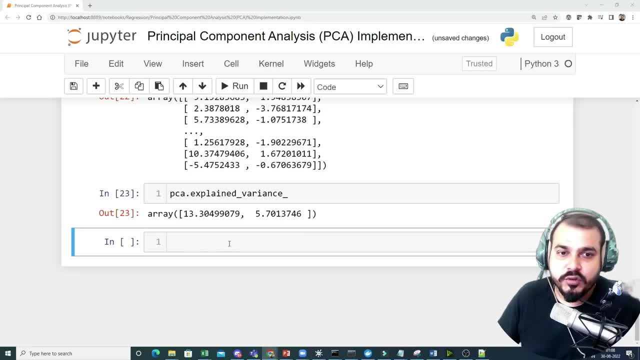 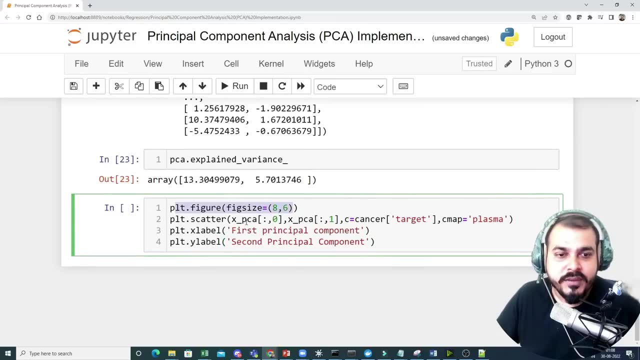 Right, Will we be able to do something? So the best way is that we'll try to see it in the most visualized format. So yeah, I'm copying a code where it is written as plot dot figure And here you can see data underscore: PCA. 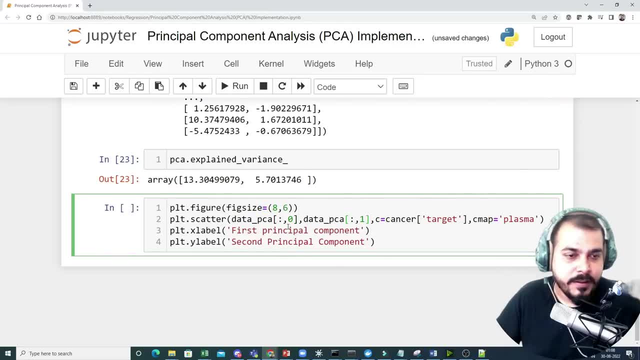 I'm just going to use data underscore PCA over here: Data underscore PCA. So this is for my first feature And this is for my first feature. Sorry, Zeroth feature. Zeroth feature over here And this is my first feature. 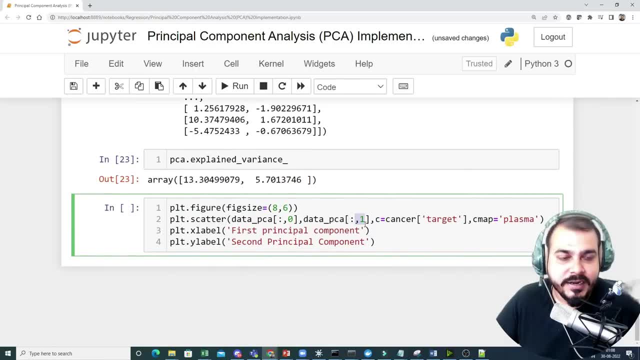 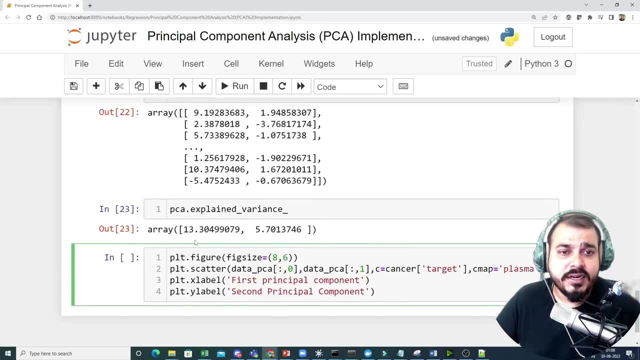 I'm just trying to plot it in the scatter diagram And over here. what I have actually done is that we are going to also take the target column Now, this target column here you'll be able to see that where our target column basically exists in this. 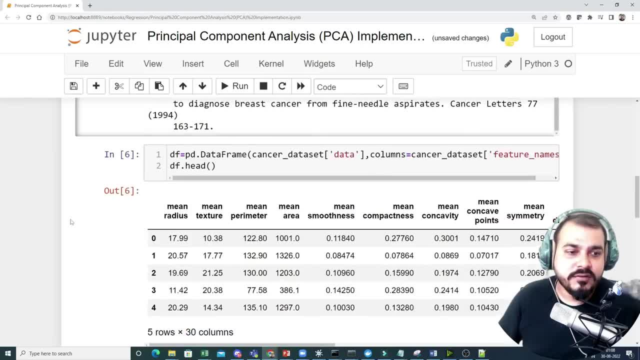 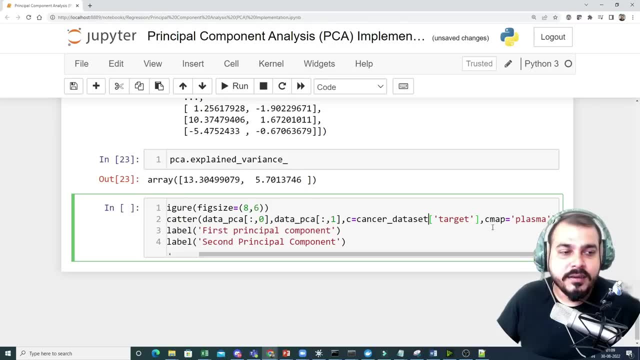 Right, So cancer underscore. data of target. If I probably write, we'll be able to get all the target values over there, And then the type of mapping we are going to use is something called a plasma. My X level will basically be the target. 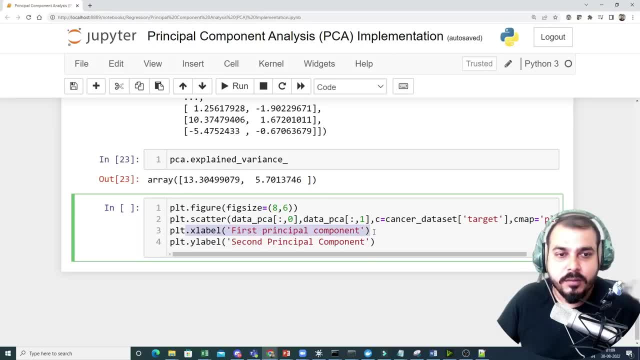 Right, So my X level will basically talk about first principle component and second principle component. Always understand: the first principle component will have maximum variance captured when compared to the second one. Then as we go with respect to the third one again, the variance will get reduced. 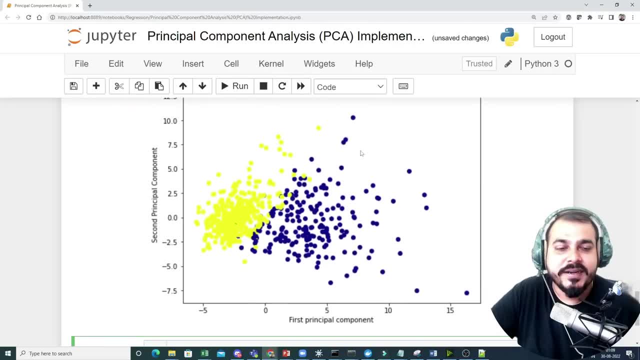 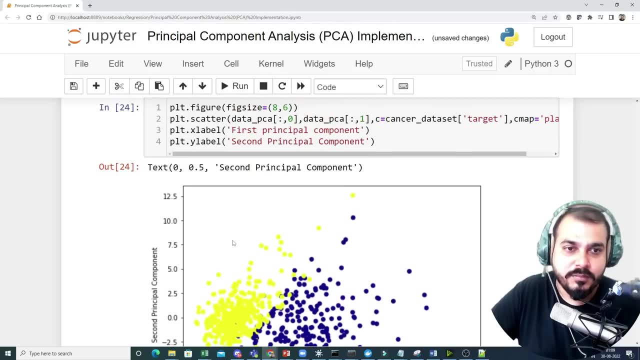 Okay, So once I probably execute it here you can see that how clearly the my data points is visible, And even for this particular problem statement I can probably solve it with the help of any classification problem statement. But here you can definitely see that. 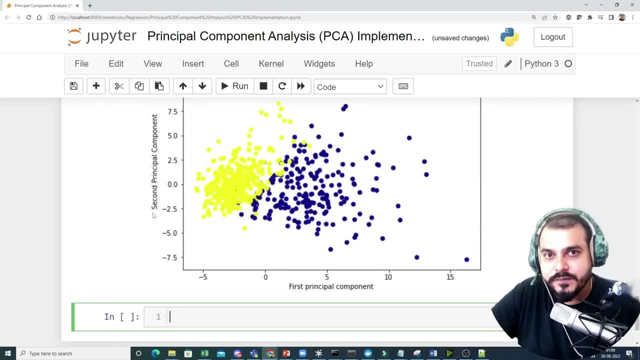 Of all the 11 to 12 features. you have easily converted this into two features And now it was able to capture maximum amount of information. So that is the reason my data points is clearly separable, And this was all about principle component analysis. 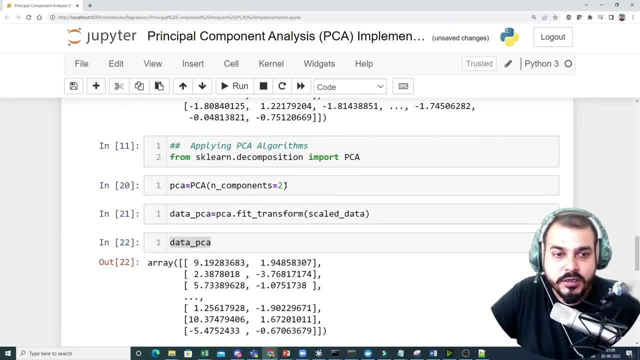 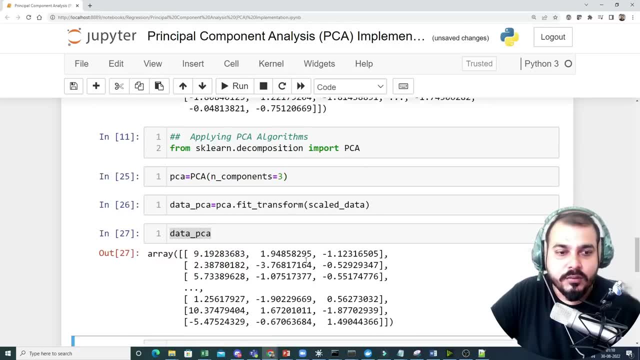 And how can you implement it? Probably, if you wanted three components, you could just need to write three components over here, Right, And let me just show you. That will also give you an idea. Like see, when I wrote n underscore, component is equal to three. I got three features. 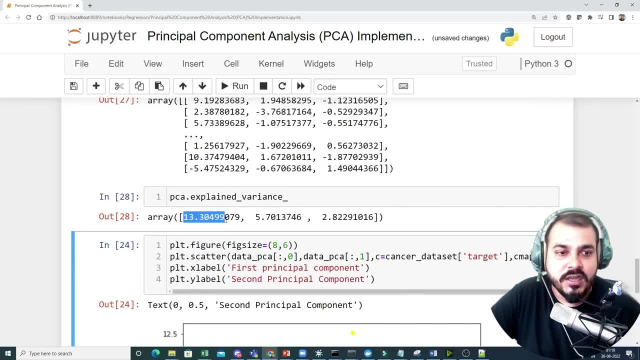 Now, if I probably go and write explained underscore variance, I'll be getting three values: This is PCA one, This is PCA two And this is PCA three: PC one, PC two, PC three. Right, And here you can see that this variance is getting decreased. 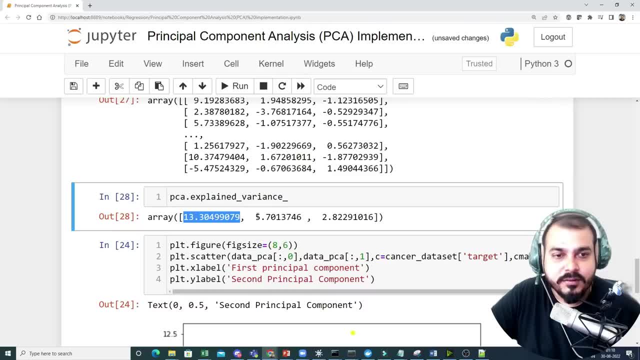 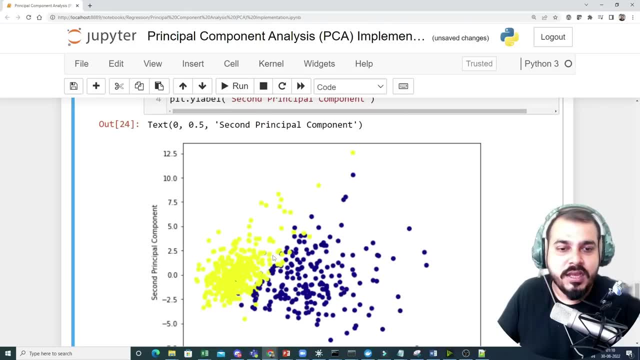 Right. So PC one will be having the maximum number of variance that will be able to capture out of this Right. But now here, just to further displaying purpose, you can also do it for the three dimension. I'll just keep it like this. 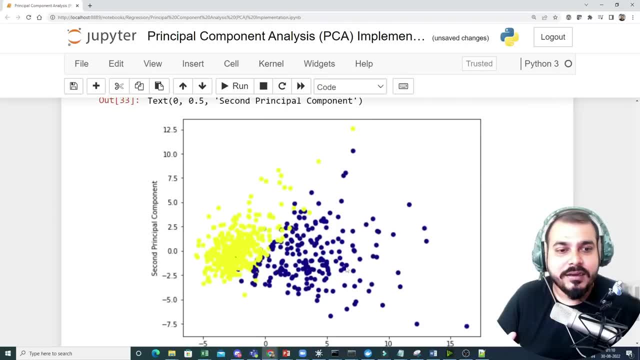 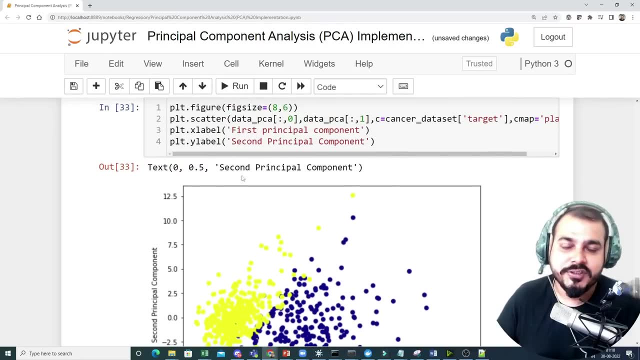 And this is how it basically looks at. Okay, So you can definitely Try out your own examples. You can take up a data set and try to convert it into two features, one feature, three features, as many you actually like, Right.